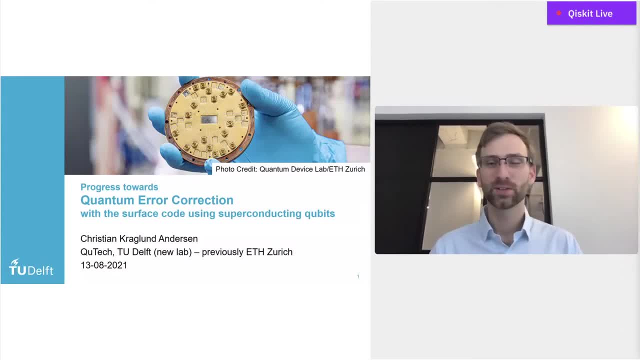 I'm thrilled to roll out the latest episode of the IBM Qiskit Live Quantum Seminar series dedicated to you, the research and academic communities, And today I'm your host, Slatko Minev, from IBM Quantum Research, and I have the pleasure and privilege of hosting Christian. 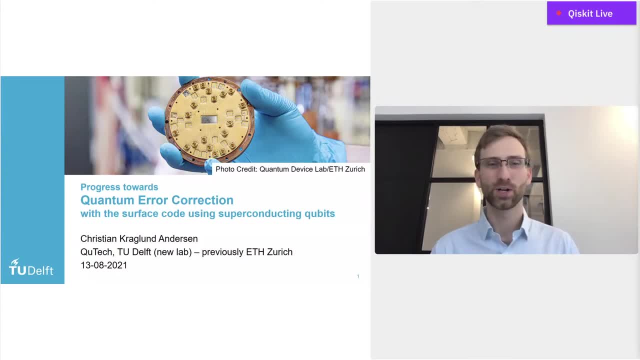 Anderson from QTech, previously ETH, who will talk about progress towards quantum error correction with the surface code. Hello Christian, How are you today? Hello Slatko, Thanks for having me here. I'm very good, thanks. How are you? 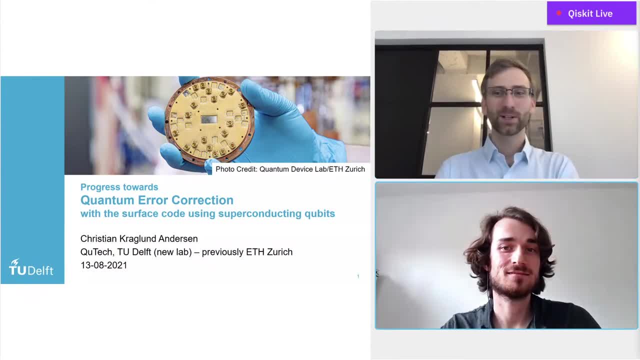 Great, I'm glad you accepted the invitation. Where are you tuning in from today? So I'm sitting in my home in Netherlands, close to Delft, which is a sound close to Den Haag. That's wonderful. It feels like you're. 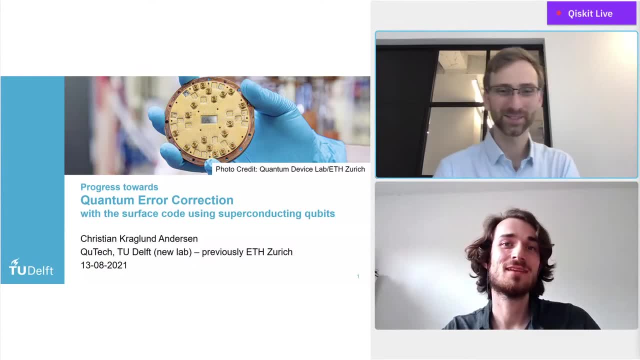 very popular in the Netherlands because we have a very strong presence from that region today. So good to see everybody, All the locals. Yeah, Before we begin, Christian, allow me to give a little bit of background. So Christian did his PhD at Aarhus University and finished in 2016 under Klaus Molmar. 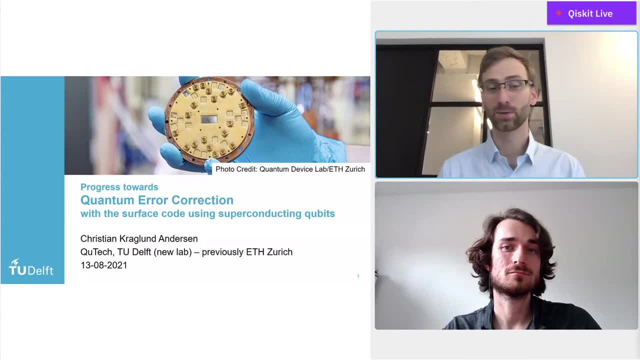 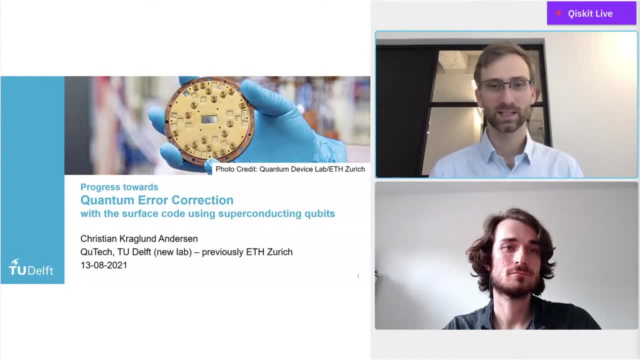 And from March this year we're thrilled to congratulate Christian on starting a new lab at Q-TEC Delft as an assistant professor. And, Christian, I think, with that, the stage is yours And folks feel free to pose questions as we go through this in the chat. 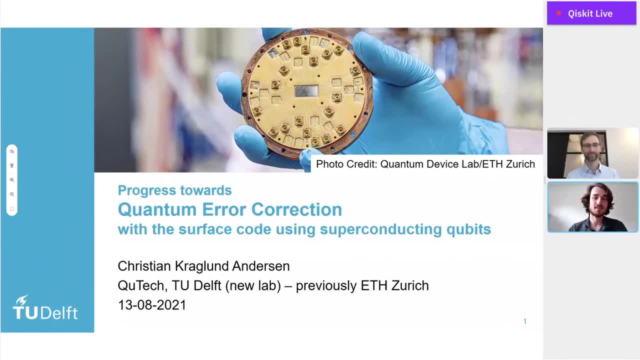 Great. Thank you for the kind introduction, Slackfor. So I will go on and tell you a bit about quantum error correction and the progress that has been made in the field over the the last couple of years towards building real devices of superconducting qubits that can really 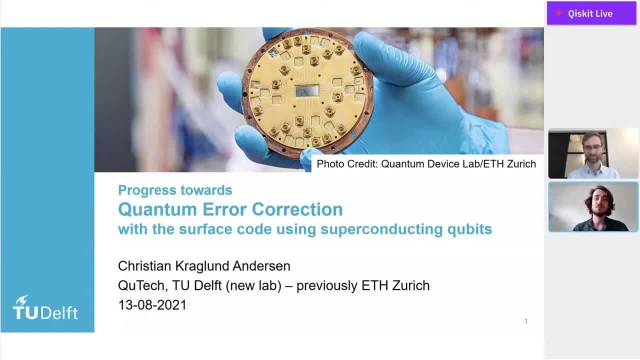 implement quantum error correction within what is known as the service code. When I say real devices, I really mean real devices, as you can see on the title slide here. So what I'm holding in my hand here on the title slide is really a quantum device that we use to make a small demonstration of the 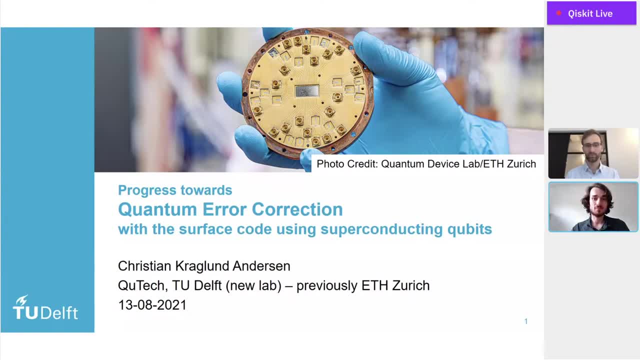 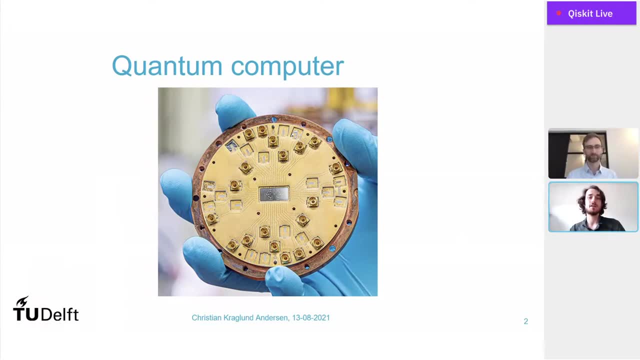 service code that I represent. So maybe let's just zoom in a bit on this and what I'm actually holding here. So this is sort of a very small example of what a quantum computer looks like today. This is a device that has seven qubits that sits here in the center and then around it you 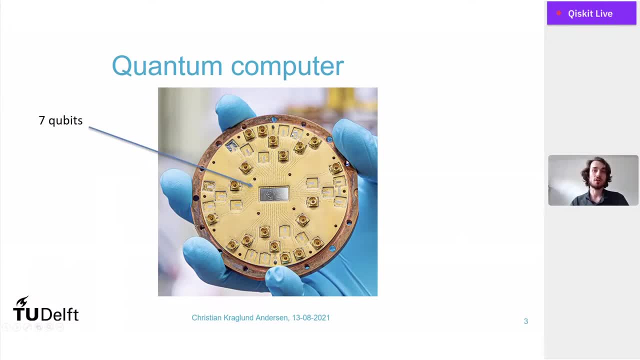 see all these cables and connections going to the qubits. What we can do is we can make sort of a quantum circuit that we can write in Qiskit or whatever favorite language you have, and this circuit is then sent down to our quantum device and that way we can run our quantum. 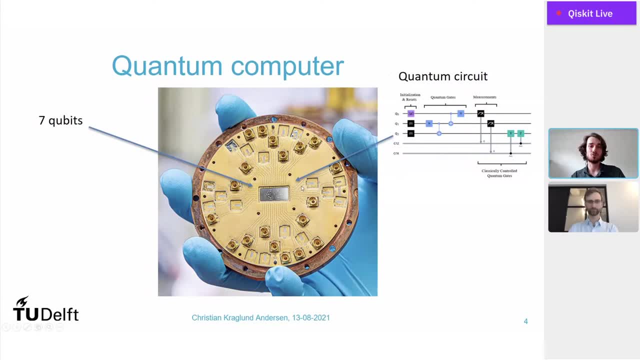 but what happens is that if we do a gate here on our qubits and the thing that can happen is that when that gate is operated it can make an error. The error here you can really think of as a as a small problem, But the gate just didn't do what we wanted to, so we get an error. And now the question about 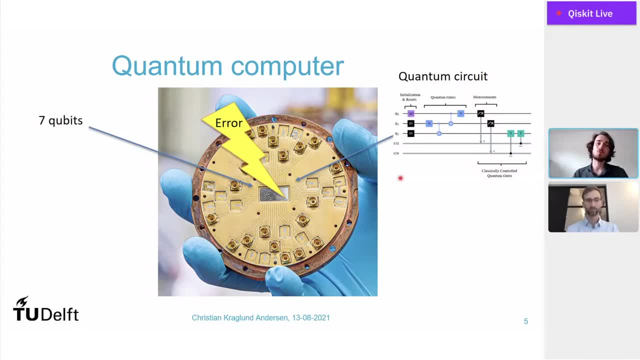 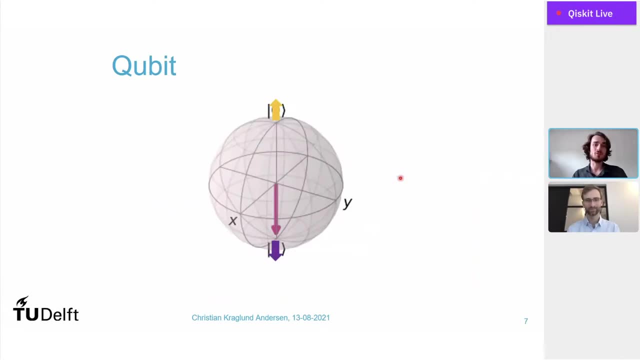 quantum error operation is that how can we take these errors and then correct them such that they are not there? So this is the goal: To make this sort of a bit more complete. let's just take the sort of very basic example of a qubit. So we have a qubit, a block sphere, it can be up. 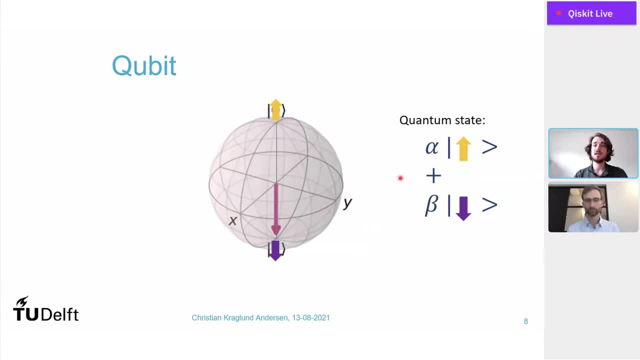 or it can be down, And then we can make a quantum state between these two Which is sort of can make be an arbitrary superposition. So we have some alpha up plus beta down, and this is our qubit state. We take this qubit state and then run a gate on it. What can happen is that there was an error. 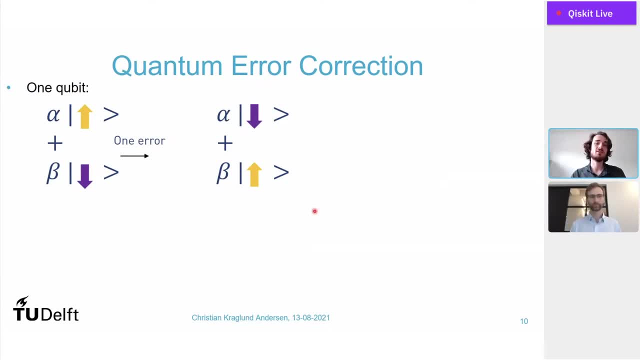 And now, in this sort of very simple school picture, the error here could be that up goes to down and down goes to up, So the error goes from this state here to this. And if that happens while we are doing a quantum algorithm, that's pretty bad, because then all the rest of the algorithm does the wrong. 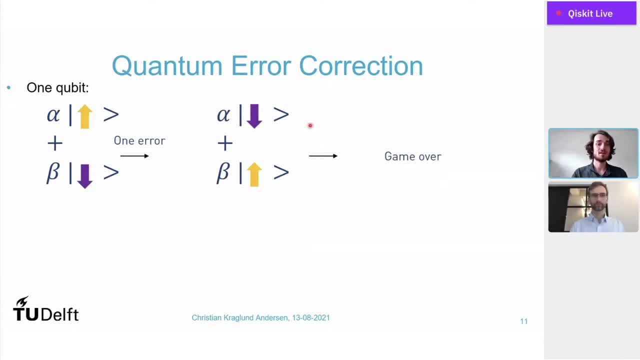 thing. So it's really game over from this point. Instead, what we want to do is we want to play sort of a game called redundancy. So instead of just having one qubit, we can take more qubits. Here's an example: with three, And instead of just having one up the qubit, we can say that okay, our zero. 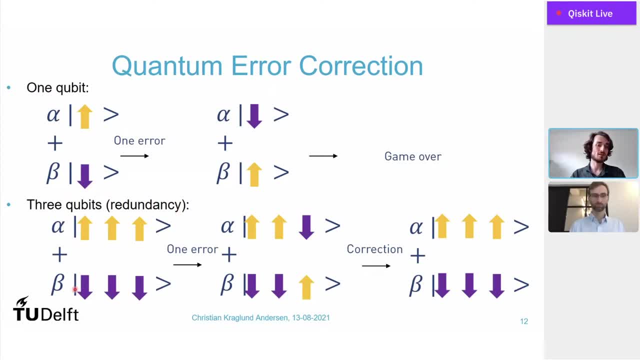 state is really three qubits And our one state is three qubits writing down. Since then, our quantum state is then alpha up plus beta down. Now, in the case again that we are trying to do a computation and an error would occur, Then the error would occur only on sort of one of these physical qubits. 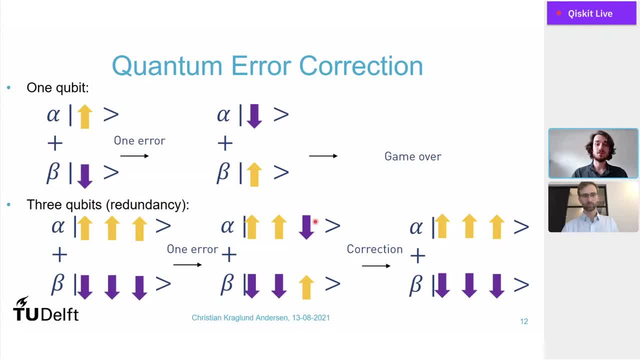 And if that happens, for example here on the third qubit, it's possible to correct it. And now you can say, okay, it's quantum mechanics, so how can you correct it? because you can't actually ask now what are the state of each qubit, because that would collapse the state. But then the trick. 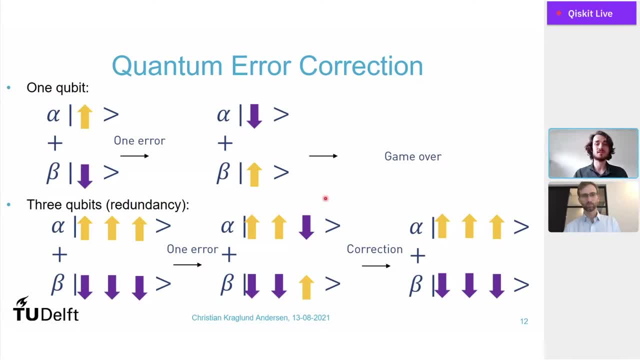 you can do together with redundancy is asking two neighboring qubits: are you in the same state? And in this case it would be yes, In this case we would get a no. When we ask this question, we actually don't collapse the state because you always get the same answer for, let's say, the both. 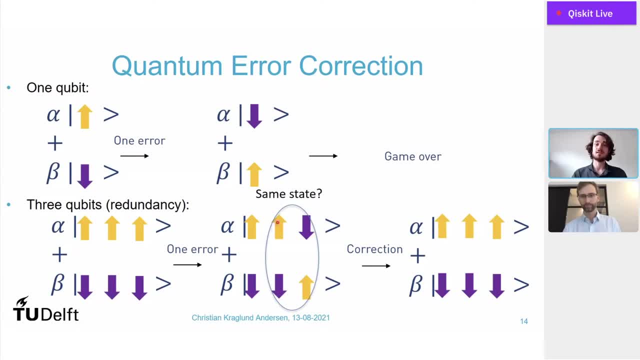 parts of your superposition. So it's a valid answer. that doesn't. it's not forbidden in quantum mechanics And we get a no here. and because we got yes here and a no here, we can infer in this process of affirming we call decoding- that the error was really on the last qubit. So we can. 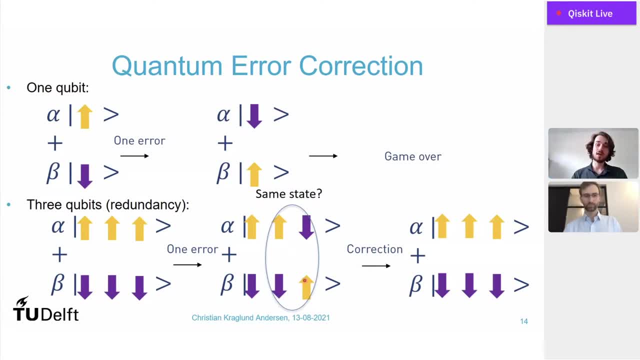 correct this, and we have sort of corrected this physical error such that our logical state here is then what we wanted to get. So this is how, very basically, quantum algorithm works. So we want to do this, and maybe I should say a bit more why we really want to do it. but maybe 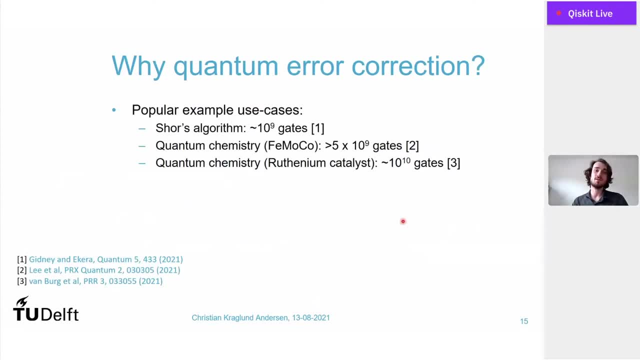 it sounds a bit complicated, but I want to sort of convey the message that it's really needed. Why is that? Because if we look at literature of sort of quantum algorithm that's written down and should provide sort of real life examples where we know that this will be very, very important to do and you just count: how many gates do you need to run? 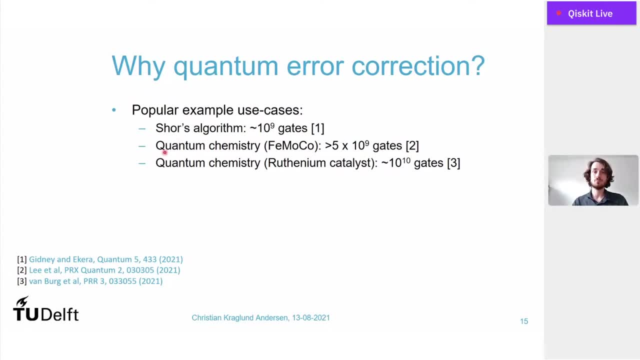 things like Shor's algorithm or things like quantum chemistry for nitrogen sequencation, or we can do some catalysts in quantum chemistry. If you count the number of gates, it's like ten to the nine, five times ten to the nine, even ten to the ten gates. 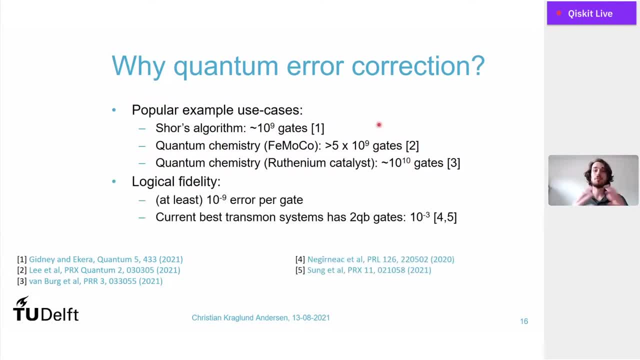 That's really a lot of gates. So if we are just very naive- in reality it's a bit more complicated It's, but really naively for this case, sort of in the very worst case- we at least need errors that are at ten to the nine, meaning the probability that we have an error every time we do a gate. 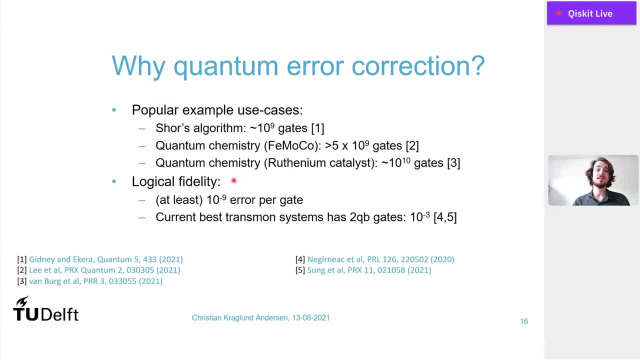 should be smaller than ten to the nine and reality maybe even ten to the ten, ten to the eleven, Let's just say ten to the nine, which is really really much smaller than sort of the current best two qubit gates for superconducting qubits, specifically transparent qubits, which are sort of getting close to this. 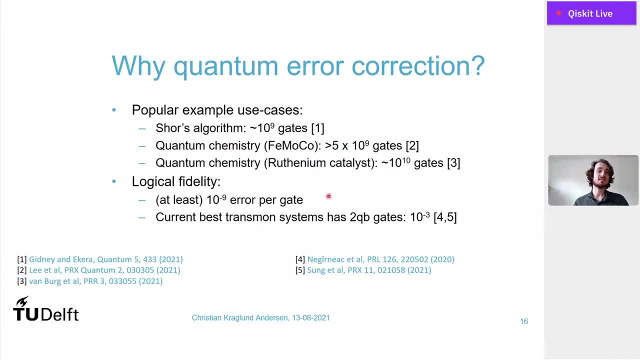 ten to the minus three, So we need to be essentially six orders of magnitude- or even more- better than we are now in terms of running our gates, And the only way that we currently know how to get there on paper is using this trick of quantum algorithm. 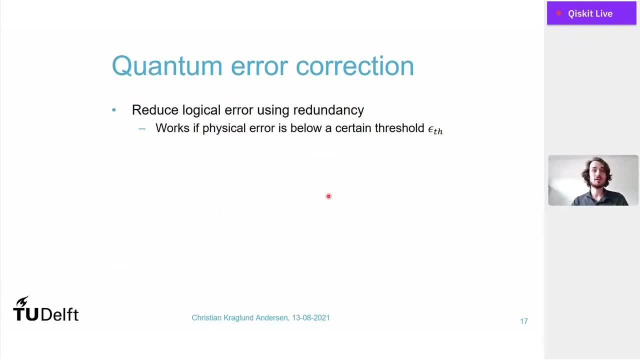 Be slightly more formal about it. what we talk about is we talk about what is called a threshold. So when we play this game of redundancy, it really only works if the each individual gate that we do on the physical qubits are already somewhat good, That's somewhat good threshold. We call that the operation threshold And then 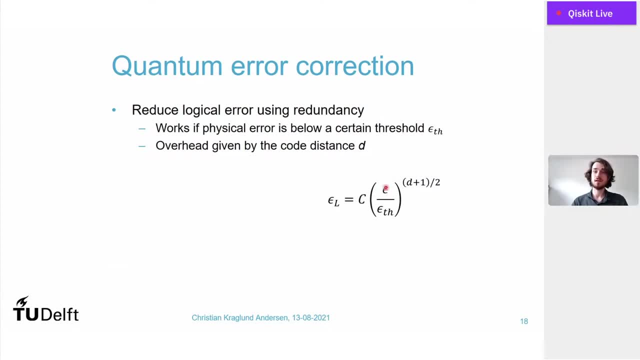 once that is given and we have an error for gate epsilon and we have this threshold error epsilon and we can see if we make a quote by a certain distance. I will come back to this, but that's basically just sort of set by how big is the code And you get this exponential relation between then. 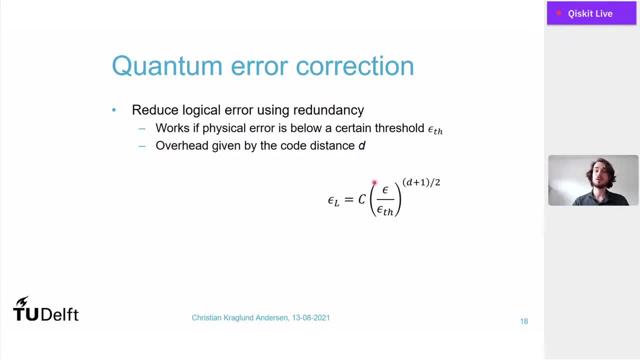 what is your logical error, the thing you do in the end, compared to your physical error, Such that if you can now just increase d, which translates into making more physical qubits, you can make this epsilon m arbitrarily simple, Be slightly more concrete what this t is. If you imagine again, 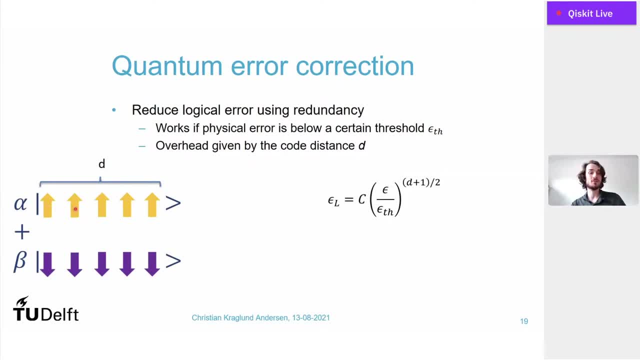 this very simple code that I showed you before, that we just put many qubits in the upstate. Here it would really just be: how many qubits did you put in the upstate? Now? you can then ask: okay, if you want to go to this tens of the time, how big do we need? So let's do a simple example and let's 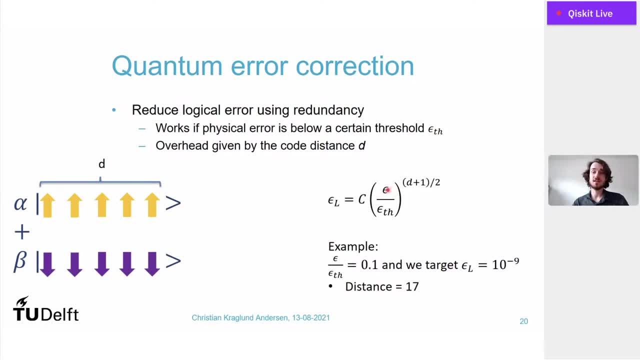 assume that the error here On our physical gate, this sort of factor of 10, smaller threshold, and if we target this 10 to the 9, the distance we need is 17.. So that's sort of a way you can translate this. So that's our quantum operation. So this is really what we 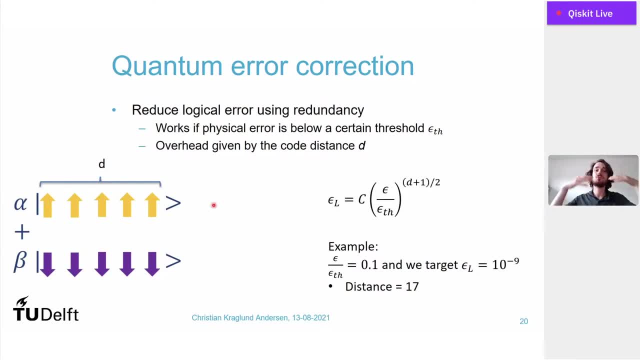 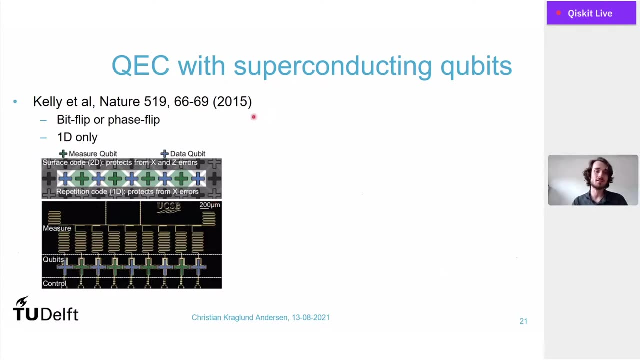 now want to take from this sort of very abstract concepts that I've presented now and make it into something real, physical that we can do with the path. And before I show sort of the very latest results in this, let me go sort of just a bit back in time to sort of a very important milestone. 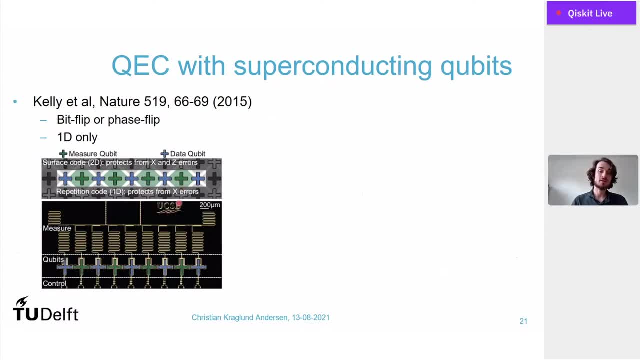 from the group at Santa Barbara that was later translated into the google lab. When they did an example that I just showed before. they did have a 1d string here of qubits that they then encoded into essentially this type of state and they really showed that they can actually do some of basic quantum error. 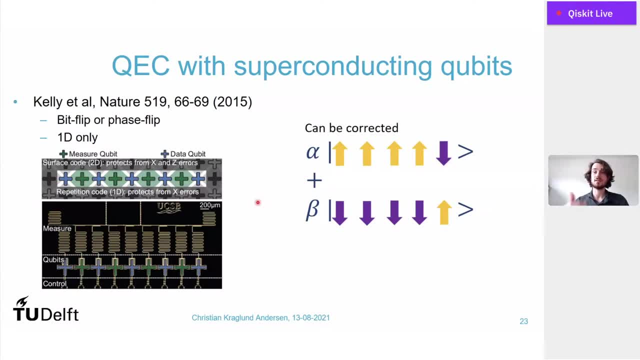 correction operations in this, So they show that they can correct these type of errors. But one of the downsides with this basic example is that I showed here and what they also did in this experiment, which is now five years old, six years old- is that while you can correct this one type, 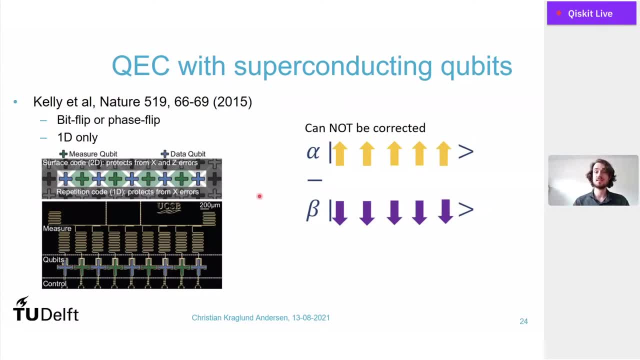 of error by left-foot phase flip. it cannot correct a phase flip at the same time, So you can see that at the same time, meaning that if the sign here changed instead- which can happen- if that's a set error on your physical qubits, then this cannot be corrected, which is a problem. 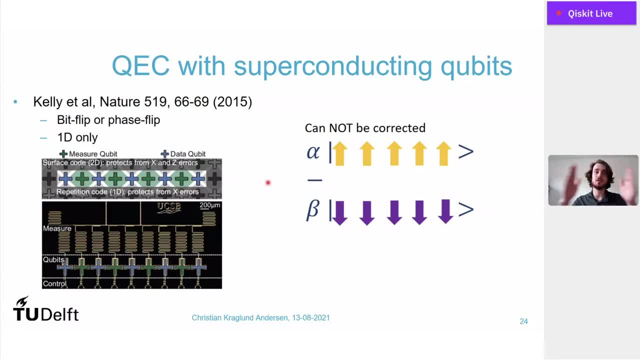 So what you really need is to sort of go beyond this sort of just 1d string qubits to two dimensions, and the sort of idea to do that is called the surface code, where you can make a two-dimensional surface of qubits that can make a code and 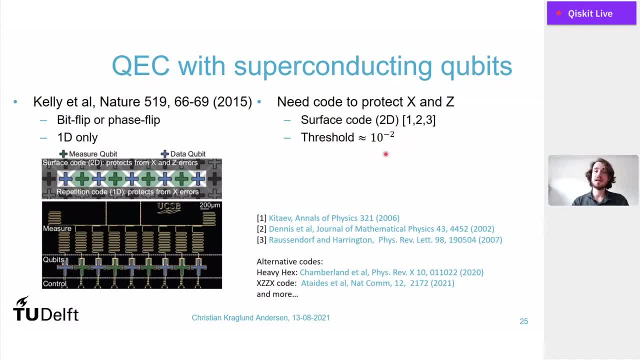 if you crunch all the numbers, it turns out that and again I should say this is sort of when- and this is maybe a good warning for everybody who hear about thresholds not too often- when people talk about thresholds you should always be very skeptical because thresholds depends on many things. it depends on what are the error models people do, what is the code they do. 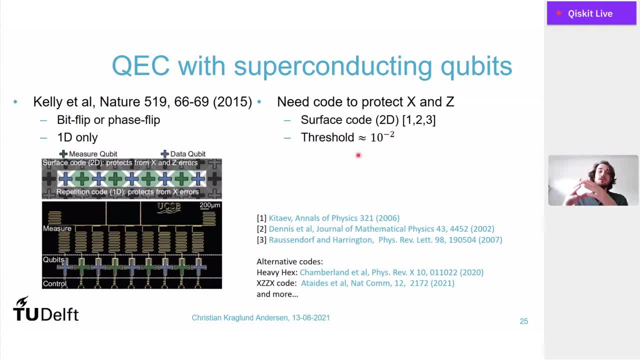 what are the decoders they do? and decoders here, although they translate from the syndromes that they measured, which in this case would be okay, two qubits are in a different state to figuring out where are the real numbers, and all these things goes into the expression. so I'm always 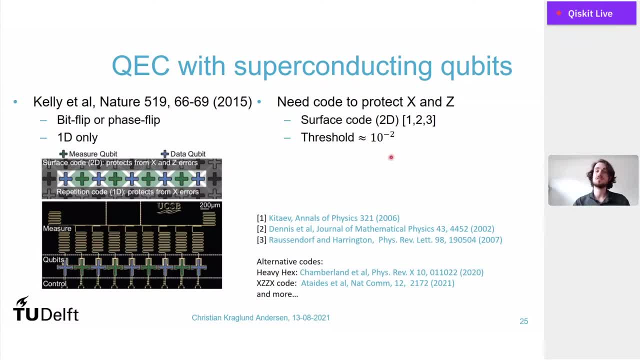 cautious about putting very precise values here because there's many, many less functions. but for the surface code it roughly translates to. the error per gate should be around one percent or maybe half a percent, but in this sort of order. so this is great. we have a code that can correct x errors and set errors. but we want to translate. 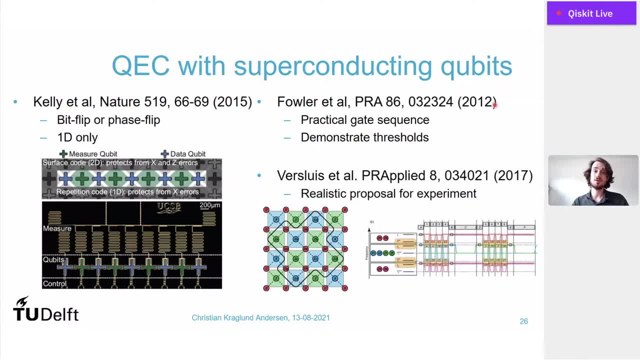 it into really something physical, and the first step along that was, I mean this paper here where from the google group again- where they really showed that, okay, there's a gate sequence that you can run and if you do it, it has a certain threshold and you can do all the operations, which is great, but it needs to be even more realistic. 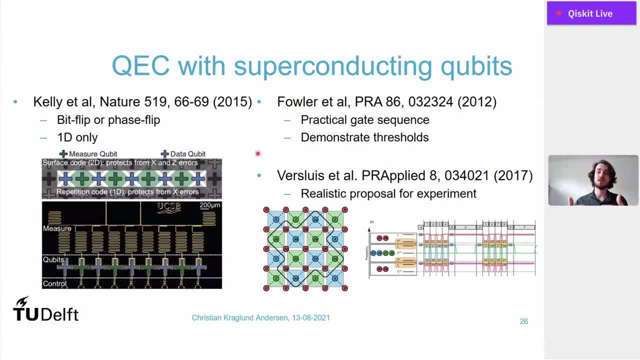 than that, because physical qubits would have frequencies, they would have pulse sequences that are not just here's an x gate. so one of the first steps was then really making that really happen. for starting, this nice paper from the group of very carlo went out, where they really had a very concrete recipe for how to build a service code. 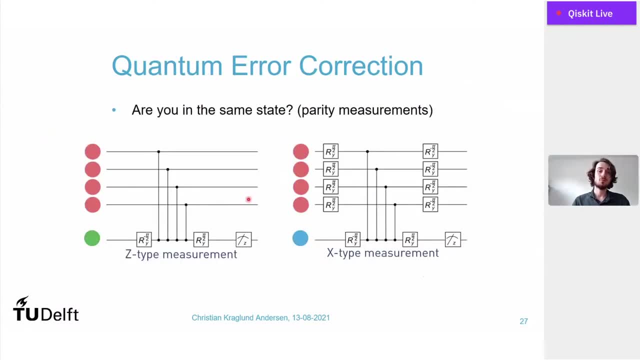 so let's make this a reality. before I go into more details, let me go a bit more about the service code. so, as I mentioned, the idea of the operation codes is really to ask: are qubits in the same state? when you have this one d, you have sort of two neighbors. well, if you have a surface, you really 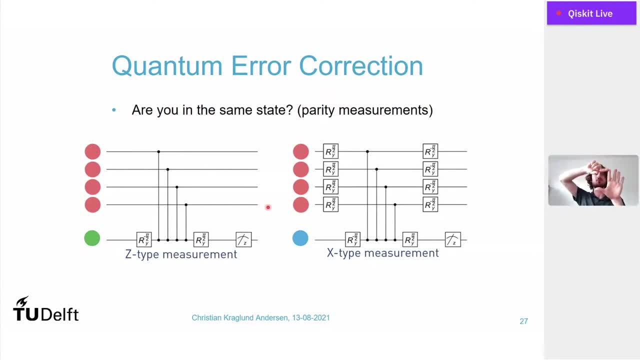 need to ask sort of four qubits, that's, it's sort of a square, and you would want to have them all to be in the same state, and the way you can do that is through this gate scheme here. if you have four qubits sitting here and then you have one extra qubit, which we'll call it select qubits, what you 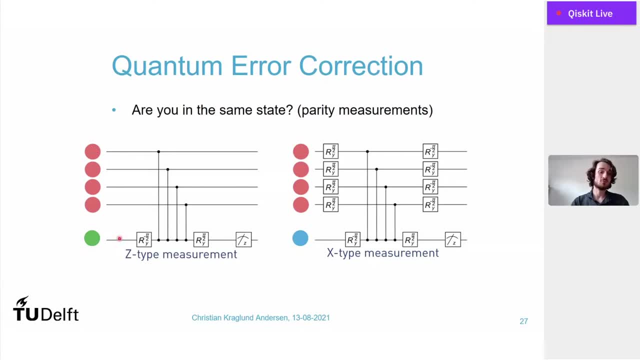 can do is you can run this sequence where you start with the axilla qubit with zero state, then with this pi half policy, put it in an equal superposition so it points along the block equator of the block sequence. then you have this control set gate. what it does is that if the data qubit, the upgrade, 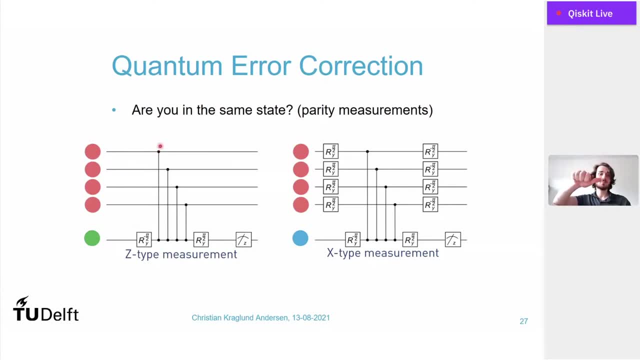 is in the zero state, it will not do anything. but if it's in the one state, you will change the phase of this area and select it. so let's, for example, take this situation where all these qubits are zero state- okay, nothing will happen. and we do a pi half once again now with a different sign, meaning. 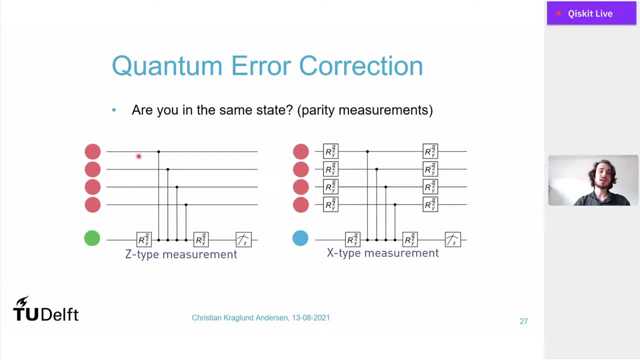 you will just go back to the zero state. similar if they're all in the one state. you will sort of flip the sign of the equator, go to the other side of the block sphere and then go back again and go back, and go back and you would again end up in this state. but if there's an odd number, 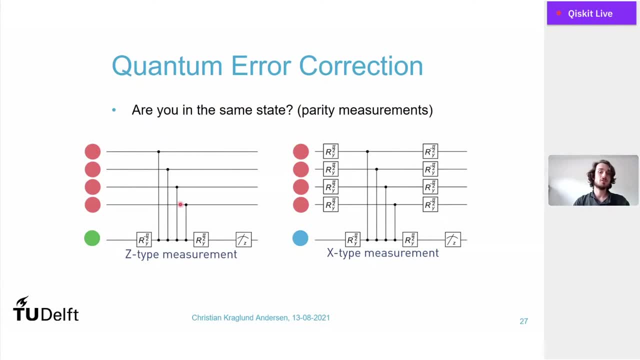 of one states here, and then you will sort of end up at the wrong side of the block sphere. this pi half policy will take you to the excited state and when you mention, you will get one instead of zero. so you know that. okay, some error happened in one of these four qubits and this is sort of in the 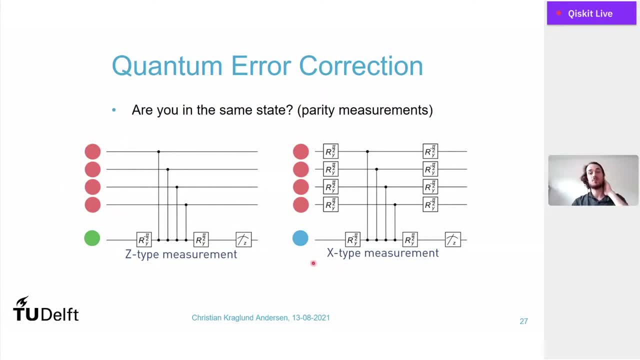 segments. you can do the same in the x basis, which really looks the same, except that we have these uh extra gates sitting here, data qubits, which sort of just rotates from the x basis to the set basis. then we do the exact same thing as well- set time- and then we rotate back again. 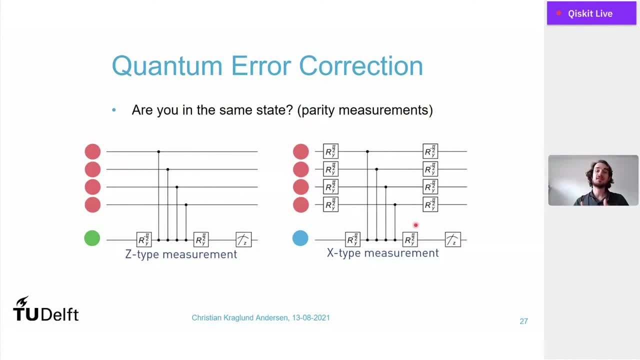 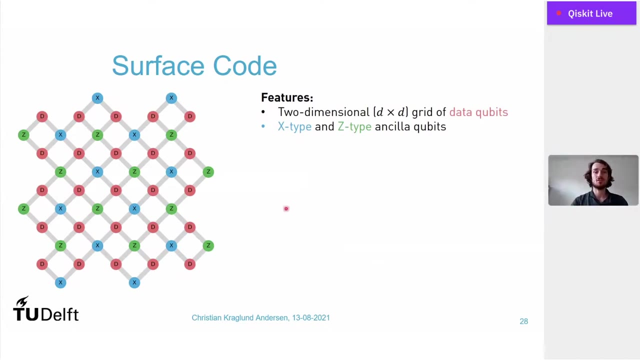 so this is sort of the question. how do i really ask the question: are qubits in the same state when you have this 2d structure? so with that tool at hand we can really start to build the surface code? so we take a tool. i'm using a lattice of data qubits. they have to mention d times d. 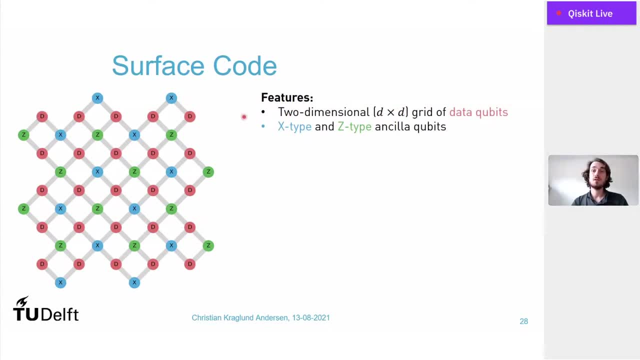 so in this case five times five, and this d here is really the distance of the code that i talked about before. so in 1d it was really just the number of codes, number of qubits, but when you go to 2d the number of qubits is really scaling as distance squared, because we need to be able to take 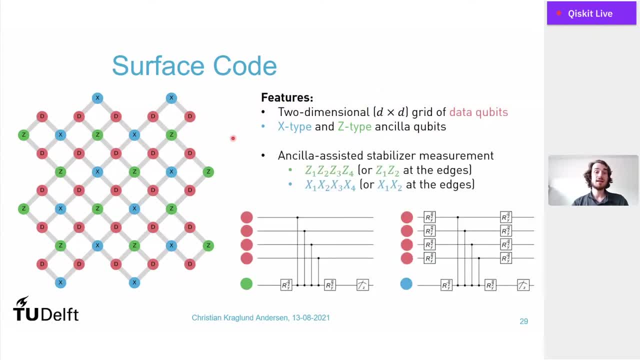 correct two types of numbers. and then we use these sort of green and blue qubits in between the two of the data qubits, as these ancilla qubits, to run these two surveys that i showed you. so this is how the service code is built up on the section. 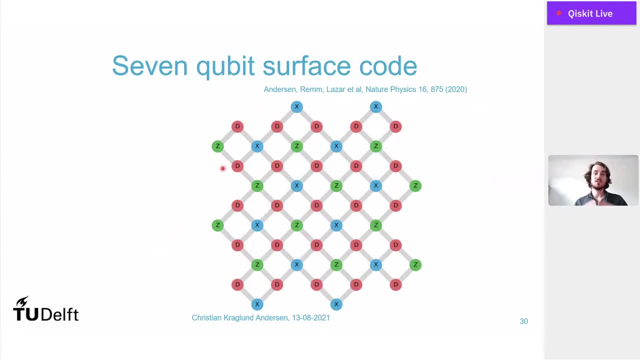 and so now we have sort of conceptually understood how to build a service code. so if you want to demonstrate this in real life, it's always good to start with the simplest example, and okay if it's d times d less. that is the smallest that is sort of meaningful to do is 2 by 2.. let's have a look something like this: 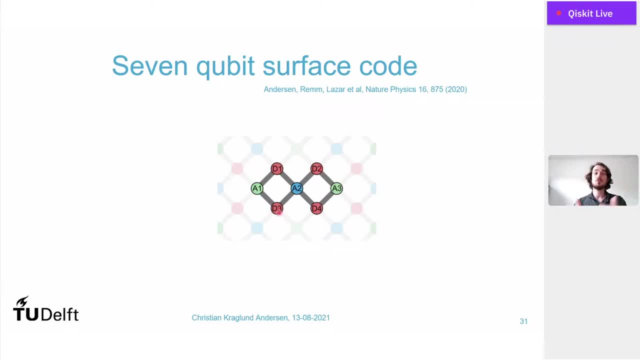 so here we will have four data qubits. is in the data qubits here that we will encode our quantum information? and then we will have three and zeta qubits that we need to then detect whether there was errors once or serve, and we did this in the group. 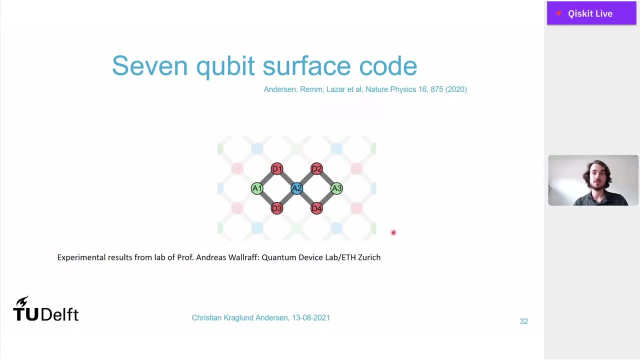 ETH and I will now show you sort of all the results. You can also find more details in our recent publication. Just in case you really want to know the details here, just a few more technical definitions for how we operate the service code. So it's a distance, two code and. 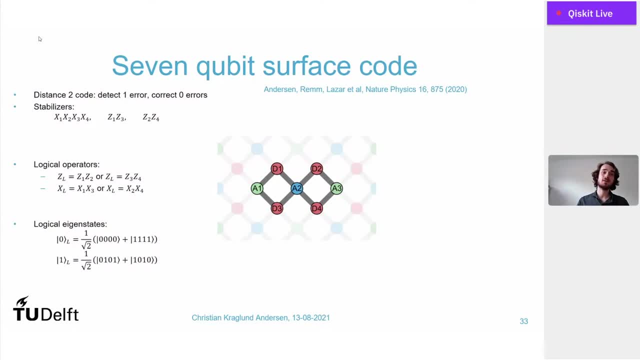 before we sort of move forward. I think one very important aspect to understand about this is that, because it's distance two, what we can do is we can detect if there was an error during our computation, But we can actually not correct it, and that's very easy to understand by again. 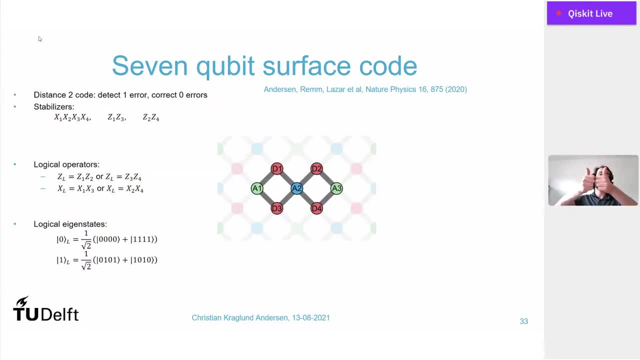 with this example. So if you have a distance two, you would have sort of up or down being what you want, but while up down or down, up would be wrong If I tell you. okay, there was an error. there's no way of knowing whether it's up, down or down. 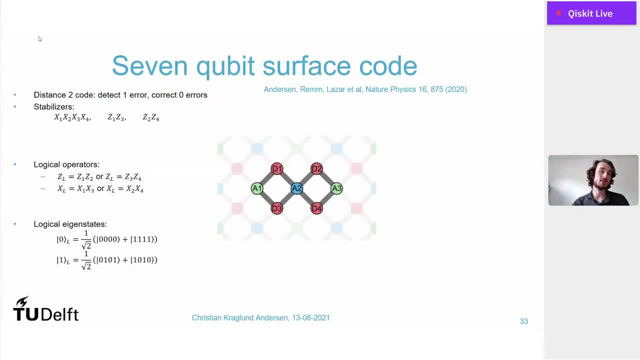 So you can just say, see, okay, there was an error, but you cannot correct it correctly. So this is why it's sort of an error detection code. when you only have a distance two, You really need distance three before you can correct the errors. 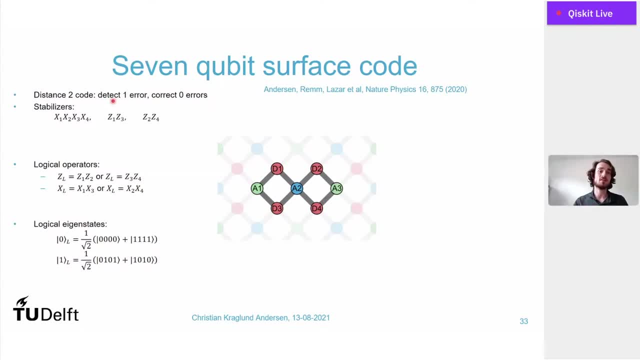 But that's fine. it's still a service code we can detect. was there an error which sort of can be formed in a way that what we really do is we measure these operators here? This is what the circuit has shown you before we're doing. 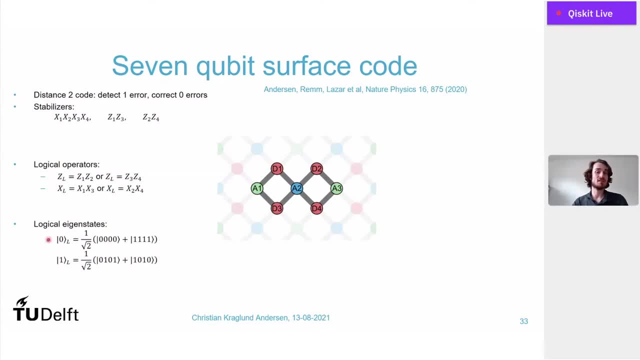 And then the logical states allow. because it's 2D, it looks slightly more complicated than just up up up, But rather it's. the zero state is sort of the equal superposition between all four qubits being zero or one, while the one state is sort of f is zero, one, zero one. 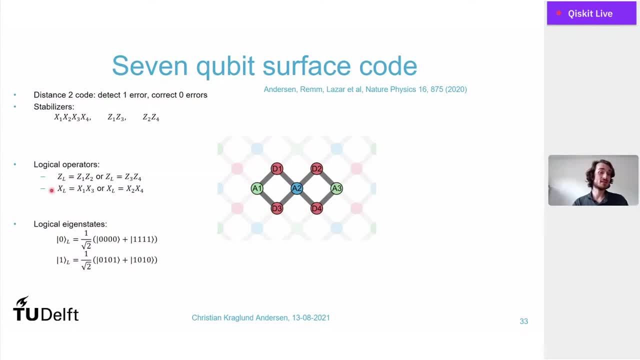 plus one zero, one zero that. These are eigenstates of these logical operators that you see. the logical set operator that you see here And the logical x here is the one that will cause a big flip from zero to one. 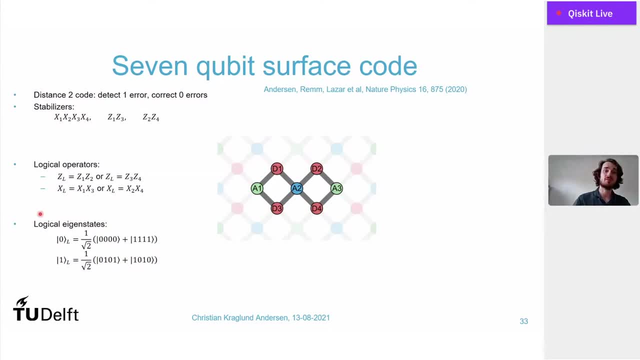 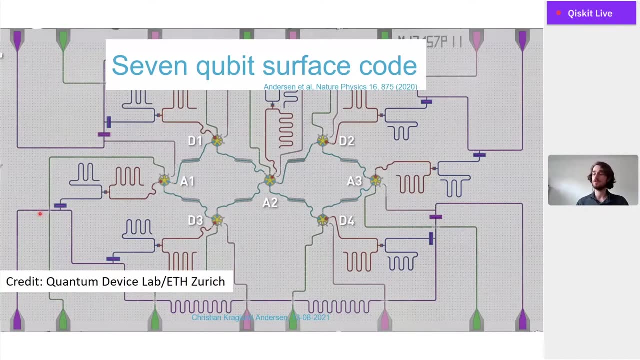 This is how all the ingredients for the service code. So how does this look in real life? I already showed you the device how it looks zoomed out, but if you really zoom in the chip here, you see that this is how the device looks under a. 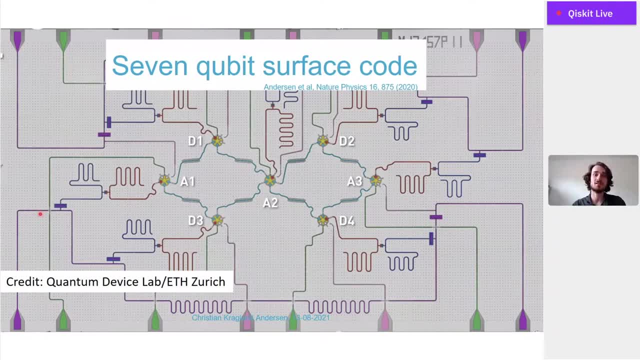 microscope Now here, added with a bit of false colors of course. So it's all in superconductor on a piece of silicon. So in principle it's all the same color, but we chose to color elements such that it's easier to see. And in particular, you see these yellow stars here. These are our. 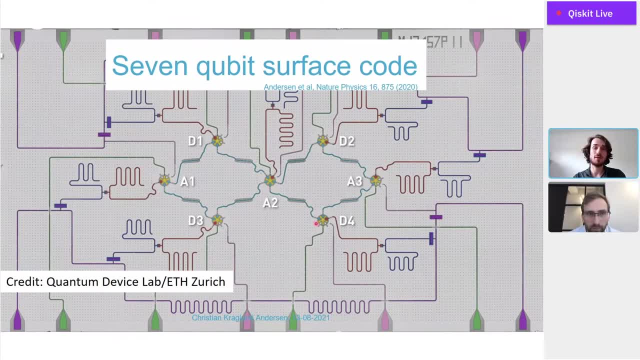 transmon qubits that sit in this pattern that you also see. The qubits are each connected with this line in the pattern here, And this connection here allows us to do two qubit operations between neighboring qubits. That way we can use this, for example: 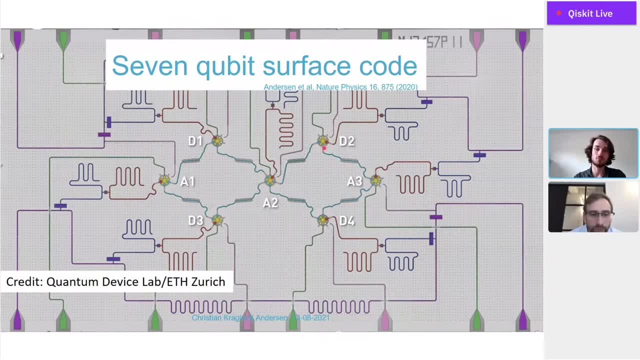 qubit in the center here, So we can do all these four two qubit gates that we're going to use, That we need to detect whether there was an error in one of the four qubits. Now you also see that each qubit here has a green line. 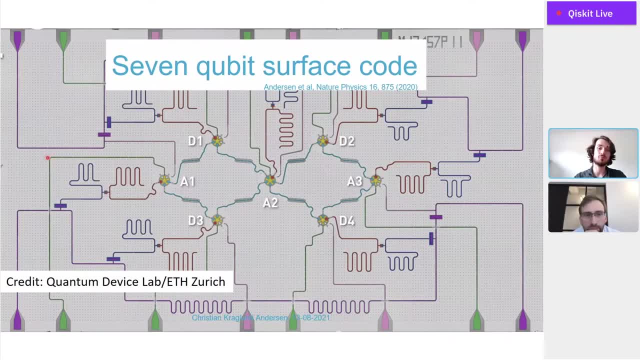 This green line is a flux line. We use that to sort of put a magnetic flux through the squig loop of each qubit to put a specific frequency where we want it to be. And at the same time, when we do our two qubit operations, what we do is we make a very fast 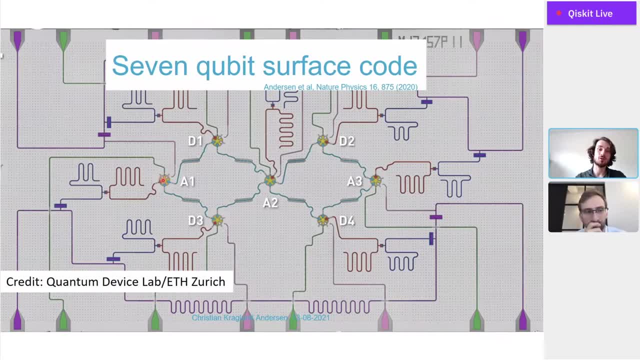 pulse on this flux line, to take, for example, the frequency of qubit one and put it close to the frequency of one of the data units. That way we can enable the interaction, do a two qubit gate and we can go back again. 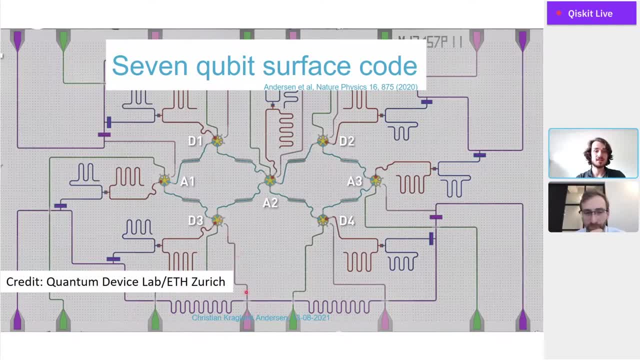 You also see that each qubit has this pink line here. This is a charge line that is used for single qubit gates. And then all the rest, which is this red, blue, purple parts are part of the readouts, which is really important. And then, just to re-emphasize that, what I told you before, 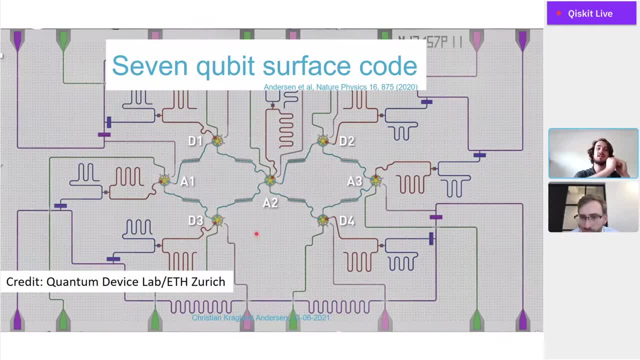 how we operate. inauguration is that we really need to measure the ancilla qubits during the operation to see if there was an error. So it's really important that you have very good readout, And so that's why we have sort of dedicated. 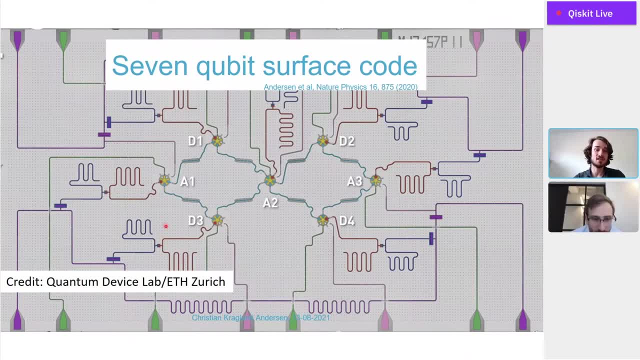 very significant parts of the qubit. So you see that there's a resonator over to each qubit. This is very standard. There's a harmonic oscillator called qubit, And then there's one more resonator here, a new couple to your red resonator. 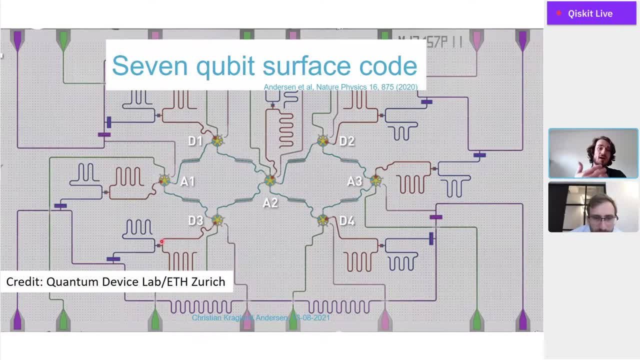 This is a pre-self data that allows us to have very fast readout without sort of accidentally causing additional errors to the qubits. Hello, And if you are sort of well known in the field, you may have seen devices from other groups where they also have pre-self filters, but they don't have pre-self filters for each individual qubit. 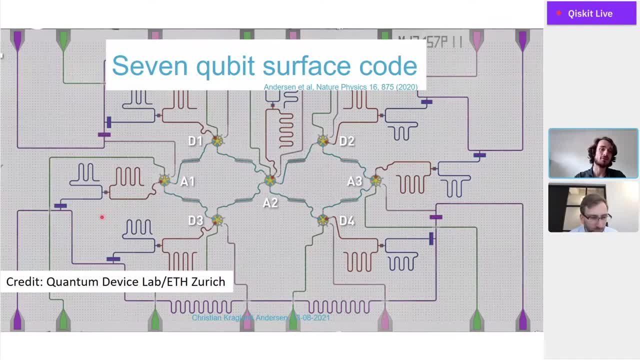 Which you could in principle do if you're just looking to have fast readout. But having these individual pre-self filters, as I've been telling you, actually helps suppressing one extra amount or extra type of error, Yeah, Which is that if you didn't have it, it would be very hard to read out. 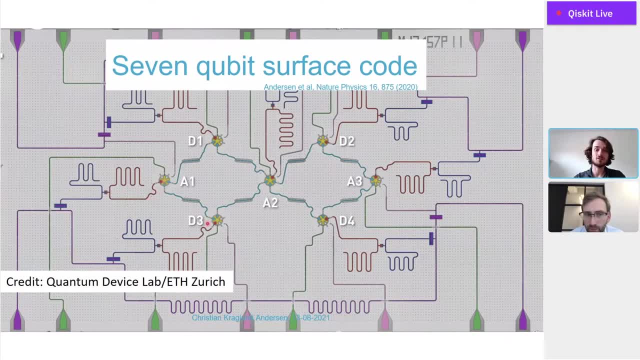 for example, a single qubit one without sort of accidentally also reading out data, qubit three- because they're connected to the same input-output line. But by having these individual pre-self filters we can really suppress this readout crosstalk on our device without doing any. 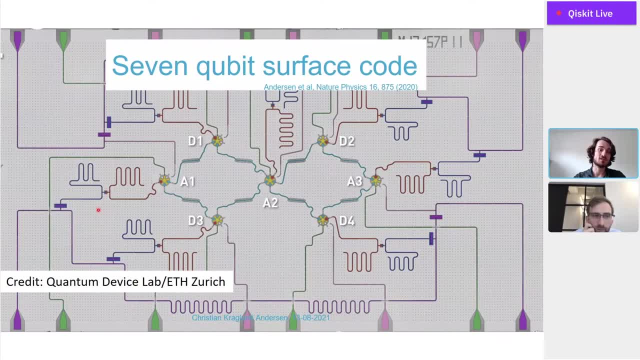 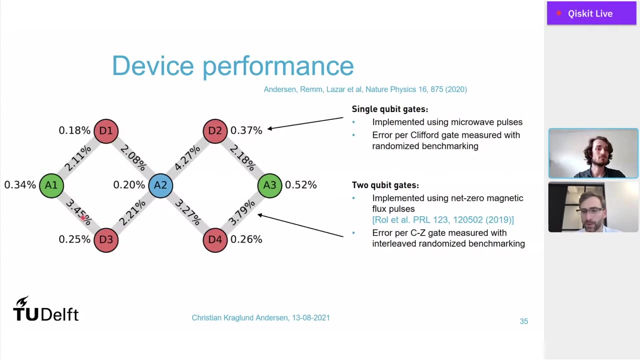 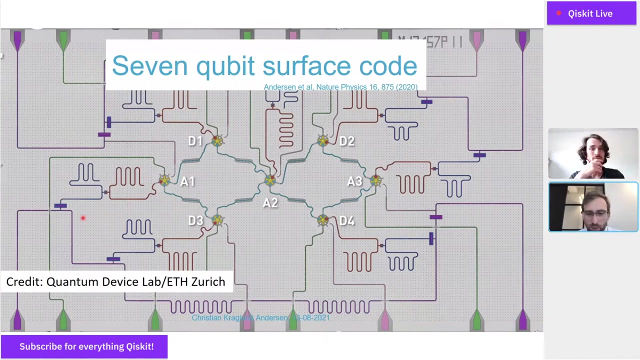 tricks. you know signal processing, And that is really important when you're operating these quantum operation codes. So how well does this device then work? Maybe a couple of questions. Christian, It's a very nice device. And one question to you. 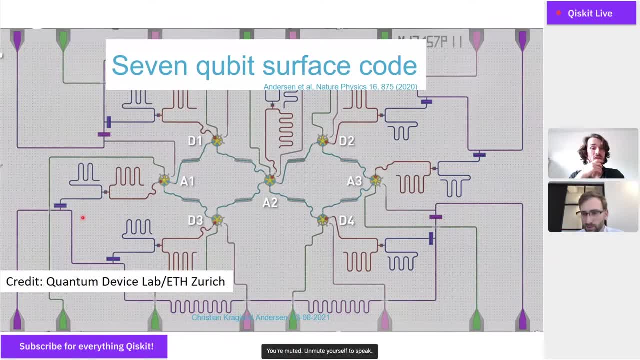 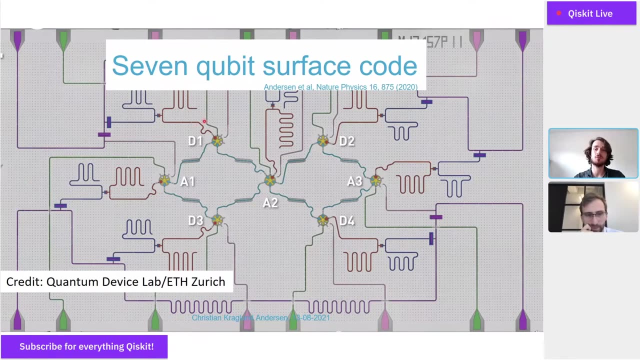 You don't have to multiplex all the readouts if you wanted to, No. so here we can read out any qubit we want, or any combination of qubit we want. This can be programmed by our room temperature electronics, So each qubit is at a different frequency and each readout is a different frequency. 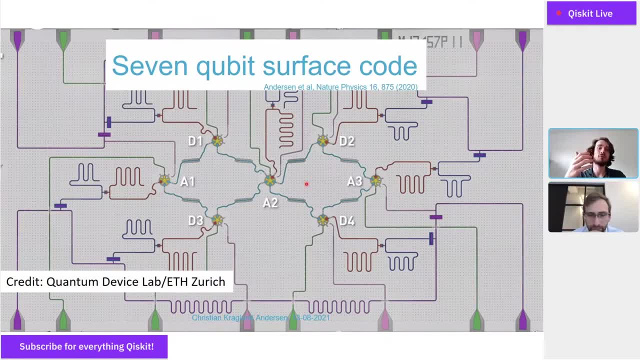 So what we can do is, at any given time where we want to get a readout out, we send in a pulse with frequency components corresponding to the readout frequencies of the qubits we want, And it's really arbitrary, Or you can, for each readout, you can arbitrarily choose which subset of qubits we want to read out. 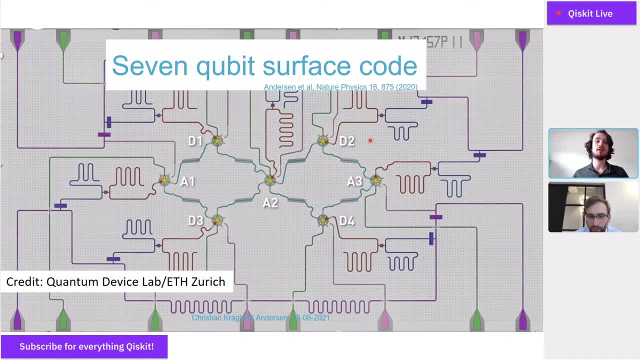 So you can read out all sevens. You can read out just one. It's going to be programmed for you And I know I've asked you this before. but maybe to clarify for other folks on the call, the cutouts at the center of the 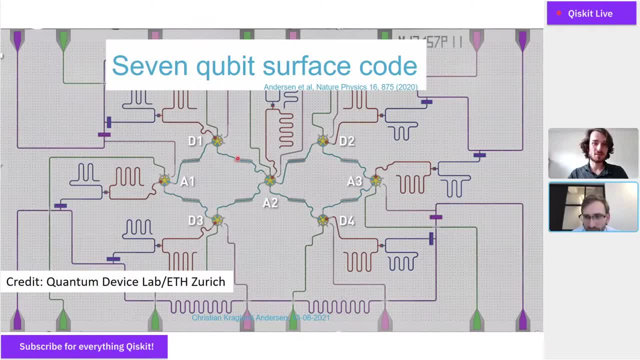 cubics of thecomputer bus couplers in blue. Could you comment on those? Ah, yes, here, yes, Yes, these are. so what you find is that the strength that you couple to here depends somewhat. 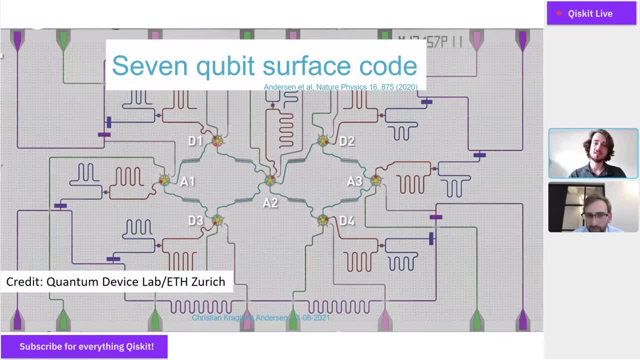 on the impedance of, or it depends on the impedance of this line here. So by making this a little bit wider, you get slightly higher coupling strength, meaning you can do your gates slightly faster. It's not a lot, It's a very small difference. 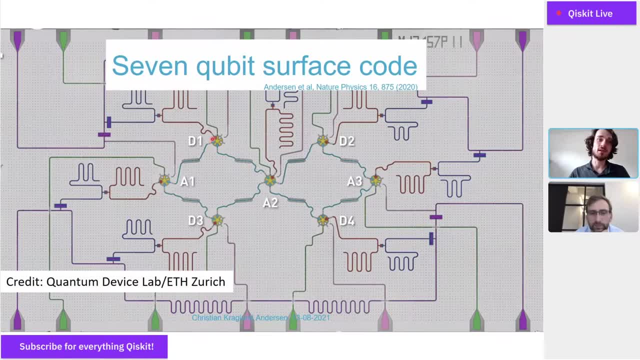 But it sort of comes for free without making the coupler at the qubit larger, and you'll need to change your frequency. So it's all you get just a little bit of speed And the big dangling capacitors off of the purple lines. 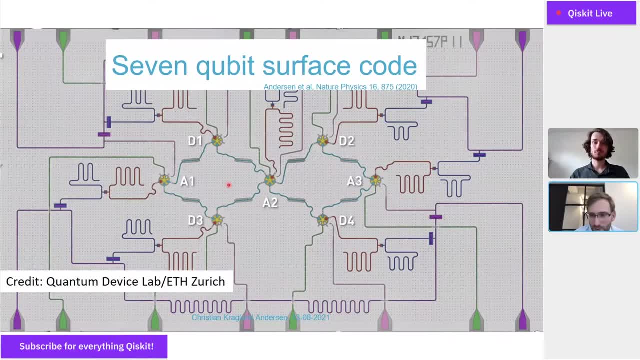 how much do they perturb the transmission, the transmission? Do they create a lot of wiggles and dips, or it's not much of an effect? Not much So it's a good observation. So you have this capacitor. It's really a capacitor. 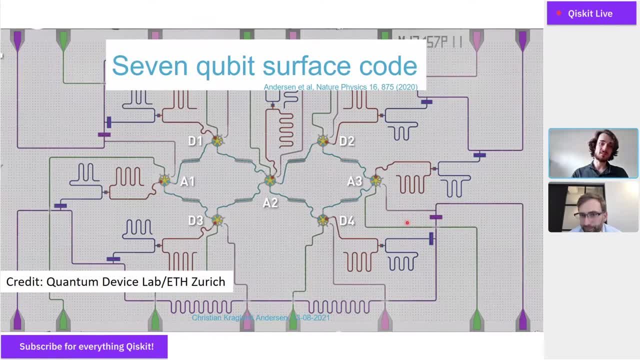 What you normally. if you just forget all the rest of the circuit and just have a capacitor in a 50-ohm line, you would have sort of a flat rising transmission. So this would in principle be fine, But what happens now is that 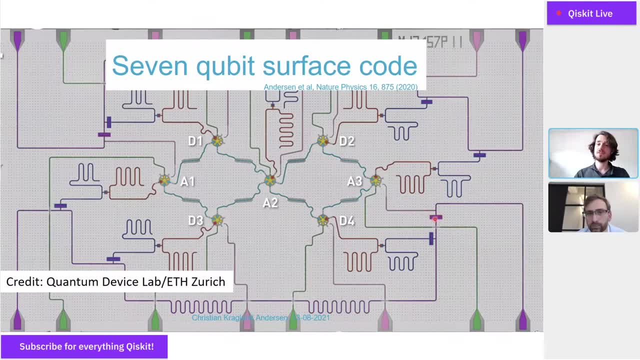 Ah, Because there is a capacitor. here you actually create sort of a semi-infinite line, in a sense that you have, by designing, a voltage antinode sitting here Because you want to cobble to your readout capacitor. it needs to be at these voltage antinodes. 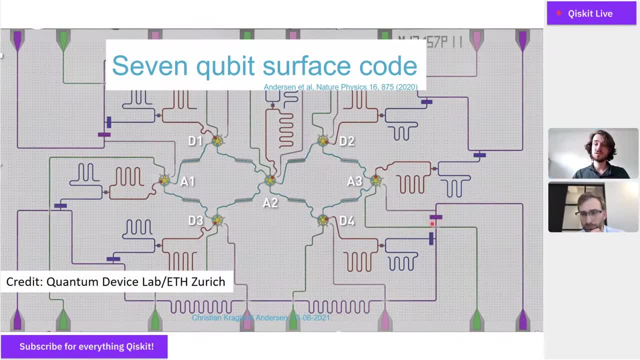 So you need to make sure that either you are at zero distance from it or that the distance from this input capacitor is a multiple of lambda. So this is why there's sort of extra wiggles here to make sure that the distance then over to this part. 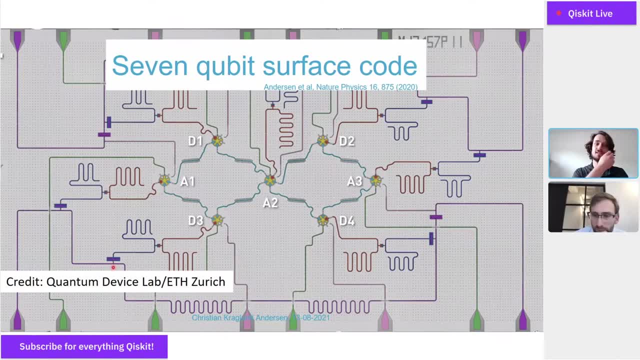 matches this lambda, which is the wavelength of your readout, And then there's sort of a few tricks that you can then play. That, OK, you see that this one is slightly different frequency than this, So that's why you can place it a bit further away. 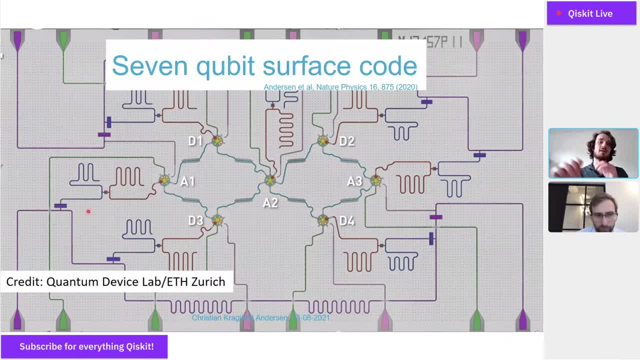 And you can lay it off- for the fact that they don't have the same wavelength And they are far away from each other. So that's why you can place it a bit further away And therefore also you need a slightly different distance. 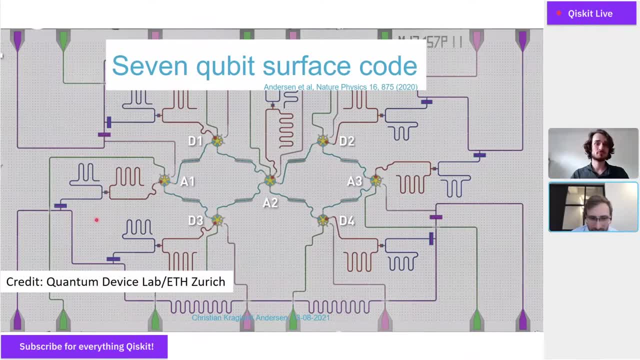 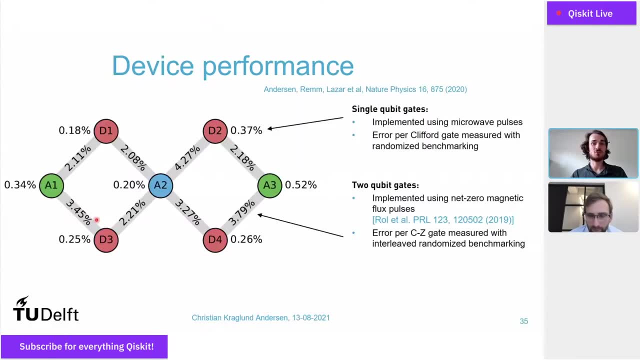 Awesome, Nice. Thank you very much. Then I will move on and just talk a little bit about how well does this device then work. So if we just look at the single-tubed gates, we have characterized them with randomness, We have randomized benchmarking and we get sort of errors. 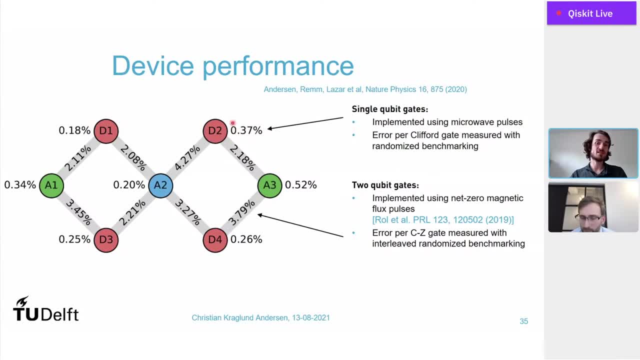 at this few tens of percent for the various qubits, Some a little bit better, some a little bit worse, which mostly comes from the fact that the qubits have different coherence. Similarly, we have characterized two qubit gates with what's called interleaved randomized benchmarking. 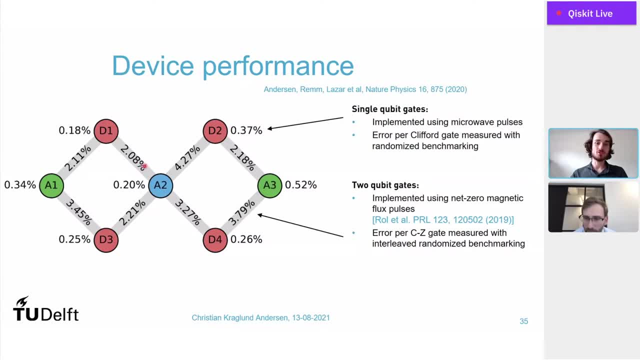 And they are. the range is sort of from maybe 2% to something like 4% in this case. So it's not quite at this error correction threshold that I mentioned earlier, which was maybe a bit sub-percent, but it's getting close. 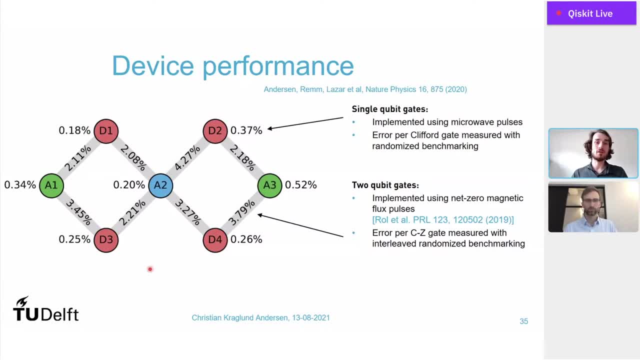 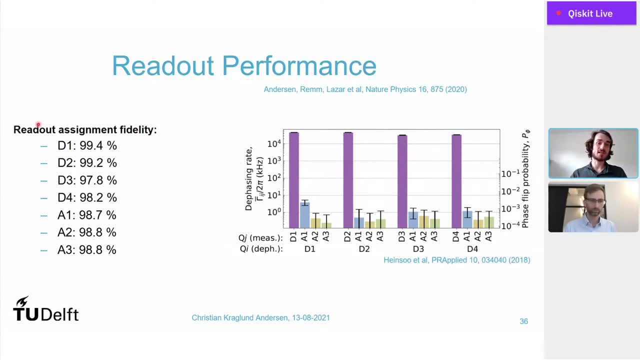 So this, I think, is looking quite good overall. So let's see also how the readout works. So here is sort of the readout assignment fidelity. So this is the probability that we read out a qubit in the state that we would prepare our deterministic state. 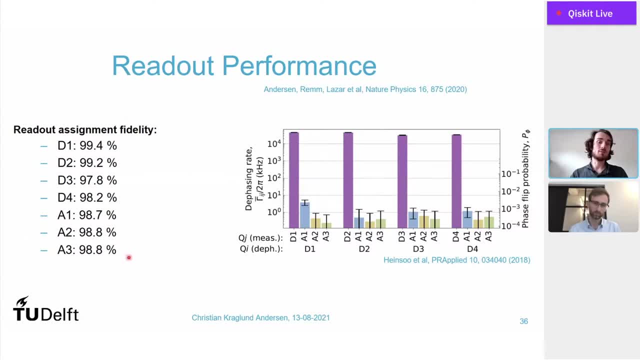 OK, You see that we can read those out with sort of probabilities of 98% to 99%, which is fairly good. Then the one thing that I really want to emphasize here- I mentioned a bit when I talked about the device- is we also want to not have crosstalk when we're 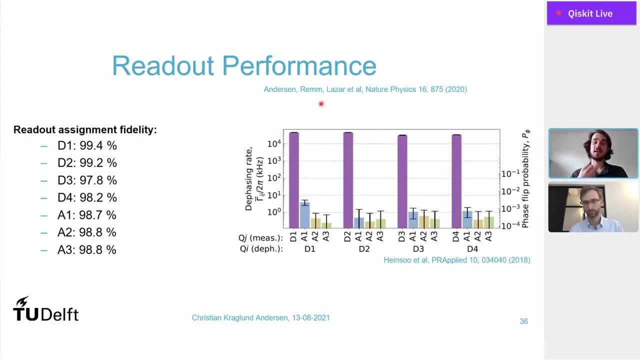 reading out the qubits And a way we can quantify that sort of very specifically is what we can do is we can take one of our data qubits, for example D1, and then we can say: OK, how much Does D1 deface if we are reading out one specific qubit? 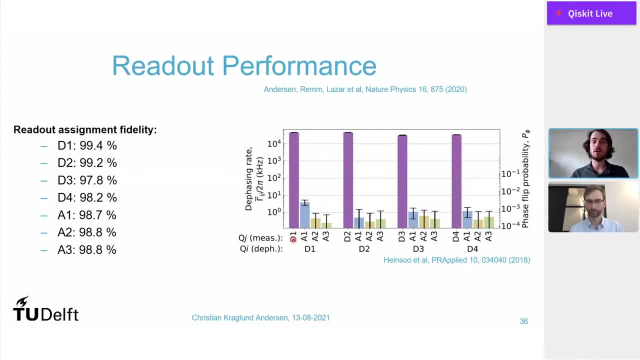 So we could look at that. How much does it deface? if you read out itself, OK, then it defaces a lot. That's what you want, right, Because that's what a measurement is. But if you're reading out one of the ancilla qubits- 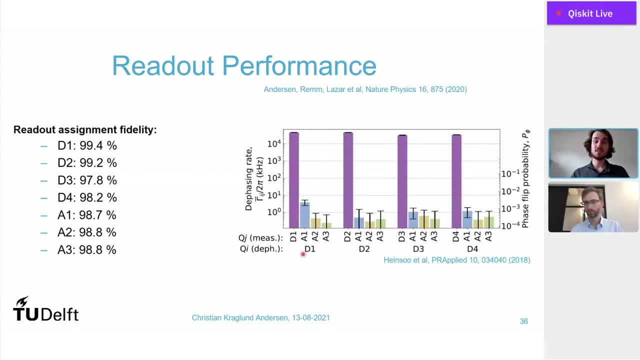 you see that the defacing of basic qubit one is really like five to six orders of magnitude less than if you were reading out the qubit itself, which is really achieved by the fact that we have these individual percent filters on the device. 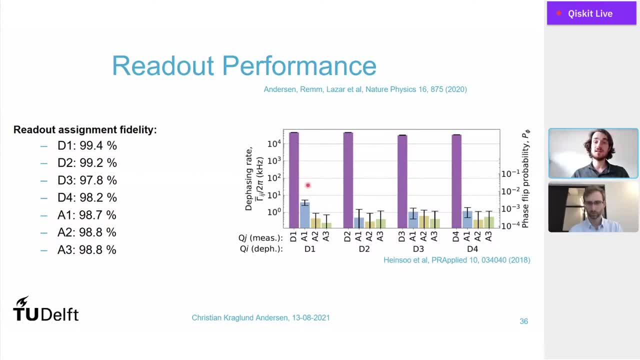 So this comes essentially for free once we have the device, that we have this very low crosstalk And- OK, now I'm talking about grades. You can also translate that into: what does that mean in terms of probability that you have an error? 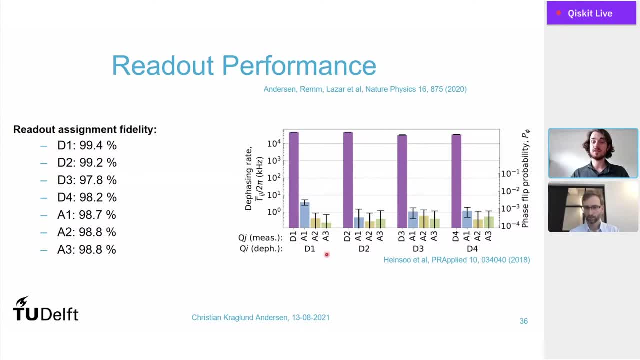 So it really means that if we are reading out one of the data qubits, the probability that there is a, say, phase flip error on one of the qubits is sort of on the level of 10 to the minus 3 into the 10 to the minus 4, which is really tiny. 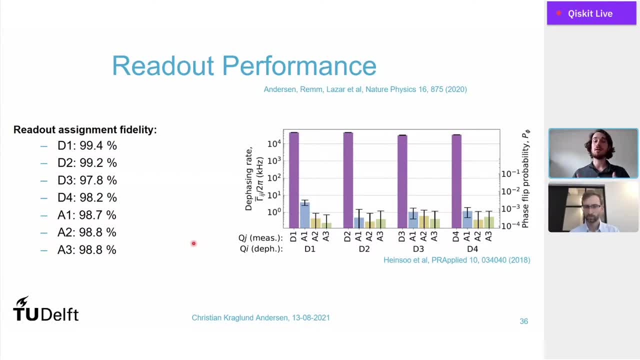 So that means that we can sort of safely measure our ancilla qubits while the data qubits will not be affected by it? Quick question before you move on. This is maybe a little technical, but just to understand when you say: read out assignment. 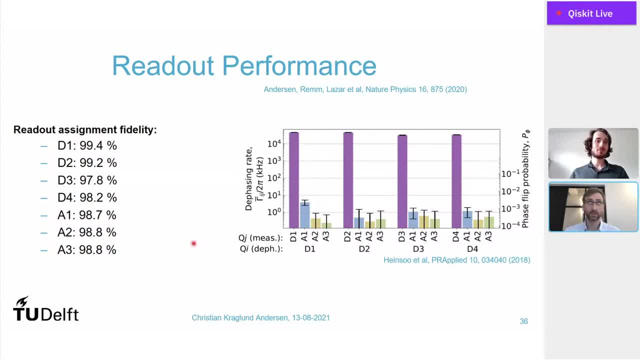 fidelity. I've seen two different kind of definitions And I think Andreas has used one with something like 1 minus 2 times the conditional probability of getting 0. if you had a 1 plus, sometimes there's 2 and sometimes there isn't. 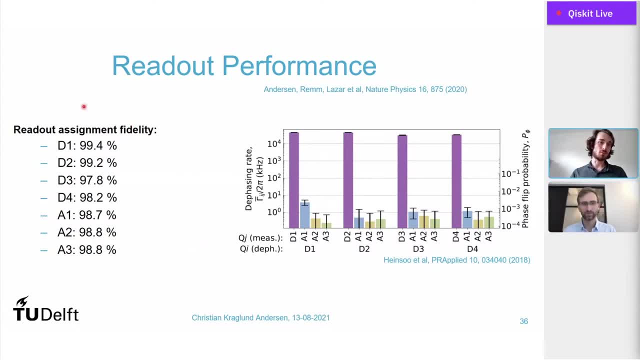 Yeah, exactly. So this is the assignment probability in the sense that this is really a real probability. This is a probability that you get the right outcome if you have a specific state. So it's 1 minus the average of the The average. OK, got it. 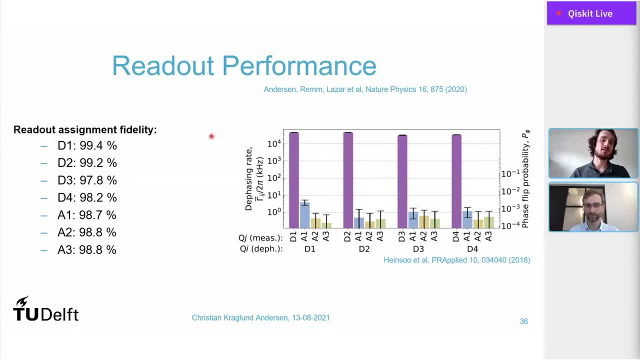 So there's a 1 over 2, got it? Yeah, exactly. Which means that if you would be completely random, this number would be 50% and not 0.. OK, so it goes from 0 to 1, not from minus 1 to 1, OK. 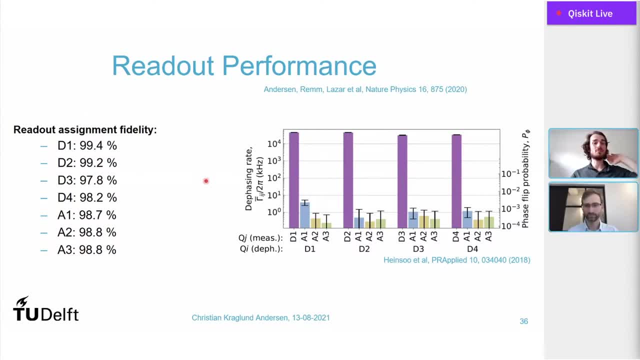 Exactly, And I like this way of defining it because this is a bit easier to generalize. to more qubits: If you have one qubit, you can go from minus 1 to 1. But if you have, if you want to read out, 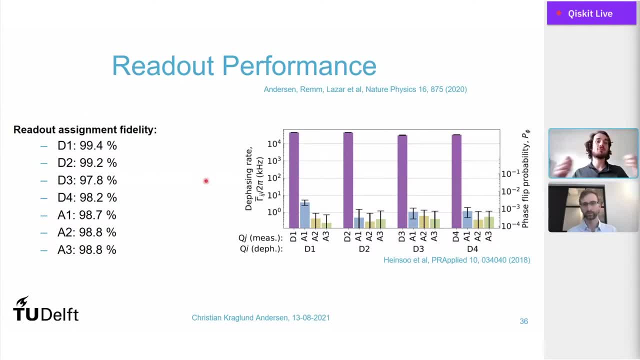 the state 0, 0, 0 of 5 qubits, then will it then go from minus 4 to 1?? I think that makes less sense to me, But if it's probabilities, it's always between 0 and 1.. 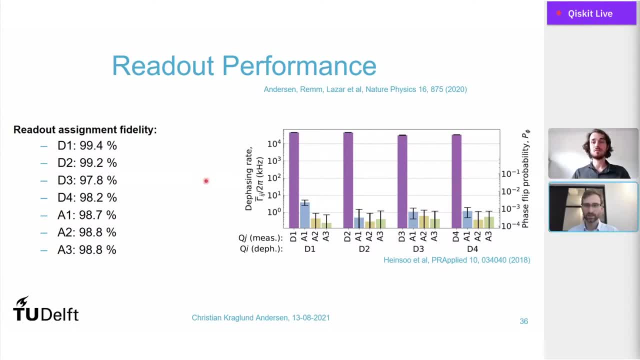 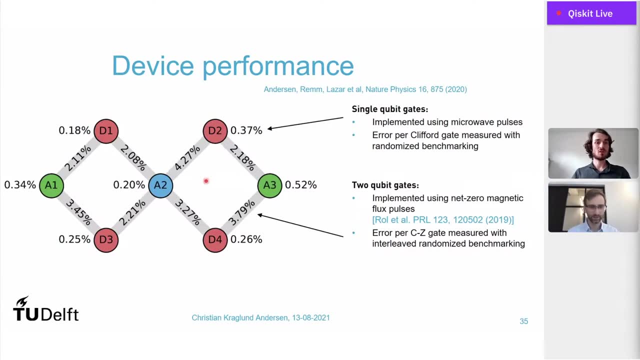 And a quick question- I missed it earlier- from the audience on: is it necessary to hook up the data qubits in a square like the schematic we see? Or what about other topologies? Yeah, So for the surface code, this is really. 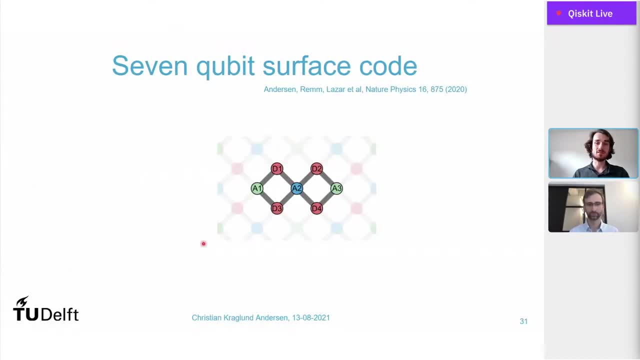 how you should hook it up. So let me show you all the way back. So the surface code is really sort of as square lenses. here In the surface code you also need to measure these so-called weight 4 parity measurements, meaning your ancilla qubits really. 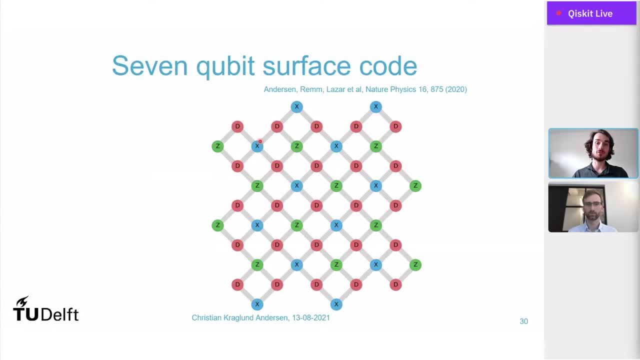 need to connect to 4 qubits if you want to do the surface code. If you don't like to connect to so many qubits, there's other codes Which have its own pros and cons. One of the pros of, for example, something 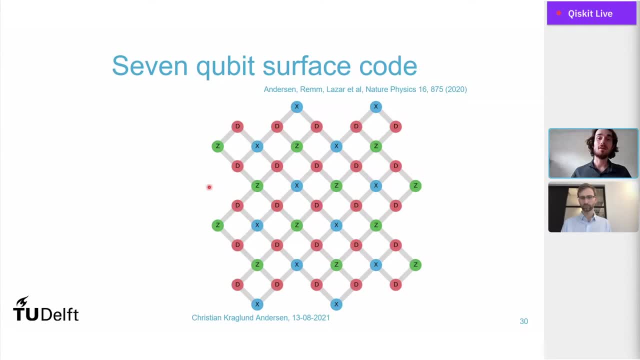 called the heavy hex code that I know IBM is pursuing There. you'll need less connectivity but you don't have as high threshold for both type of apps. So that's sort of a you can pick and choose a bit in terms of how do you want your connectivity. 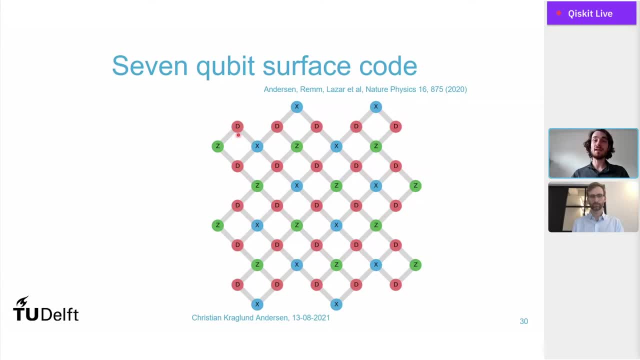 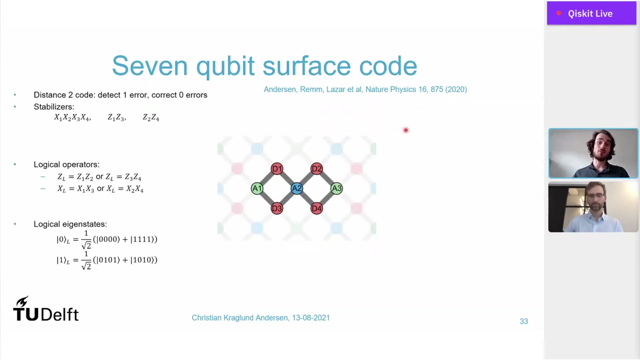 The surface code is sort of. while it does require high connectivity here, it has sort of very well-defined structure otherwise, which makes it nice for matter if you really want to implement it And, I think, for the way we designed our qubits here. 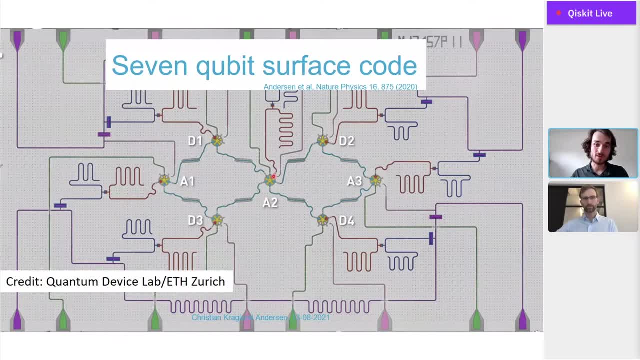 it also comes very natural. So what you can. I didn't have a zoom in on the qubit, but what you can see here is that the qubit has sort of this circle size with sort of five connections from the side, And that way it's very natural for this design. 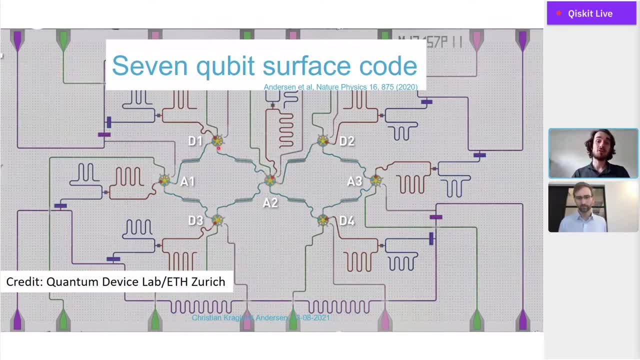 to connect to four neighbors And because we use the frequency-tunable qubits, we are also a bit more relaxed in terms of having frequency collisions with neighbors. Exactly how that works, that's in this paper by Ferslois that I had a few, maybe 10 slides ago. 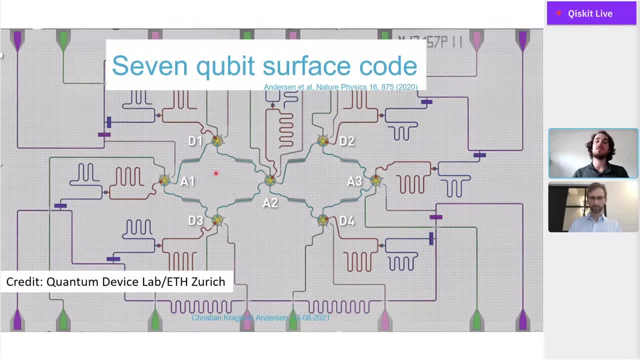 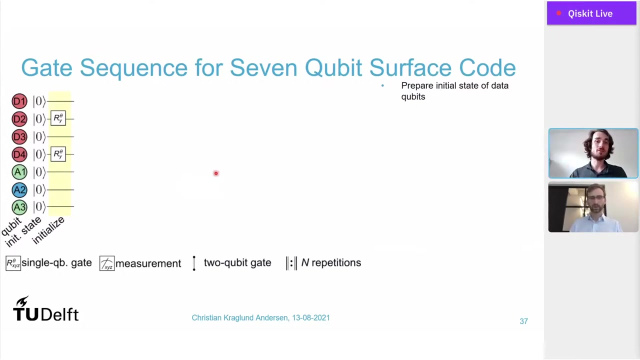 But exactly how should you tune your qubits to avoid that you run into problems with frequency collisions? So it's a challenge to have this dense connectivity, but it's something that you can do. I hope that answers the question. So with that we're going to move on. 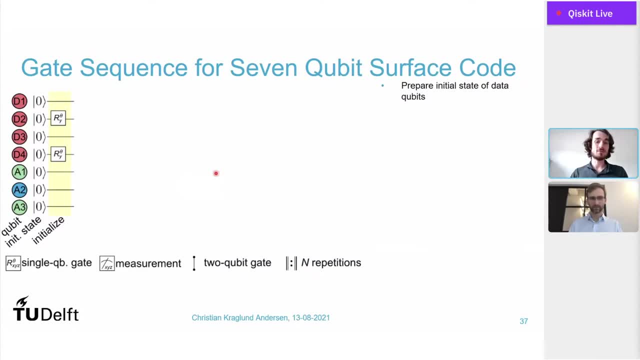 Thank you And say that, OK, now we have looked at the individual components and seen how they work. so let's actually do the surface code. And the way we do that is, we're going to do it as we start with our seven qubits, our four phasor. 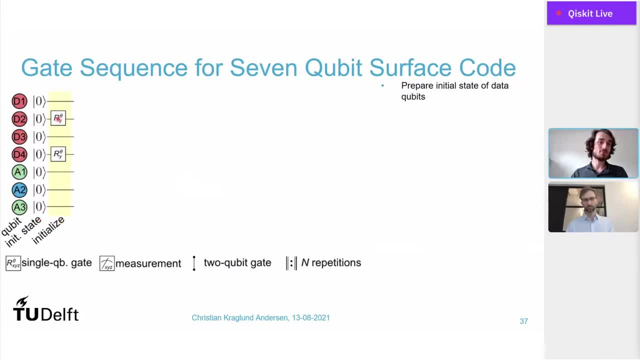 qubits and the three ancilla qubits in the similar state And then to initialize on a specific state. we can do some initialization And then the error detection begins. So we do the circuit that I really mentioned before. Here we start with the xxxx measurement. 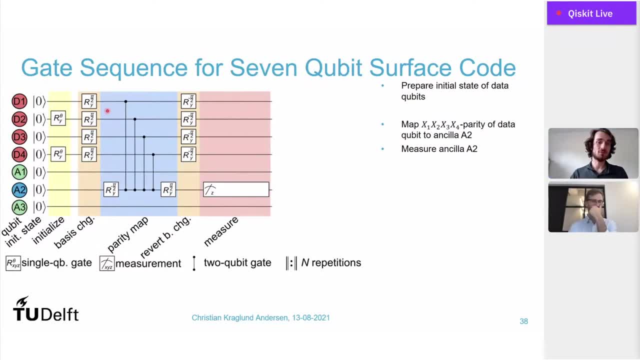 So we do our basis change. then we do the so-called parallel measurement, So we do the so-called parity map, where we really do this set of four gates, map it onto the ancilla qubit And then what we do is we measure the ancilla qubit. 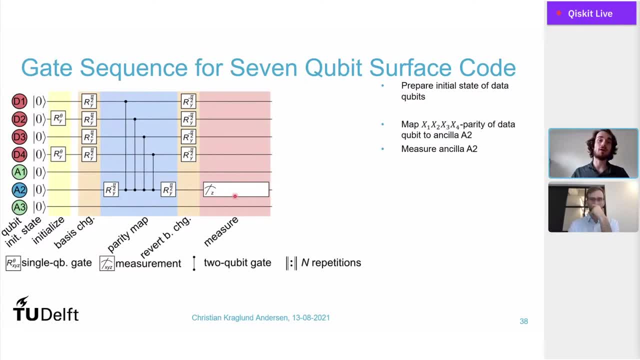 And then we see: was there an x-type of error on our data qubits indicated by this machine? Now, because we have this very low crosstalk from the readout, what we can do is that, while the measurement is really going on, 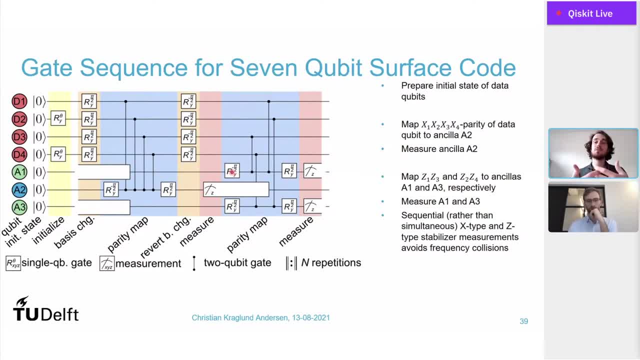 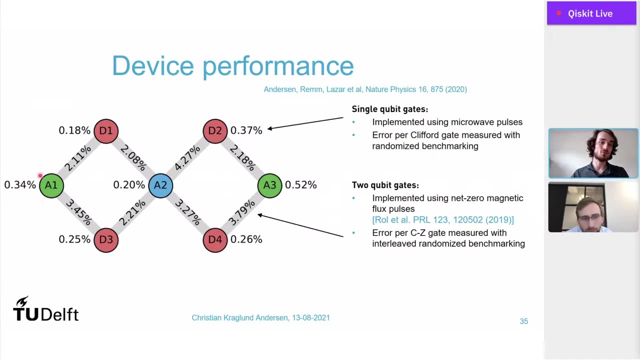 this data, of these ancilla qubits, we can start by doing the set type. So now we do these two set two. So here it's only because it's an edge. So you see, on the edges you always only have two neighbors. 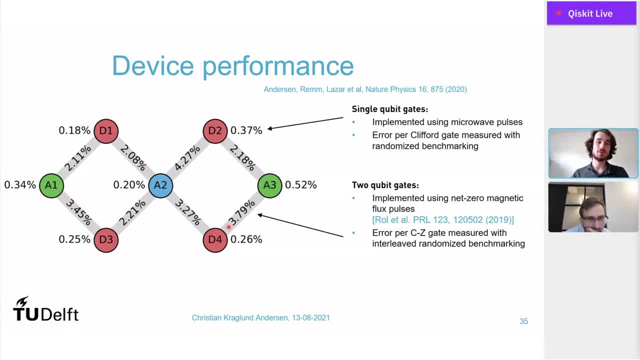 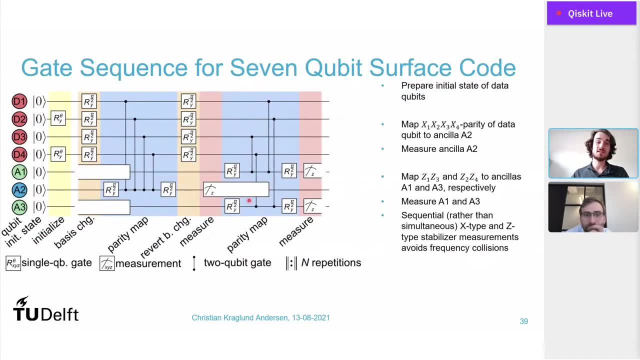 For the set type of error. there's only two neighbors for each ancilla, So we do those in parallel here while the measurement is still going on on the ancilla qubit. This is not a very precise timing diagram, but it roughly takes until the middle. 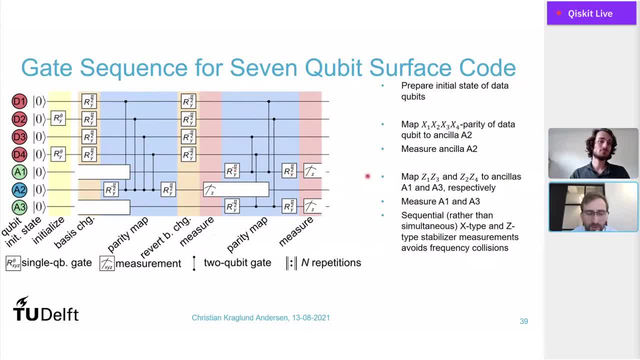 And you saw that doing this during the measurement as opposed to after didn't really affect the results very much. No, I think exactly There's two things to that right, Because our two qubit gates are already. the error on the two qubit gate is on the few percent right. 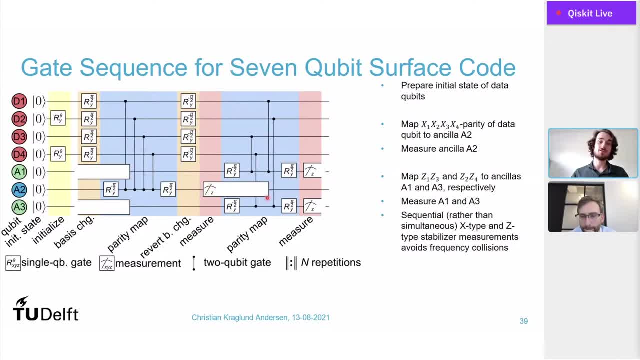 Where you saw the error coming from. this measurement was sort of on the sub percent 0.1 or even below that. So maybe if we had much better two qubit gates we would see it, but at the current states this does not make a difference. 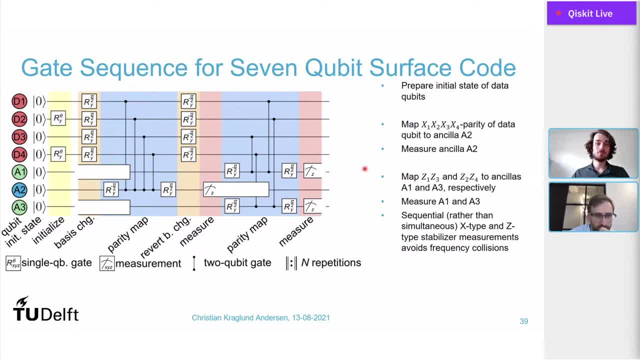 Right, And then at the end we do the measurement of the set of zippers here And then, because we want to keep our qubit information alive, we just repeat it and keep checking. is there x-type of errors? Is there z-type of errors? 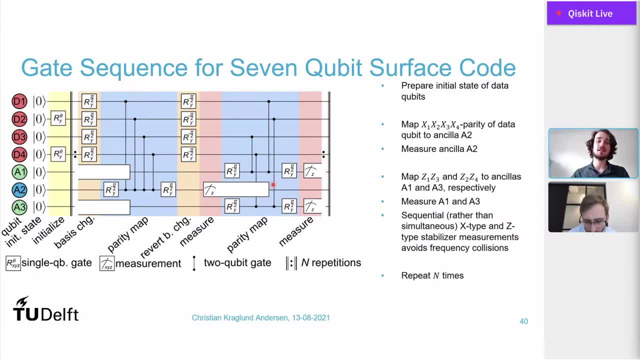 And again are there x-type errors, z-type errors and so on, And what we can then do is that we can keep some of the data until we find an error, Because we cannot correct it at that point. we can really only do one thing with this small code. 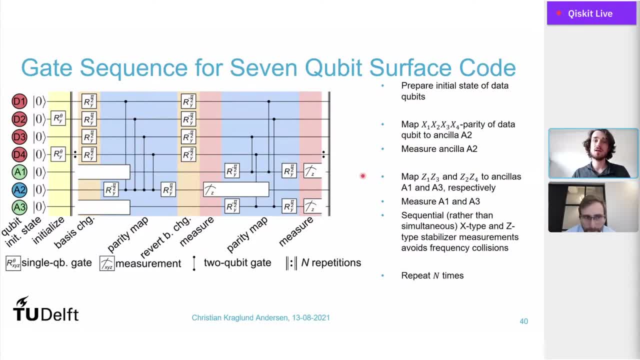 and that is to discard the data, whether it was there. But if we just keep the sort of post-selected data here, post-selected on sort of very honest criteria that we did not detect an error, we can then verify that. indeed, in those cases, 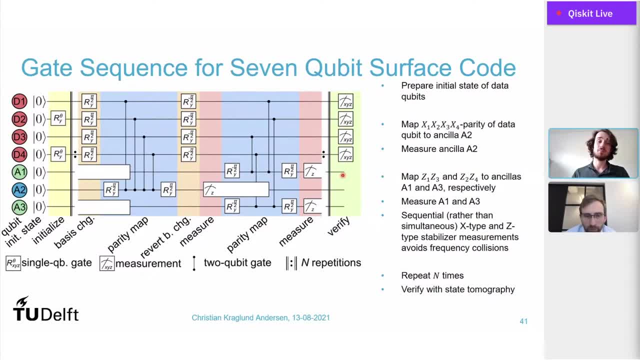 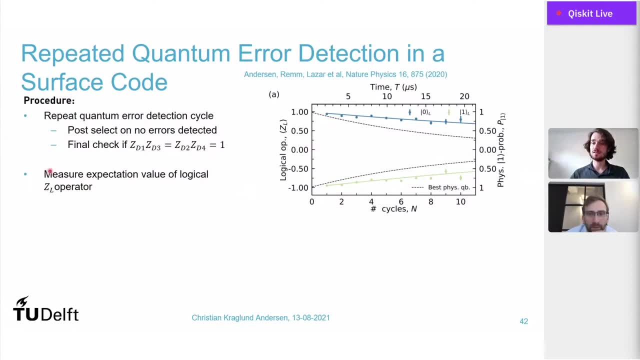 the quantum information was kept in our logical qubit. So let's do that, And here we do it for up to 10 cycles of quantum hyperaction or error detection, But we really just repeat this circuit that I just showed you, And then at the end we measure the logical set operator. 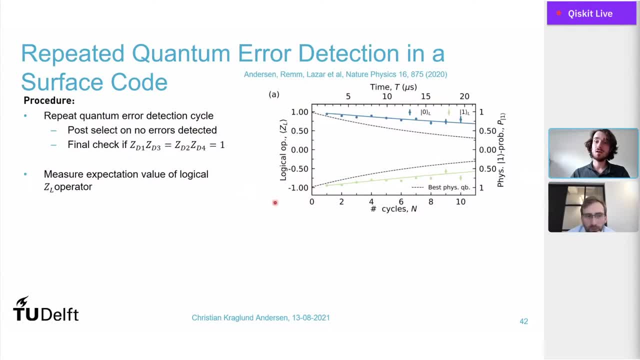 that I also showed earlier. And then what we do is we just either by starting in the logical zero state or starting in the logical one state, And you see that that sort of decays long. So here's number of cycles. You can also plot it in real-world time. 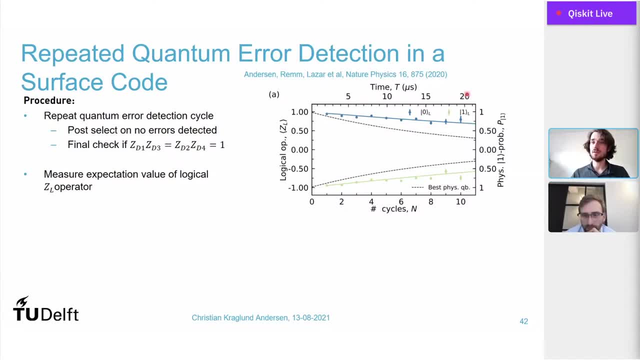 And you see that, OK, it decays a bit over a timescale of maybe 20 microseconds, but not so much. So to compare it to something, you can look at the axis that I have here on the right-hand side. It goes from sort of 0 to 1 in both directions and plots. 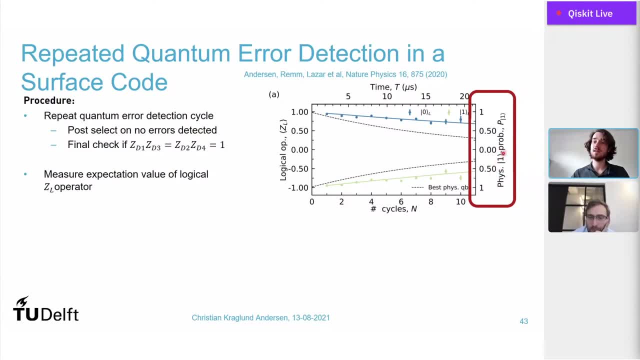 what would happen to the best physical qubit if we had it in the one state. So this is really what is sort of a typical T1 decay of the best qubit, And you see that here in the dotted line. And for the best qubit here, the best T1. 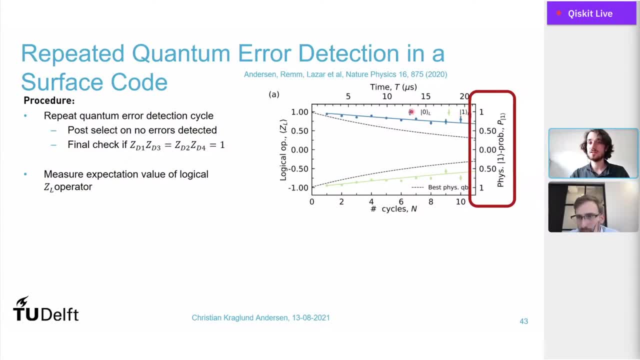 was close to 20 microseconds. So you see that from here to here you have loss of 1 over And you see mostly that here, for both the 0 and 1, the logical qubit decays slower And the best physical qubit meaning. 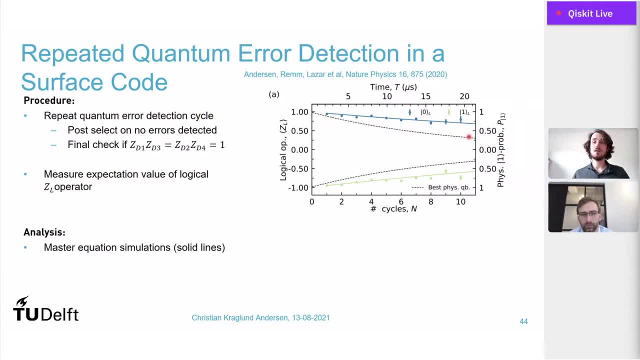 when we post-select the errors here, we really have a longer lifetime. The logical lifetime is really longer than the best physical lifetime in this system. Just to verify that this is really well understood, we also did a master equation simulation. That's the solid lines that you see here. 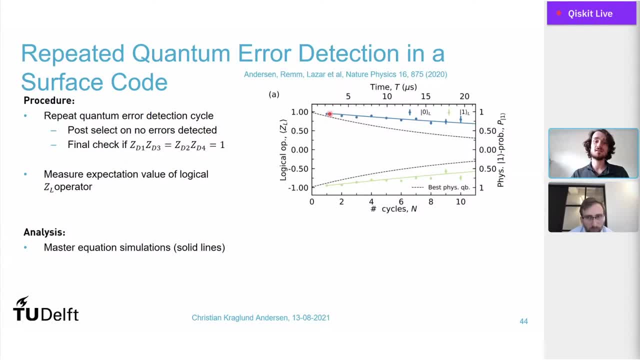 So those are actually not a fit. These are really simulations And you can see that these are the results of the experiment, based on independently measured the quantities, such as T1, T2, residual set, set and gate times, And you see that this follows the data quite nicely. 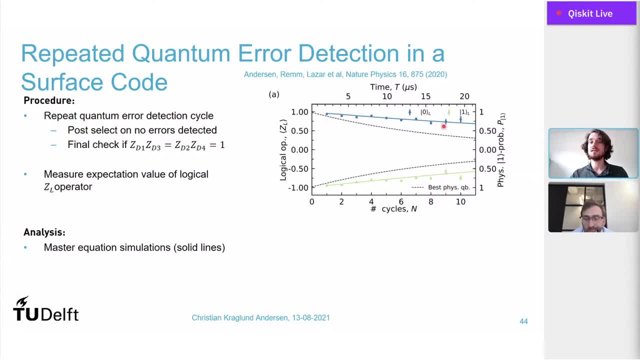 Maybe at the end there's maybe a bit change, because what happens really is that every time we have an error, we have to throw away some of the data, So the error class gets quite big. So this is how it works for the set. 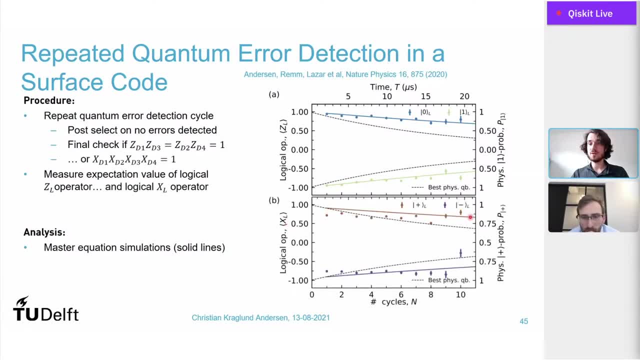 For the X. we are maybe not winning as much compared to the best physical, because T2 is a lot larger than T1 for the best qubit, But we are still surviving for just a bit longer. meaning again also for the logical X operator. 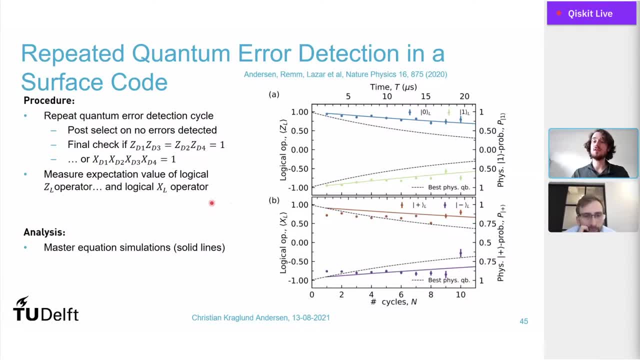 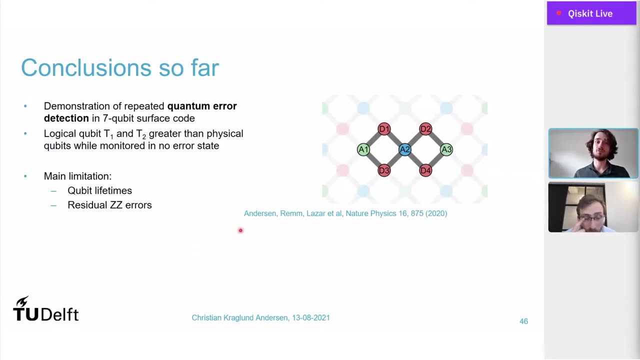 we are winning by doing this error detection in terms of getting longer appearance times for our logical Q. So these are some of the results that we got in this recent publication, And with that I want to just make a brief sort of first conclusion slide before moving on to the outlook. 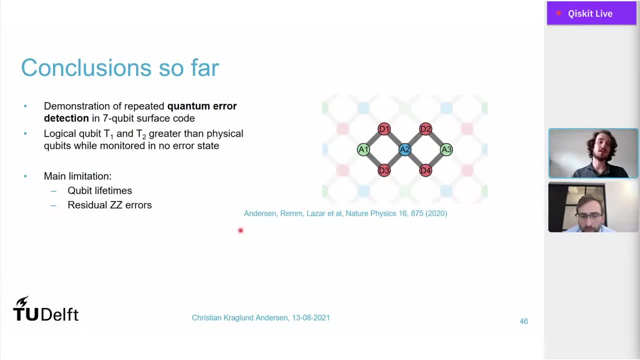 of where we go next. So I really want to say that it really excites me that we really demonstrated that the surface code works as expected And also that we saw that when we do this error detection, we can really get better performance here in terms. 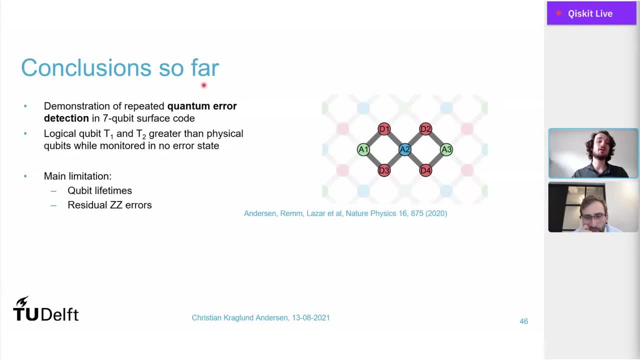 of T1 and T2 than the best physical qubit that we had at that time And because it matched very well with our master equation situations. it was also clear for us to understand what was the limitations. That's really due to the fact that, because we had somewhat finite qubit lifetimes. to begin with, the sort of threshold for getting better logical performance was not quite there yet. So if we would go- even better lifetimes- we would also get much better gate, which would give even better logical performance. which is how the error correction works. 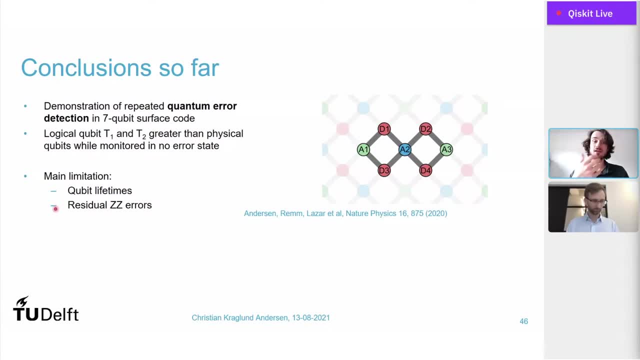 And then the second thing that showed up in our simulations as mattering somewhat from these results is that between T1 and T2, the qubits- when we are not doing a 2-qubit gate, they're sort of still weakly interacting. 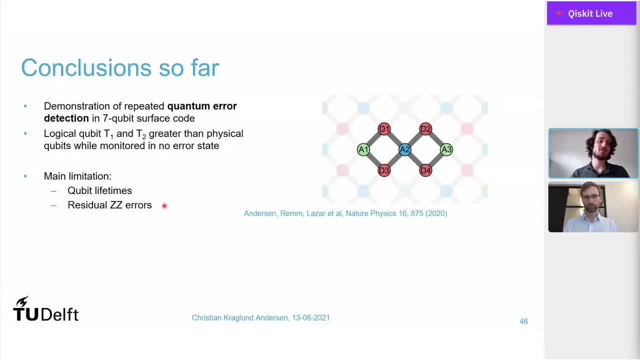 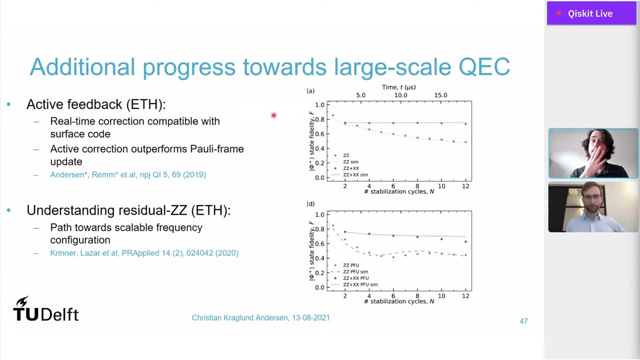 And this also adds up errors for this so-called residual set set. To then move on a bit and look towards the future, we did also two other experiments that I briefly want to mention just in one slide here. One is that we looked at active feedback, because at the end, 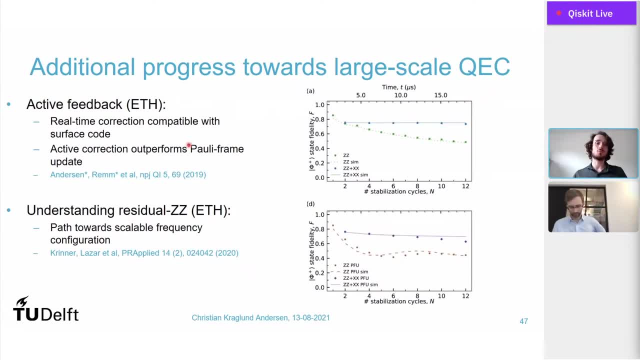 when we have our surface code. we also want to actually correct the errors on the device in real time. In the error detection that I showed you before, we just throw away the data when we see an error, so there's never any correction. 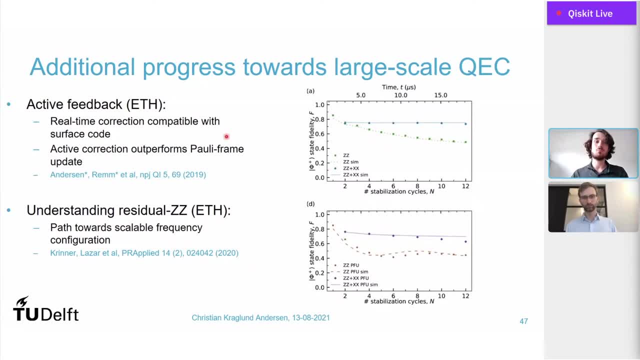 But we would like to actually do the correction. So we did sort of a very simple experiment for that, where we just had a single state here, a bell state, so a highly entangled state, And we used sort of a scheme that looks like a surface code. 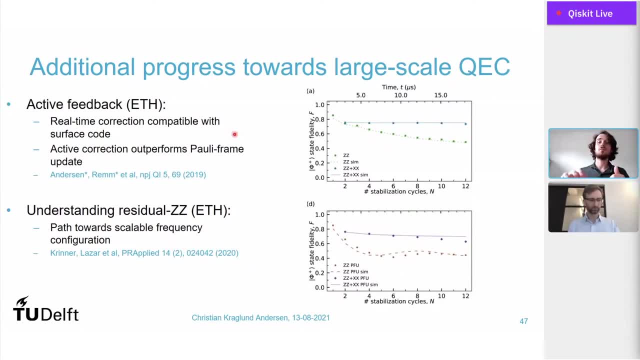 to measure: are we still in this bell state? and, if not, we used real-time feedback to correct the state, And we saw that this could. if we were looking for both X and Z errors, we could really keep the fidelity constant, while if, for example, if we are only looking for Z errors, 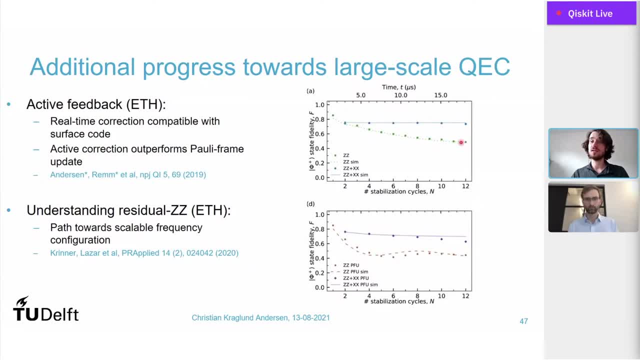 we would sort of lose half of the information. So we can really see that we can correct both types of errors, And one very interesting aspect is that what we saw is that actually doing this correction, even though on paper it would not make a difference, 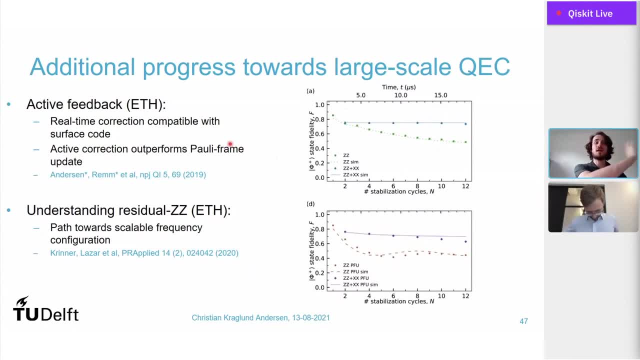 we would, in principle, be able to do the correction after the fact, But because of these residual ZZ terms that we have, they actually add up if you don't do the correction on the fly but instead try to do it after the fact. So this we found very interesting. 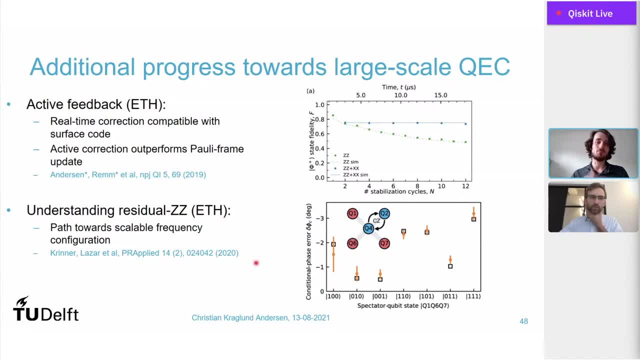 So we also looked a bit more into the ZZ because it turned out that in both our experiments that I showed it was very important. So we made a very detailed study about how these errors really add up coherently. So there are real coherent, correlated errors that you can quantify. 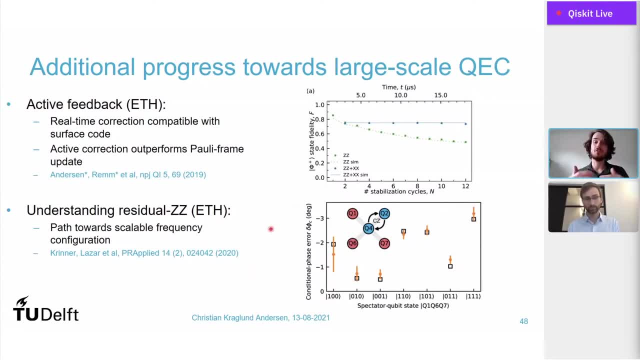 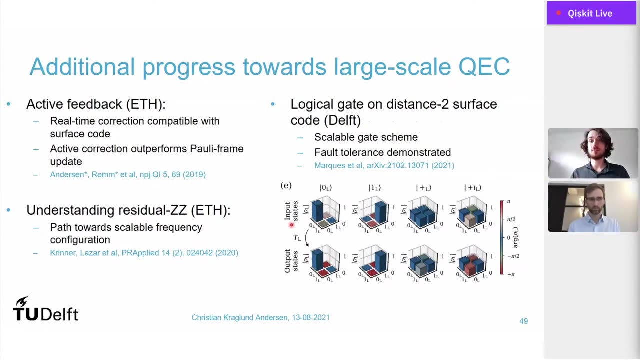 by looking at what is sort of the conditional phase that you get in your two-qubit gate in the presence of all these neighboring qubits that all have residual ZZ errors. Then a few results that I want to highlight, also that came up lately from other groups. 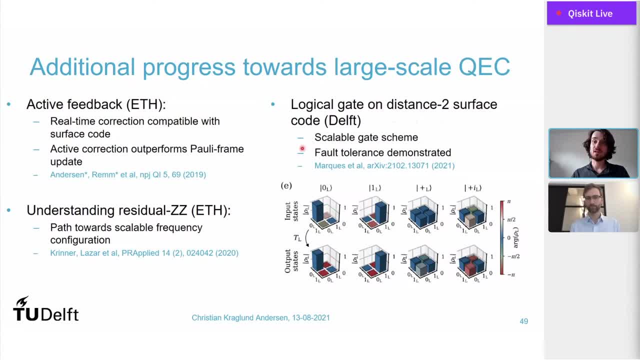 one from the group of Cleo Di Carlo in Delft is that they did the same type of experiment, so a distance-to-surface code. but they also went a bit beyond what we did here. In particular, they looked also at gates. 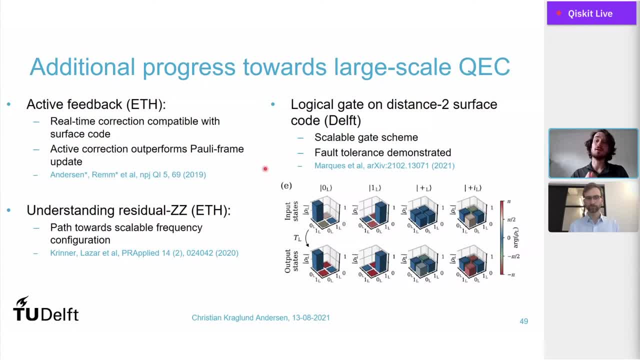 So they really showed that if you do a logical gate on this distance-to-surface code, they behave fault-tolerant, Which is very great, because in the end we don't want to just have memory right, We want to do computation. 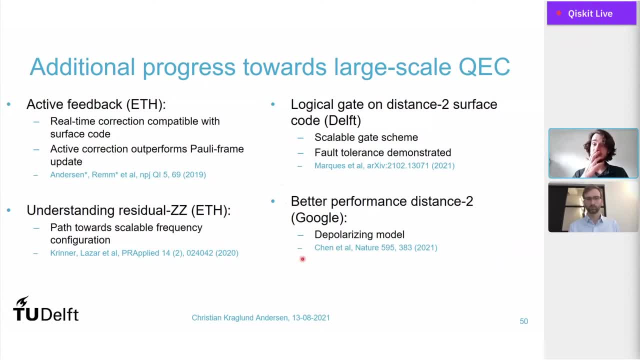 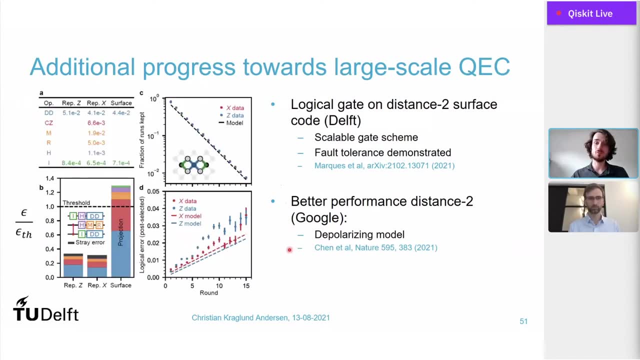 And the last experiment from another group that I want to mention here is from Google, where they really again did the same type of experiment, so a distance-to-surface code, a very similar gate scheme, And you see also in the drawing that they used the same color code. 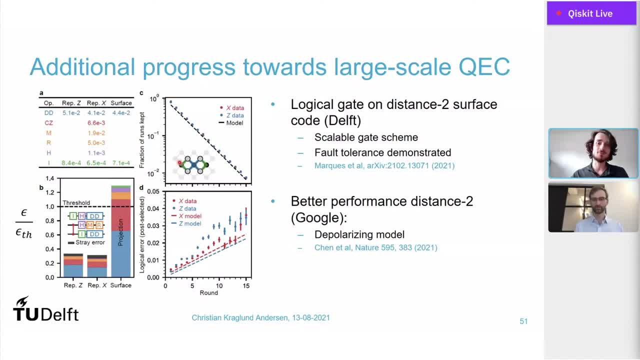 for X and Z, so it's really easy to compare this. They had somewhat better gate performance overall, so they have sort of better logical performance. But what they also did, which I think is really, really cool, is that they took this experiment. 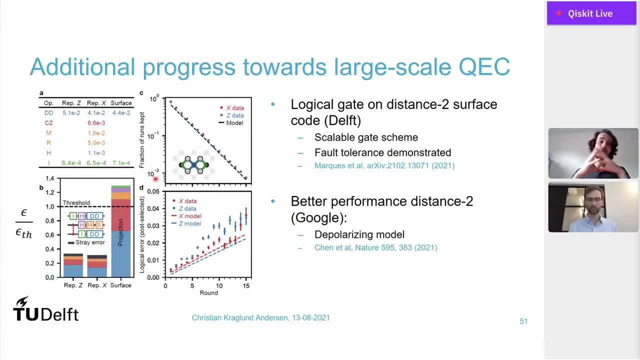 and they then compared it to a model that really compares it to the error correction threshold that I talked about in the very beginning. So you can look at this error and here's really the total error of everything divided by the threshold And they saw for their device. 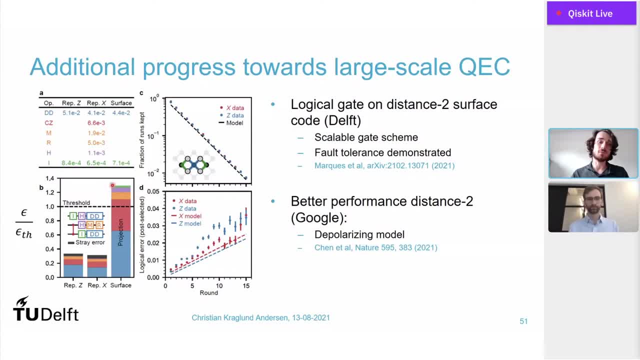 that they are still somewhat above the threshold for their experiment compared to the model, And then even beyond that. you see, it's a model. You see, for example, this data. so this is logical error after post-selection. So the data is here in dots. 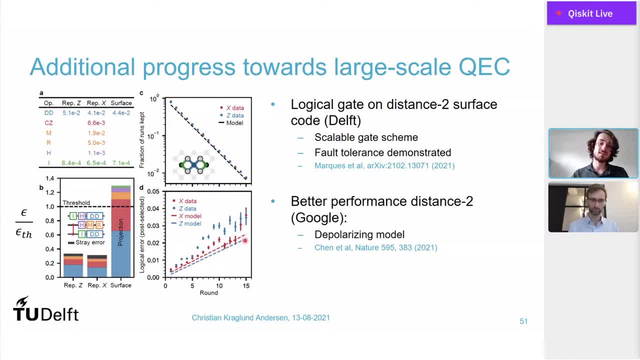 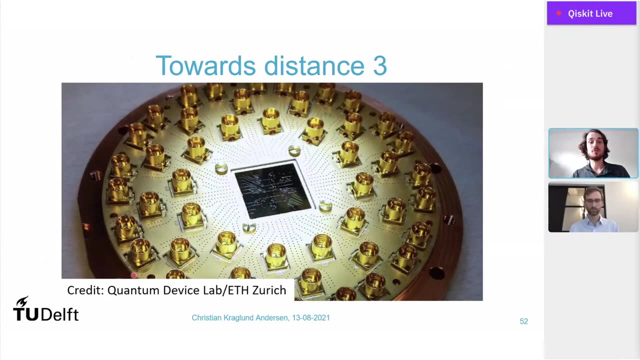 and then they have this dashed line, which mostly follow the data, but it's still somewhat different. That's because, even though they tried to model everything here, there's always some errors. that doesn't quite fit into the model, And this is really important going forward. 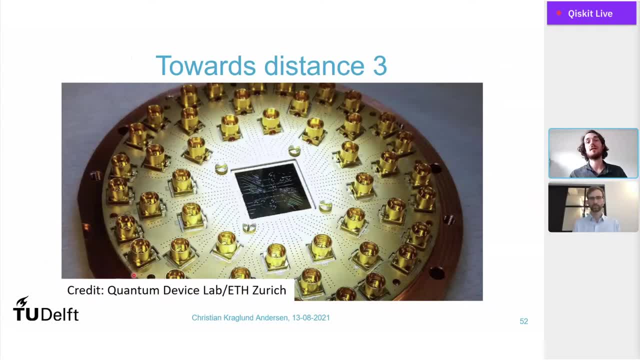 because what we eventually want to do is we want to do quantum error correction And what I mentioned is that we did a distance-to code which could only do detection. So to really show that you can also correct error, you need to do distance-free. 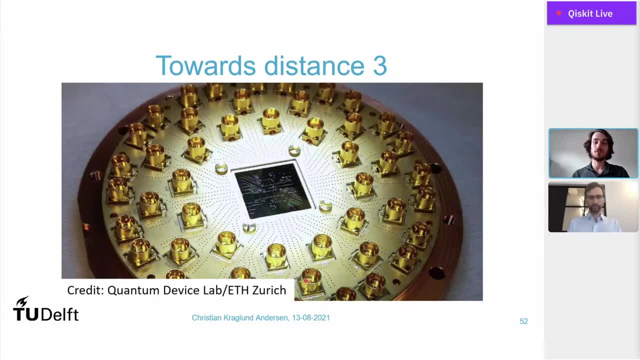 So in Zurich we recently made a first-generation device for that. So here is actually a 17-qubit device sitting again in a sample holder, similar to what I showed in the very beginning. If you zoom in again, the device actually looks very similar. 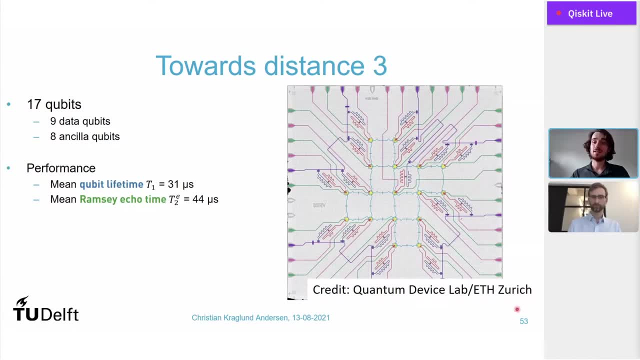 to the one that I also discussed in detail, except that now there's 17 qubits. You see, the data qubit sits inside of this pattern here, So it's like three times three patterns, And then the rest of them are select qubits. 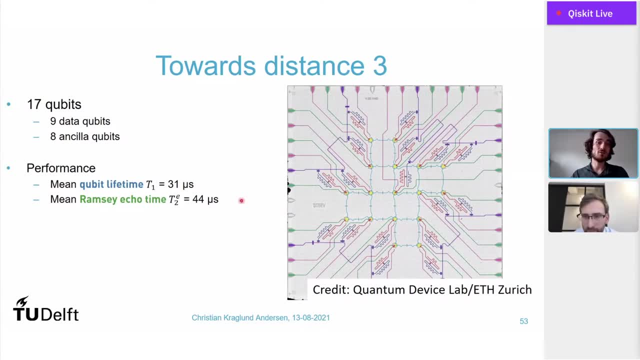 And in this sort of first-generation device we already got quite good coherence times. These are actually, on average, around a factor of two better than the seven-qubit device. So we managed to increase the number of qubits and also increase the coherence times of our qubits. 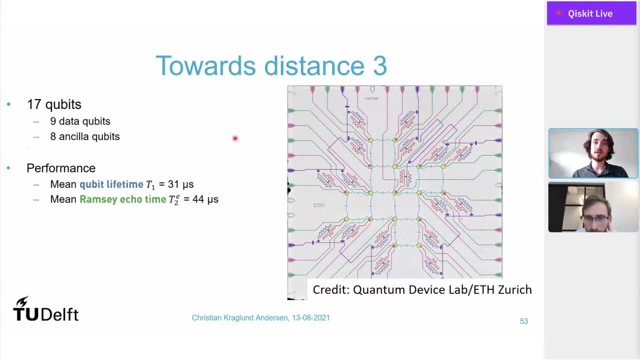 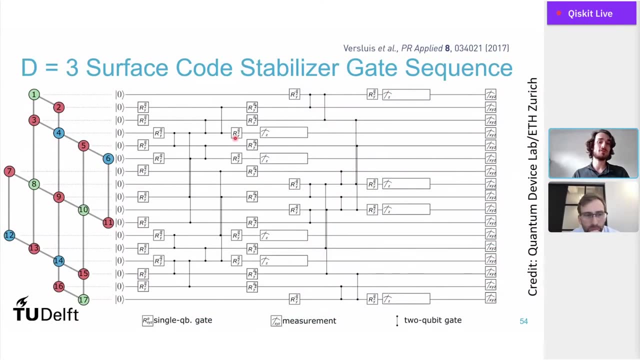 which is great. So this is still an ongoing experiment, but just to give you a feeling for what needs to be done, the eight-sequence bump for doing this service code looks like this, And this may look complicated, but I just want to show that it actually follows. 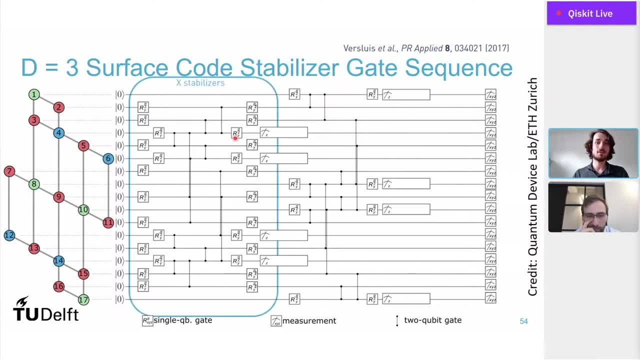 on this very nice pattern. So you start with the X gates or X stabilizers, then there's the Z stabilizers And then, after doing your initial single-qubit gates, you have these layers of two-qubit gates. They can really be understood sort of geometrically. 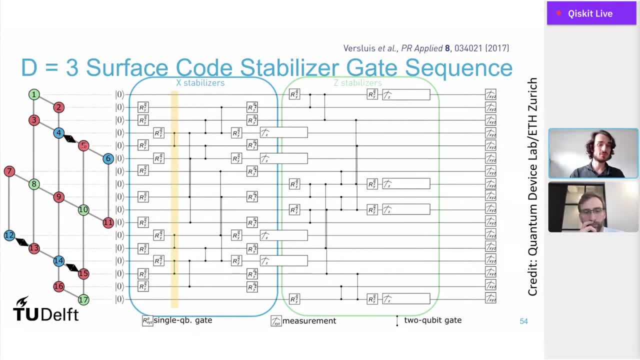 that okay, if you are here, you go first down here sort of south, what is that? southwest, southeast on the device, And then you go around sort of in a circle, then you go fully south, then you go northwest. 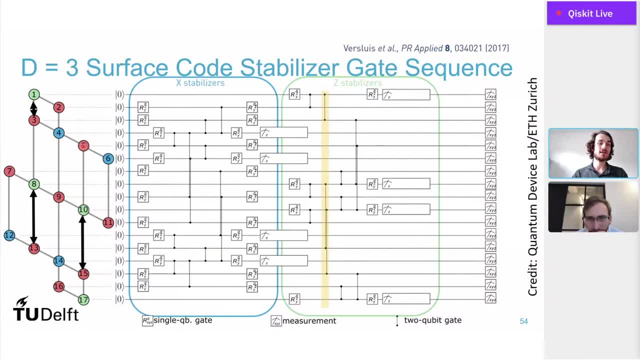 then you go north, then you go over to the Z and you again go in this circle, And this is also a way that I hope sort of convinces you why this is really a scalable way of doing data collection, because you can always go in this sort of pattern around. 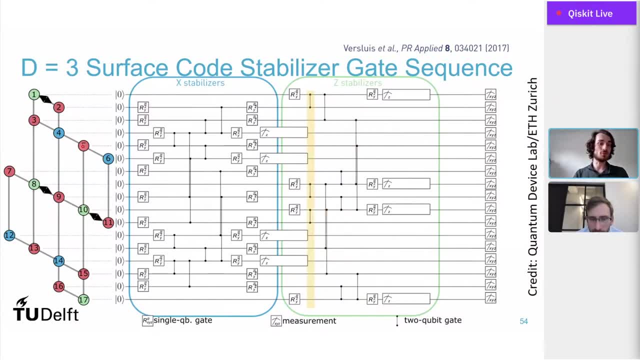 If you would have a much larger service code, you could still sort of go in this circle, which I think is great. This is an ongoing experiment, so I don't have any flashy data for this, But just to still understand, would this really work? 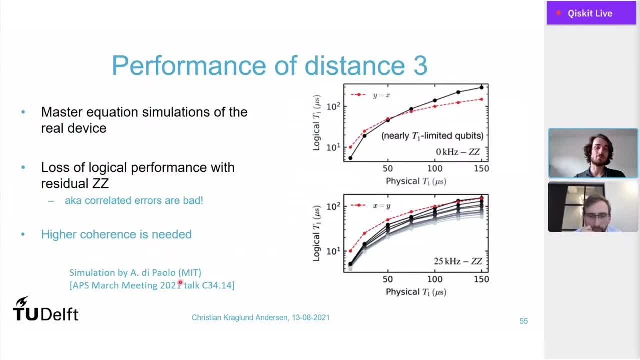 Together with Augustin Di Paolo at MIT, we talked about how this would look in real life, and he then did some numerical simulations of this. So he took the real device with the parameters that we have in terms of gate, maybe a little bit conservative parameters. 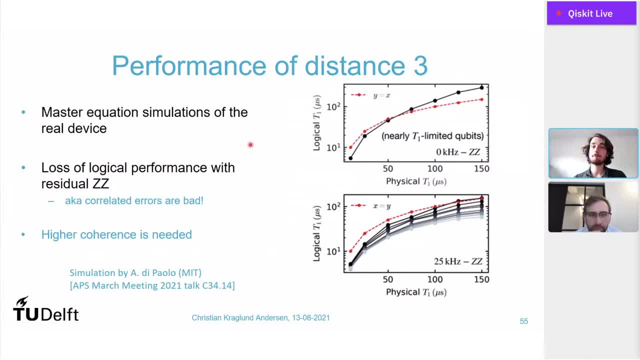 and said, OK, let's simulate the full thing. And then he put sort of average T1 here on his x-axis and calculated what would the logical T1 be after doing this sequence, And he compared it then to this red line, which is sort of the case. 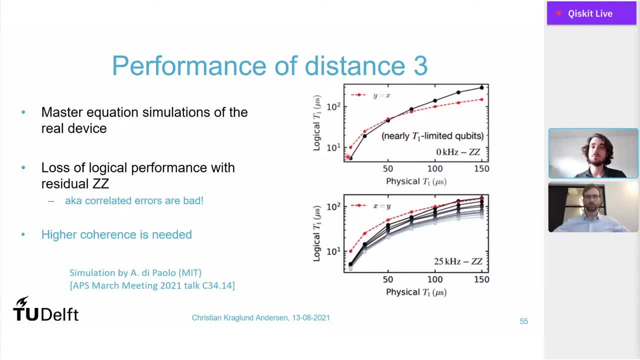 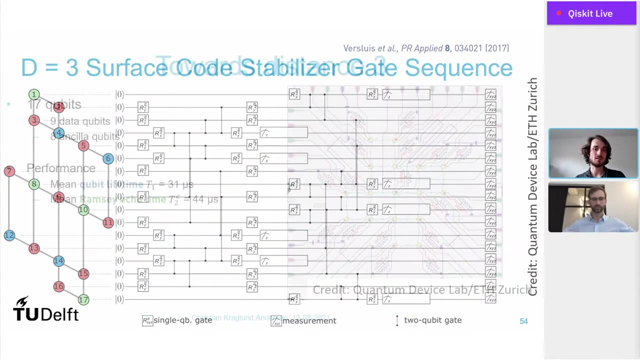 where you have logical T1 equals physical T1.. And you see that there's sort of a threshold, maybe around 50 microsecond, which which is somewhat higher than the number that we had. So we had 30.1 microseconds T1 here. 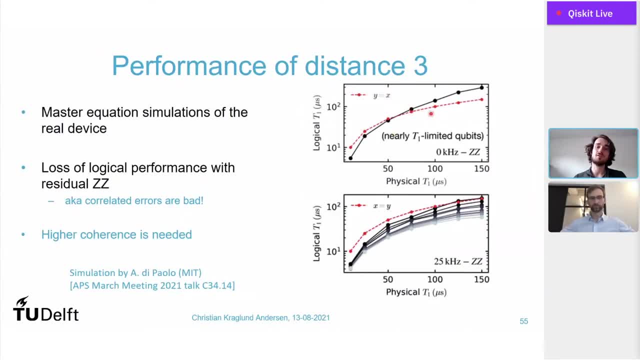 So there's still some way to go, but maybe we can also push it a bit in terms of gate time and we can make it a bit shorter. we can squeeze the sequences, But then a very interesting fact is that you can also add this residual Z-Z coupling. 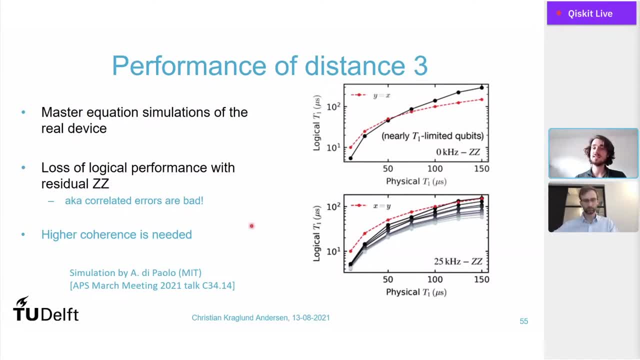 that we discussed before, And when you do that, it gets even harder to actually read this level. So even with a somewhat smaller coupling of 20 kilohertz, there's sort of required T1 time that you need to break even on the threshold. 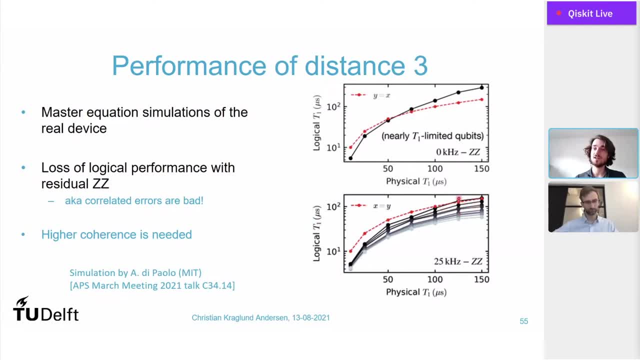 gets much higher. The different colors here are different readout performance, just to see how much effect this is. So the top one is for perfect readout and the light one here is for 10% readout, each percent. So we really need super good readout. 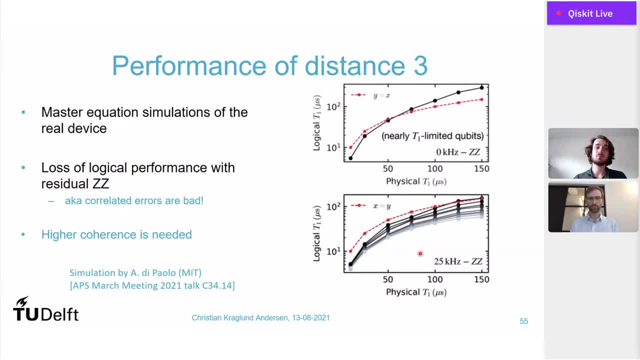 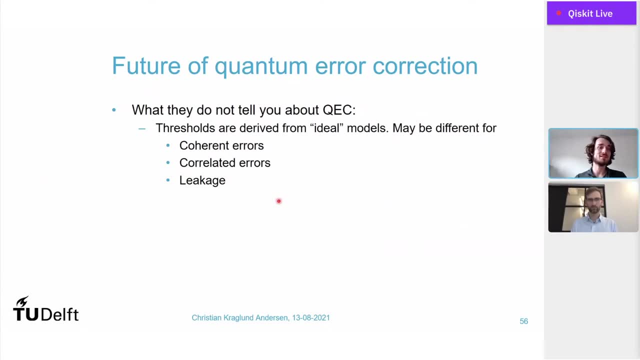 and we need very small of Z-Z, Which brings me to the take-home message if you want to move forward when I say the things they don't tell you about quantum error correction. So one of the things that often gets forgotten a bit is that 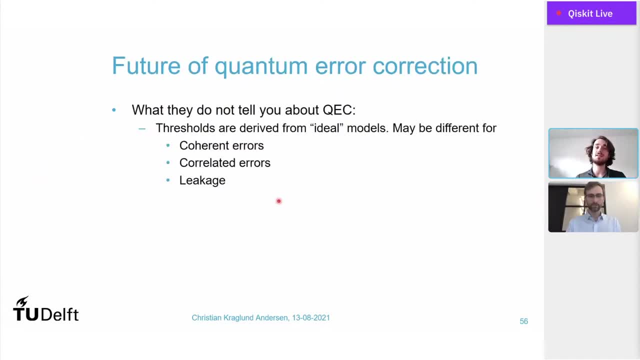 when you talk about threshold, they're always derived from ideal models, And things like this residual Z-Z coupling can really make life much, much harder. And that's other things, in particular leakage, which, for example, was discussed in this paper. 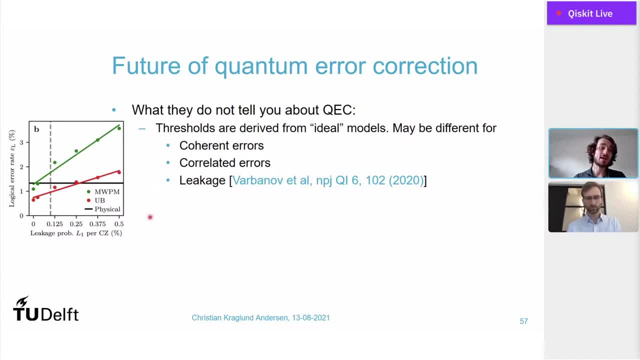 from the group of Barber and Tera. If you add leakage to your Z-Z gates, you could take a service code that would sort of, if there was zero leakage, be below the physical. But if you add leakage, even at 0.1% leakage, 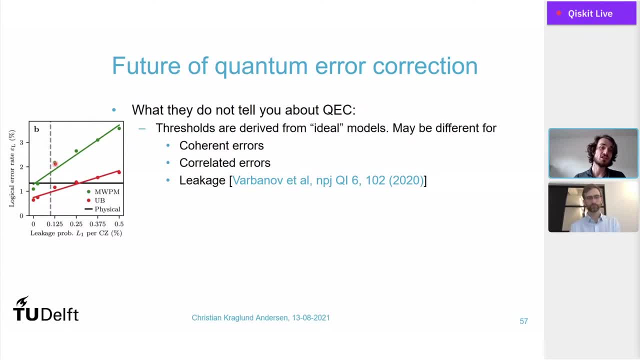 which is Z-Z gate. when you do the decoding, which is the green part here, suddenly you are not below the threshold anymore, Which makes things or makes life hard. The second thing that often gets forgotten is that if you actually want to go to this distance, 17,. 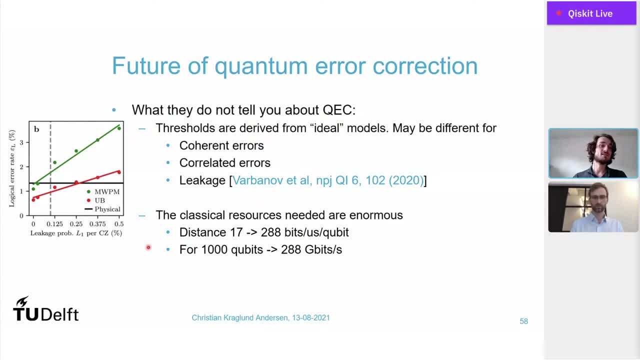 that I mentioned at the very beginning. you have an insane amount of data coming out of your device because you keep measuring these in semicubits. Every time you measure them you get one bit of information: The time for each- let's call it- each roundup. 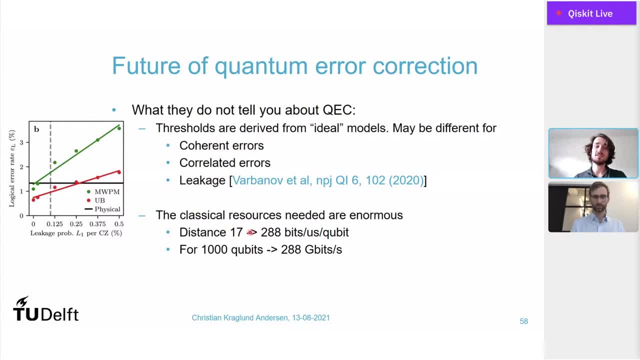 or cycle of error correction, is around one microsecond. So for distance 17,, you get 288 bits per second per logical qubit. So if you want 1,000 logical qubits, you get, yeah, close to 300 gigabytes of data. 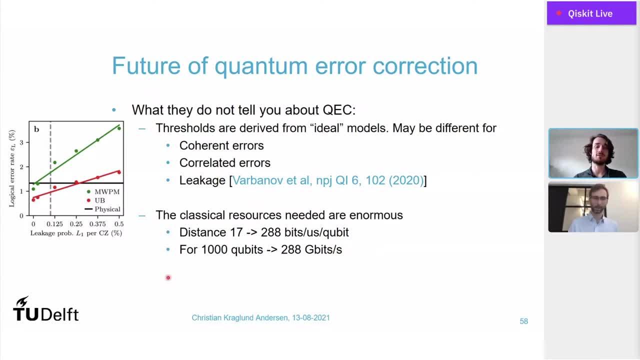 that you need to process in real time to decode your data. It's also so- that's just to tell you- that if somebody tells you or comes to you and say: hey, I will do quantum error correction at distance: 17 for 1,000 qubits. 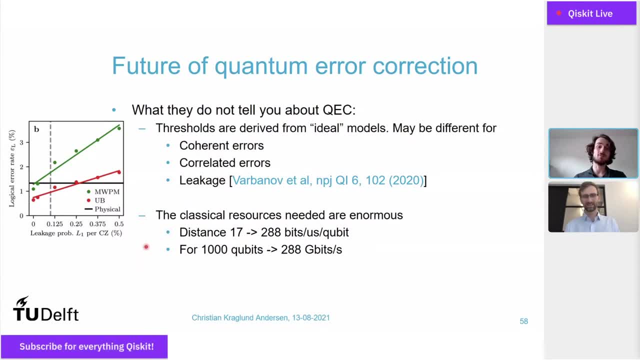 in five years. not only do they need to actually do 17 square times 1,000 physical qubits, they also need to solve all these problems in terms of like actually having a threshold that holds when you have coherent and correlated errors. 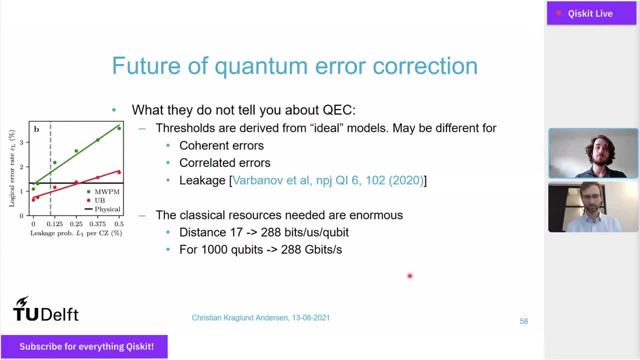 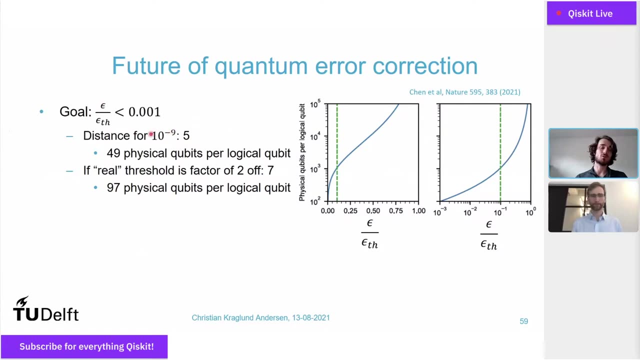 And they have to have found a way of really dealing with the data problem in terms of processing this data in real time. One way that I think would make life easier is maybe be a bit more ambitious in terms of the goal of the ground threshold before we start scaling. 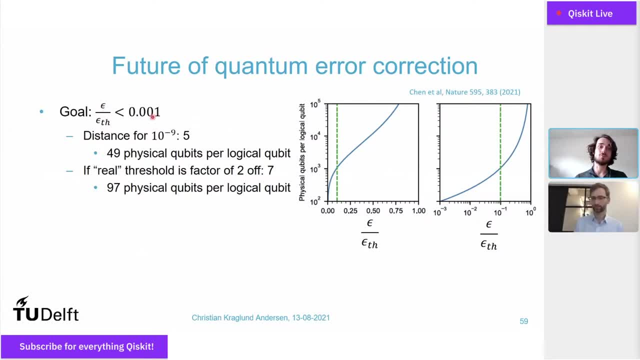 So if we go to, let's say, two orders of magnitude, we go better than the one I was mentioning before. Suddenly you only get distance five. if you want to go to 10, to the minus nine, You need 49 physical qubits. 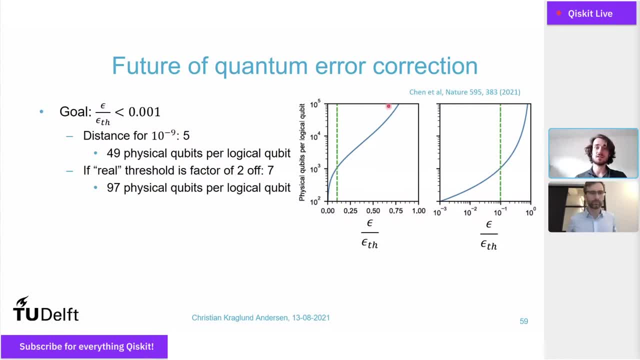 or logical qubits, And this is much more robust. So Google made this nice plot here with physical qubits that you need as a function of threshold. Here they were typing in 10 to the minus 12. So the numbers here is a little bit different. 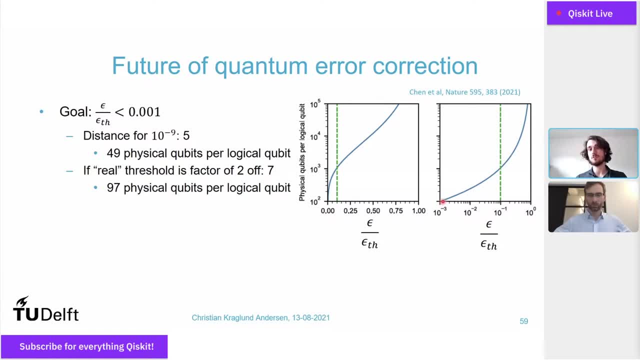 But what you see is that once you are far below threshold it looks a bit more flat than once you get sort of close to the threshold. So you don't want to be just below threshold because if there's some error, that just makes it a bit harder. 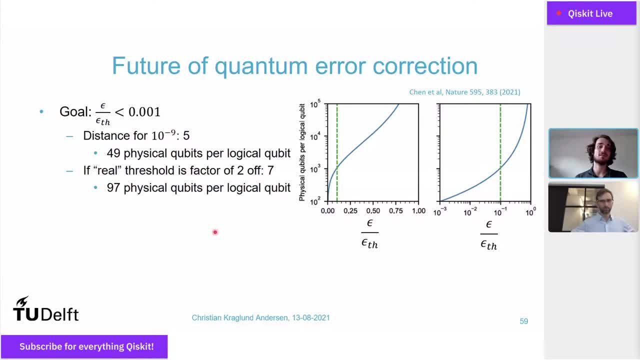 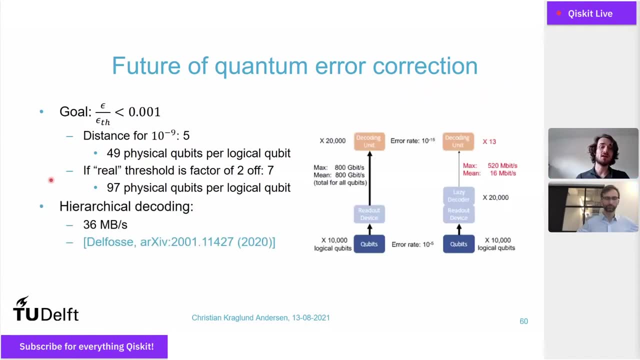 suddenly the overhead increases exponentially. So life is a bit easier if you're far below threshold And you can play tricks with decoding. that also limits this data rate. So there was this nice paper by Nicola de la Fosse that really showed that you can sort of have 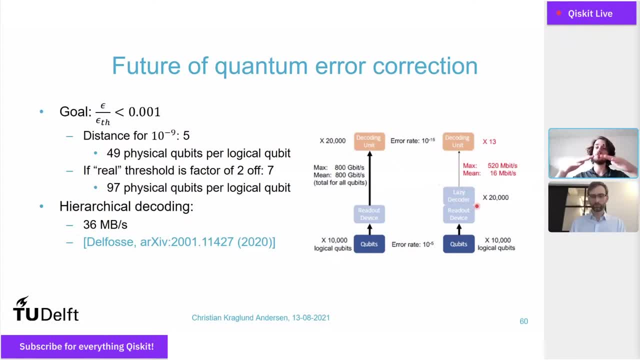 local laser decoders that lives close to the device. You don't need sort of global information. that do part of the job. And then you really have a very small data rate coming out of those And you can sort of reduce it to something maybe like 36 megabytes per second. 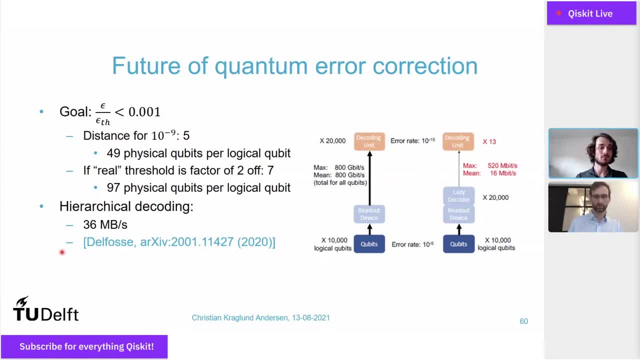 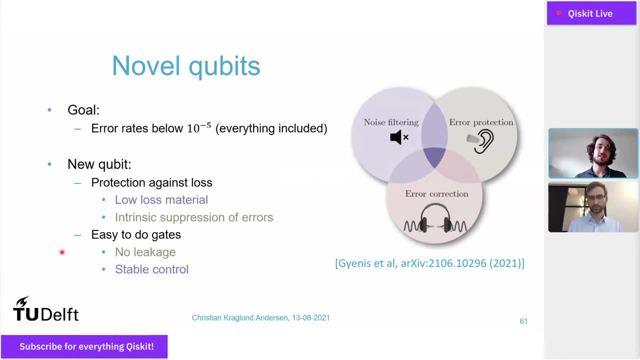 which is something to work with. So that's sort of the motivation I have for it. So starting my new lab is that. I really want to emphasize that. I hope we can at some point get to the level where our qubits are just much, much better. 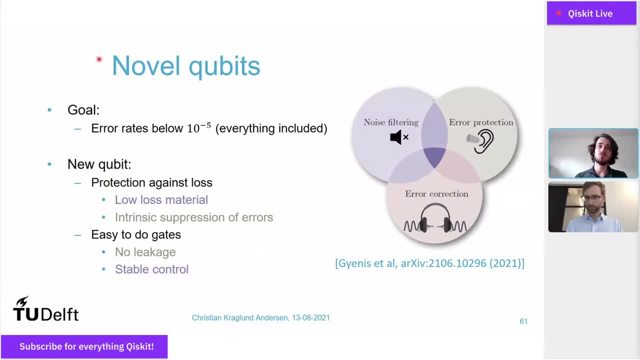 And one way of doing that is by making better qubits, in the sense that they are not only we not only filter them by noise, we are not only doing error correction, but we're also making sure that they are protected, sort of intrinsically whatever. 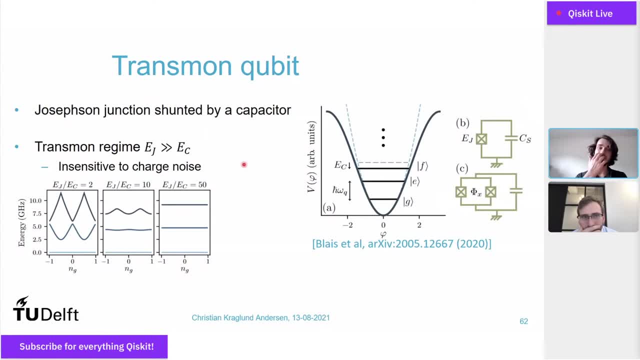 But that's something to enhance more, In the sense that if we just look at the simple transform, you have the Joseph junction, you have the capacitor. Here it becomes a little bit technical, but I want to still mention it so you can read about it later. 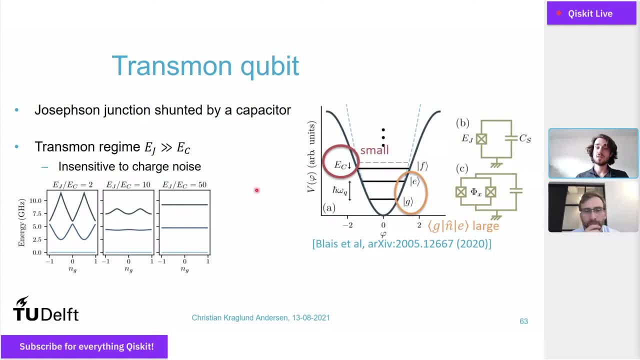 If you look at this simple transform, there's sort of two things that makes it a qubit. One is that you have this anharmonicity here, which is why you can address the zero-one transition GE here. But this is quite small in a transform. 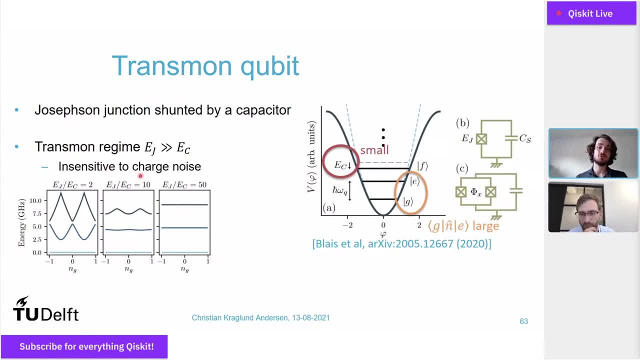 Which is good, because that gives you insensitivity to charge noise, But it also means that it's very prone to leakage, which I mentioned was one of these error sources. that makes it hard. And the second thing is that if you look at the charge matrix element, 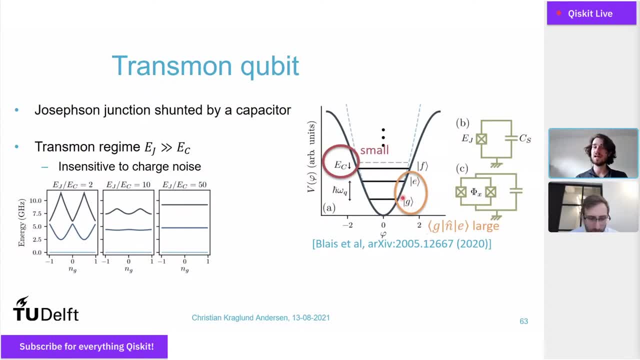 between the ground state and the excited state. this is sort of as large as it gets in sort of a unit as well, Meaning that the only way you can really get better coherence times for a transform is by making your materials out of. There's alternatives in literature. 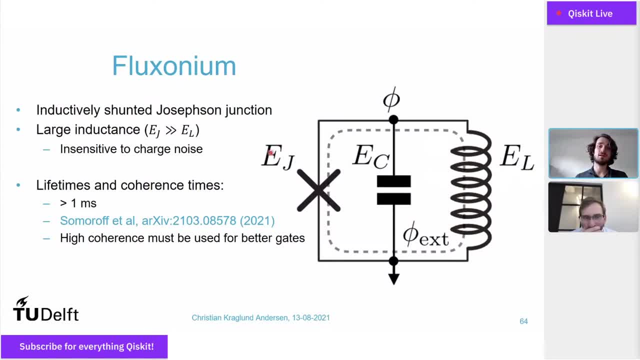 and I just want to flash this as an outlook And I think this is really cool- The results that was recently done in the group of in Ireland, where they took a fluxonium qubit, where you, instead of just having a shunt capacitor, 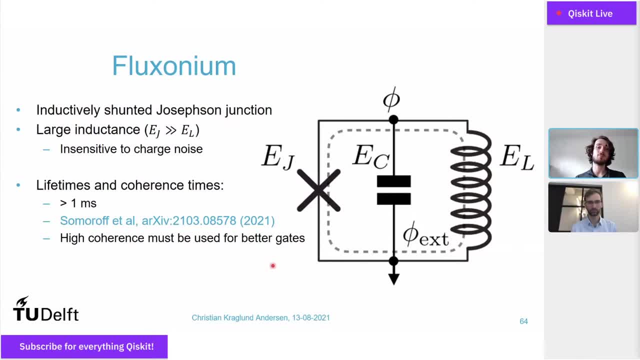 you also put a shunt inductor. By picking the parameters correctly, they could show coherence times above one millisecond And they had single qubit errors of 0.9999.. So four nines above four nines, which is getting close to this goal. 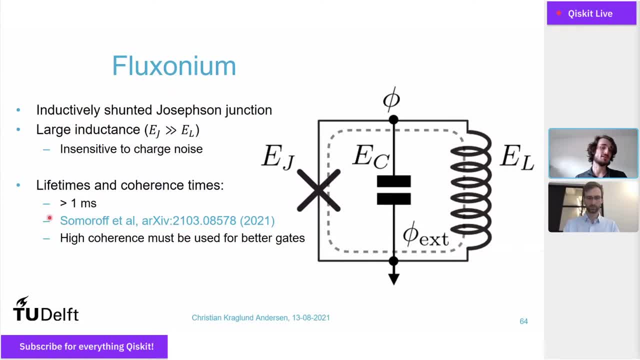 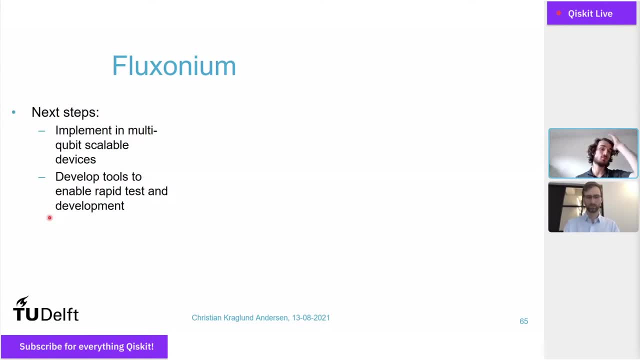 that I just had above on. So this is really exciting stuff. But what is sort of missing is that this type of qubit needs to be implemented in a scalable device, And for that there's really sort of a broad range of tools that still needs to be developed. 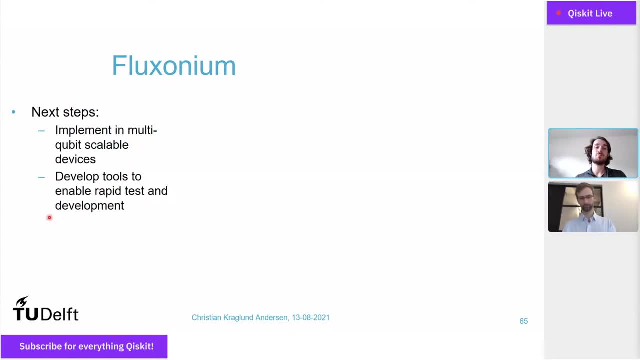 Here tools goes everything from we need to have more readily available design tools. We need to have multivariate electronics that really matches this. We need to have calibration tools that matches fluxoniums, For example, if you go to companies like Zurich Instruments or Q-Blocks. 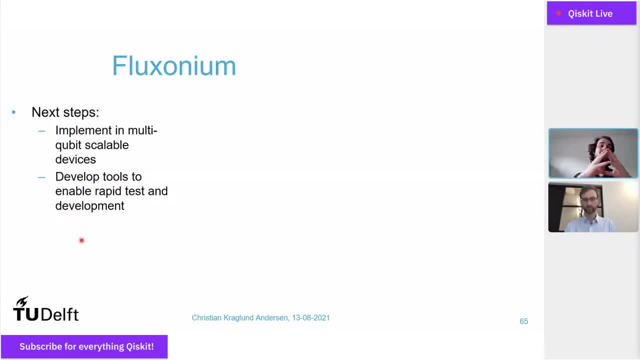 you can really buy electronics that are highly tailored to transform qubits. That doesn't exist for fluxoniums, Yes. Or if you go to Qiskit Metal, which is developed by you, have tools that just allows you readily to transform qubits. 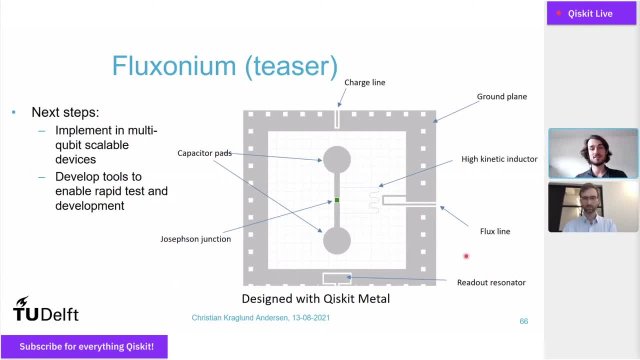 In our group we have recently made an effort to implement also fluxonium qubits using this tool, And I hope we can later make a commit with some of this such that we can really get the community involved in also designing the next generation of devices that not only uses transform qubits. 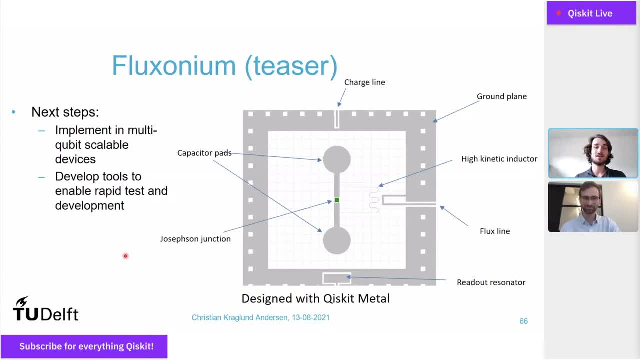 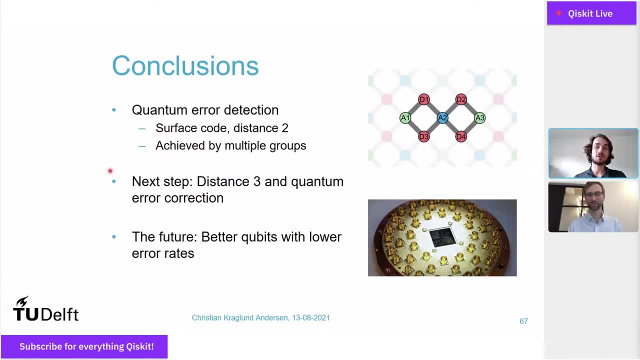 And we can get to our 10, to the minus five. So with that, thank you all for your attention. To summarize, we looked at quantum error detection with a surface code distance two And we really showed that we can achieve logical lifelines better than the best physical device. 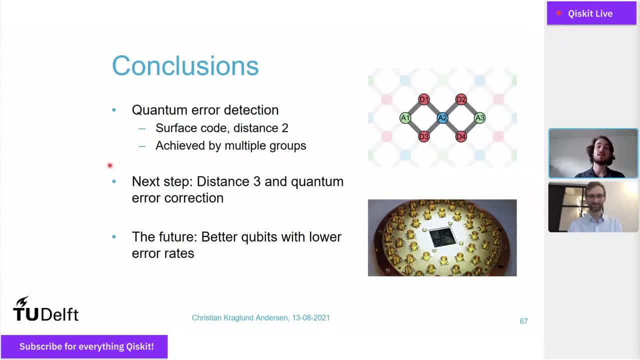 It's been achieved now by multiple group, by the group at ETH, by Diop DiCarlo and Delft by Google. So it really shows you that the surface code actually works, And the next step for everybody now is we need to go to distance three. 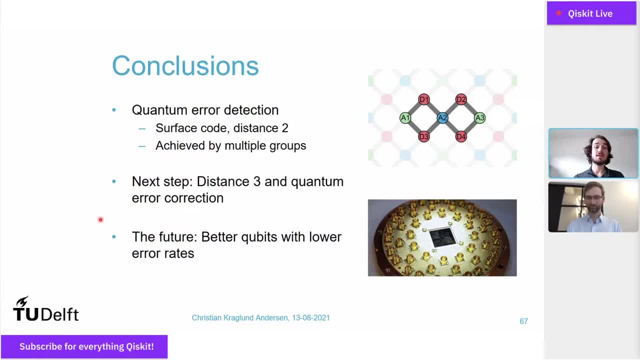 and show that we can also correct that And then in the future to make really really big, large scale quantum computing with error correction. I think it will be really important to focus on getting better qubits with lower error rates so that you can really be far below this error rate. 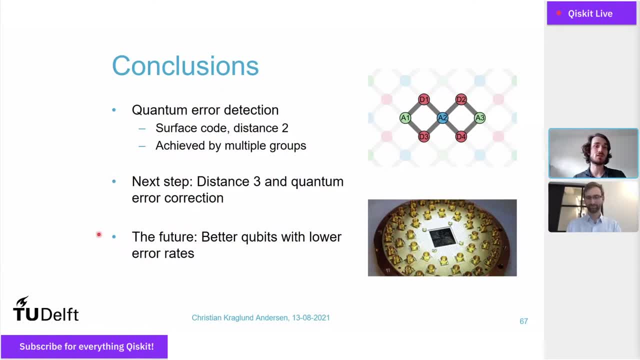 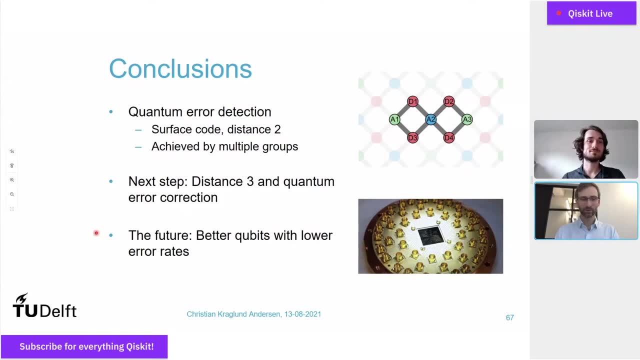 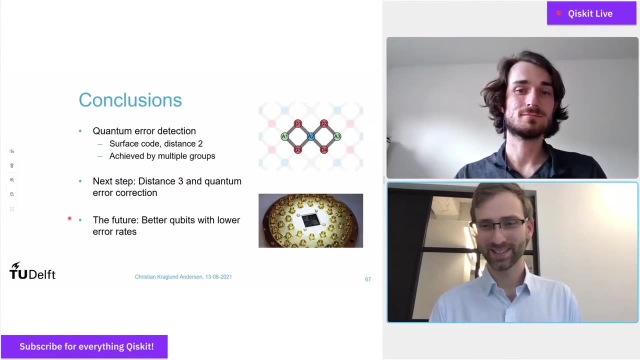 Thank you all for your attention, Looking forward to seeing if there's more questions. Thank you, Christian, for the absolutely wonderful talk and results. Congratulations again. Also thrilled to hear that Qiskit Metal has been of help to you, And that is a really neat looking fluxon. 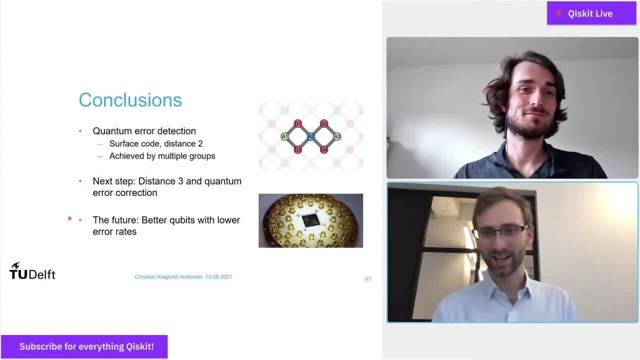 I've never seen one quite designed like that, So I'd love to hear more about that later. There are a number of questions, So where should we begin? I'll begin in order from the talk. Could you comment on the non-QNDness of the measurement? 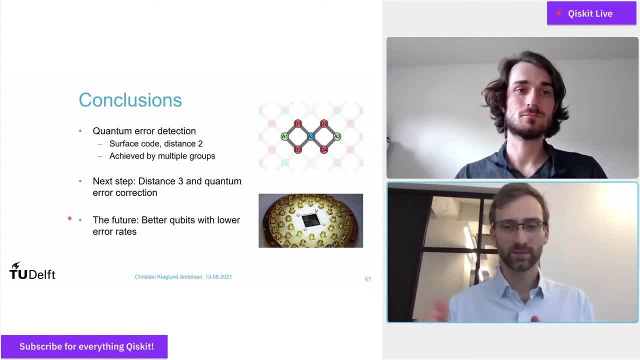 and could we measure that as well as we looked at the defeat? Let's start there actually. Yeah, Yes, So you could look at it. I think for this device we actually did not quantify that Everyone, So I cannot give you a number for that. 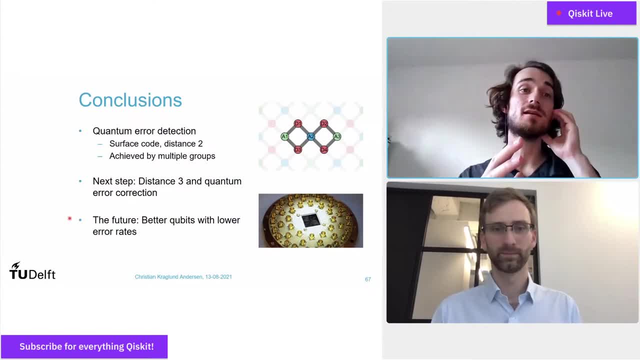 but generally for our previous devices when we looked at it, it was typically very good compared to the fidelity, So it was on the same level. What was the measure? So the fidelity was typically okay, even for repeated measurements limited by T1. 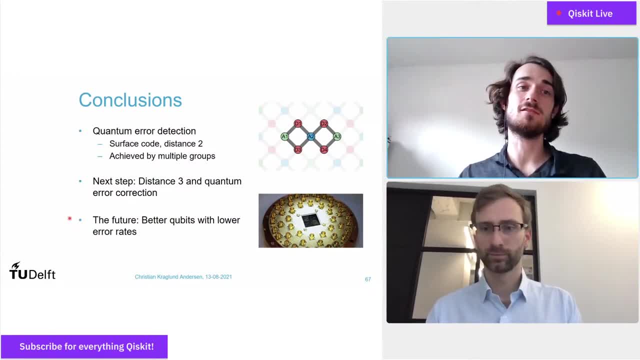 on previous devices And I assume that would be the case here also. So I assume it adds very little non-QNDness. Yeah, I see. Oh, and folks, please post questions in the chat box and we'll get to them as we go through this. 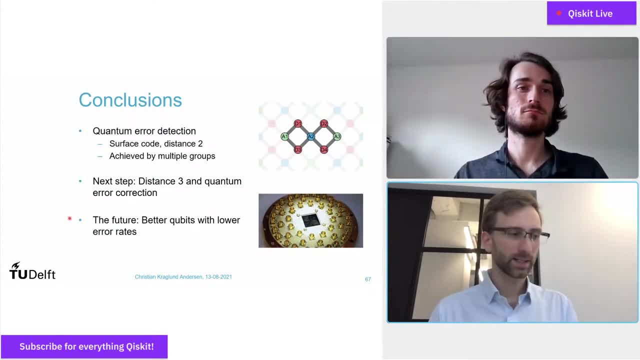 I'll pick them up from there. And you commented a little bit about this leakage out of the Hilbert space. You know the ZZ crosstalk is really big. What about gate crosstalk? Yes, this can be very important also. 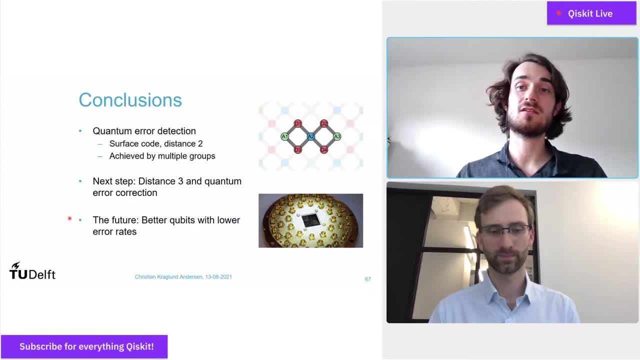 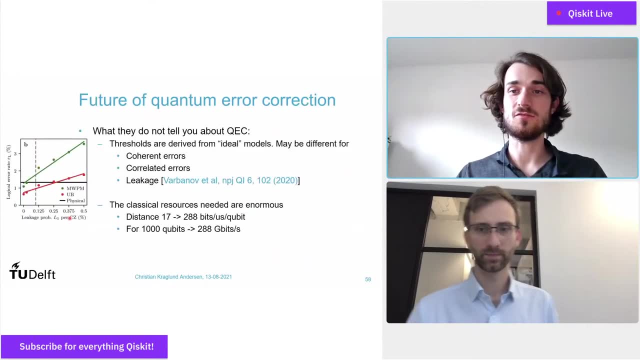 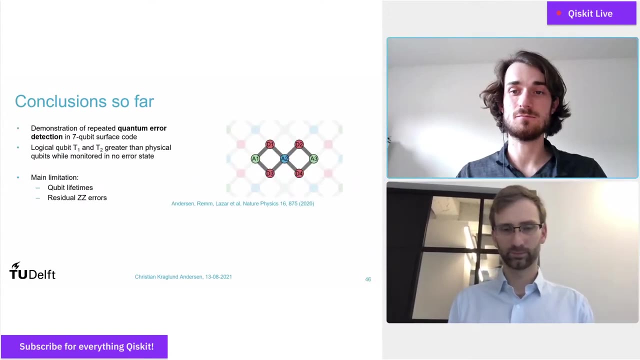 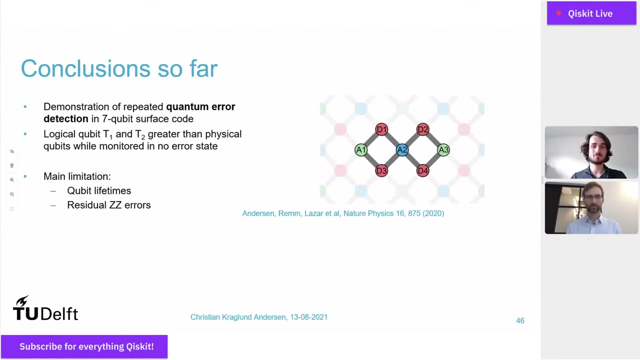 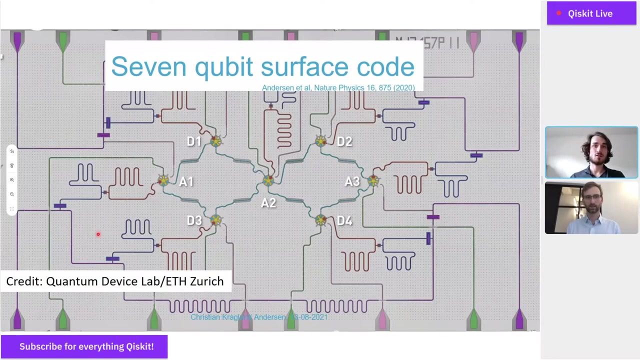 For this. it was not a very big concern in this experiment, for a few reasons. One is that we have a lot of, So one thing that you will see is that we have, So one thing you see is that we have, Okay. Okay, can you hear me now? 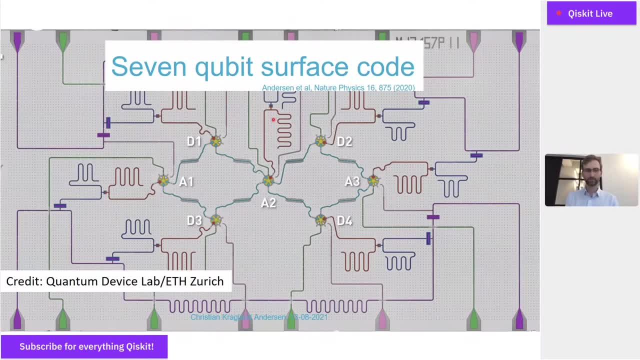 Yeah, Okay. So what I wanted to say is that what you see is that qubits have individual drive lines here in the purple. That already helps minimize the crosstalk We also have. it's maybe a bit hard to see, but if the resolution is high enough, 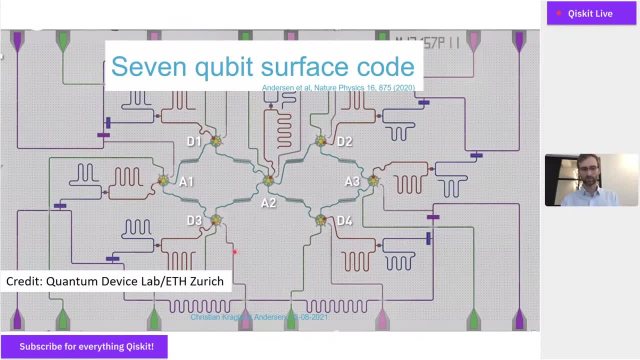 you can see that there's these white lines crossing. Yeah, These are sort of air bridges that go over, which makes sure that the ground plane is really well-defined around the chance line, which also helps suppress some of this crosstalk, which also helps suppress some of this crosstalk. 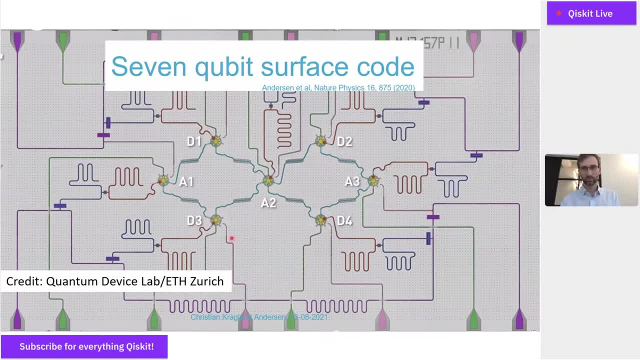 And finally, all the qubits sit at very different frequencies, meaning that even if there was some crosstalk, the crosstalk would be at a different frequency, So they're also suppressed by that. So could you give us the range of frequencies? 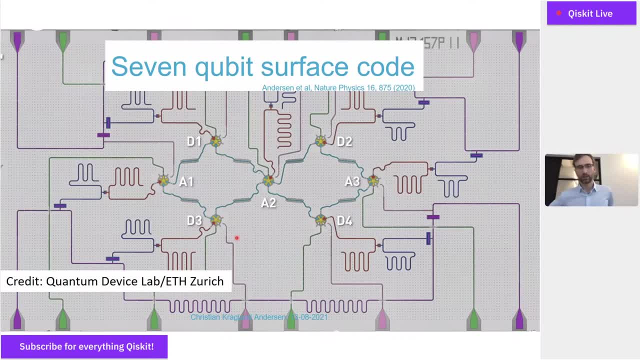 just so we have a more concrete picture. Yes, So the top ones here sit at around six gigahertz. Then we have the middle qubits. They all sit at around 500 megahertz below, so that's around 5.5 gigahertz. 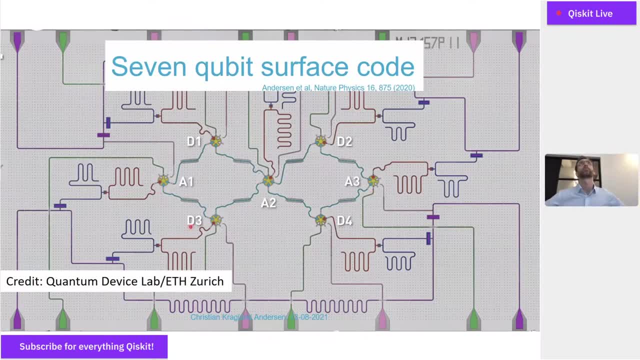 And then at the bottom here we have four point. it should be around five but it's a bit lower. so like 4.8 gigahertz, And maybe you said this already and I forget, but are the two qubit gates flux-driven? 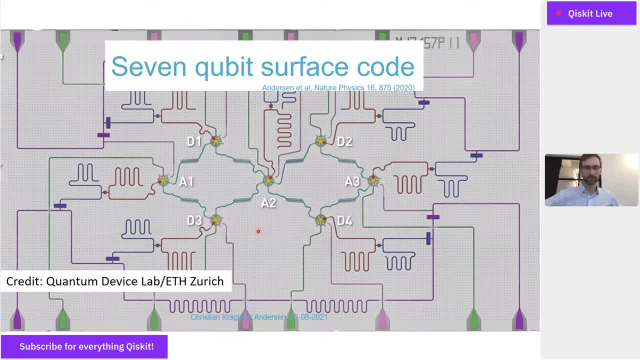 through the qubits, or are they-? Yeah, exactly, So it's flux-driven. So what we do is we take, we use the flux line to take the frequency of one qubit and put it close in frequency to the other qubits. 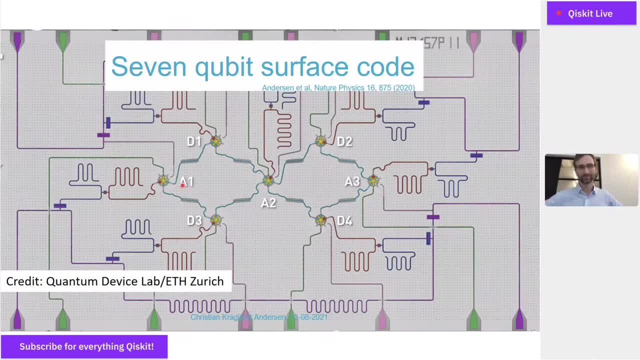 To be more precise, closing frequency to the other qubits minus the end harmonicity, because we go through the two state and back to the computational subspace, will pick up a phase only for the one-one state, which is the C-set state. Mm-hmm. 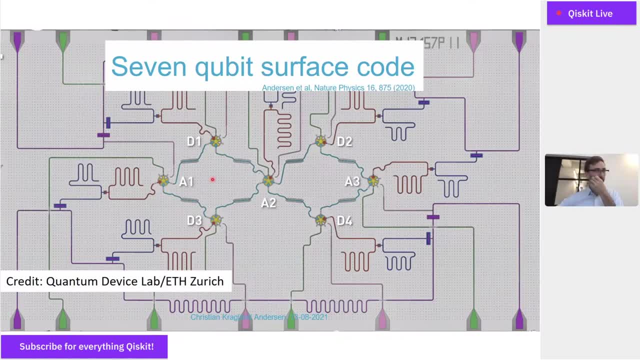 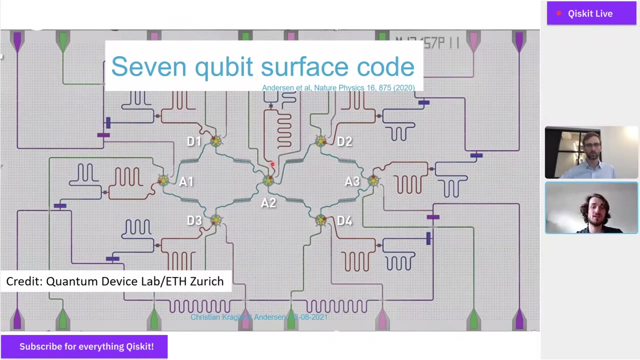 Awesome, Great, Great. And the readout. what about kis and kappas? What order of magnitude are those Readout? kis are from a few, maybe one, one and a half megahertz for some of the data qubits. 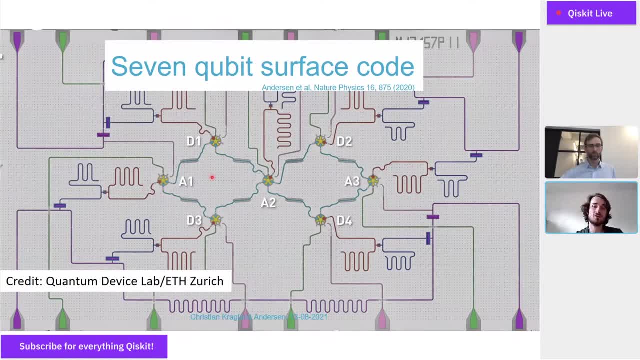 to up to 40 megahertz for the largest ones And kappa for the readout resonator and the effects of kappa is up to 10 megahertz. Hmm, That's pretty big Right, Right, I think the kappa. 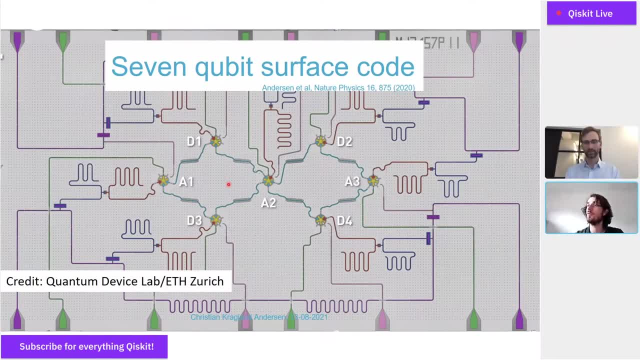 that's something that I think is often overlooked a bit in terms of getting fast readout. It's really important that kappa is big because you need to put in those photons. That's right. And question from the audience. Could you talk, explain, if possible, about? 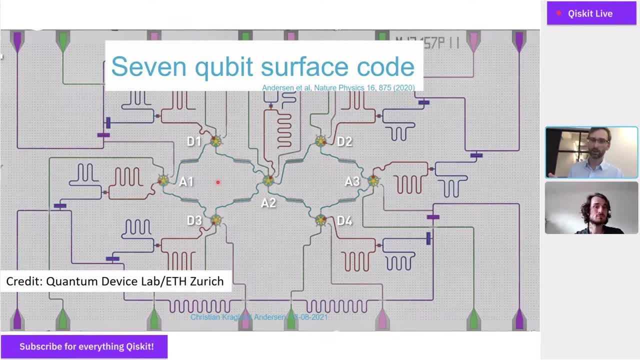 sorry, actually I missed another one. Does the experiment also include error mitigation schemes And if not, could that help? Currently there is no error mitigation beyond this error detection. Here we really wanted to just demonstrate the logical T1. But what I can imagine is: 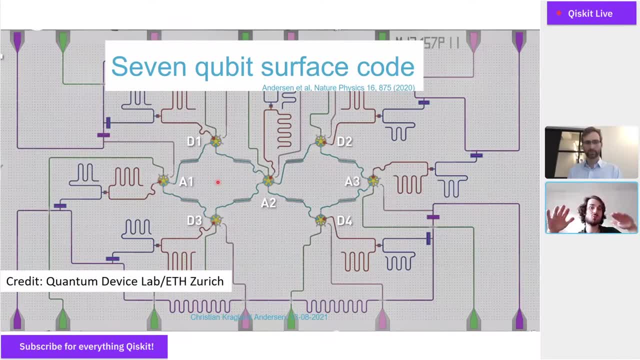 that if you would have, let's say, a small device with multiple error correction or error-corrected qubits, maybe even error-detected qubits, having sort of an additional layer of error mitigation on top that is tailored to your quantum algorithm. 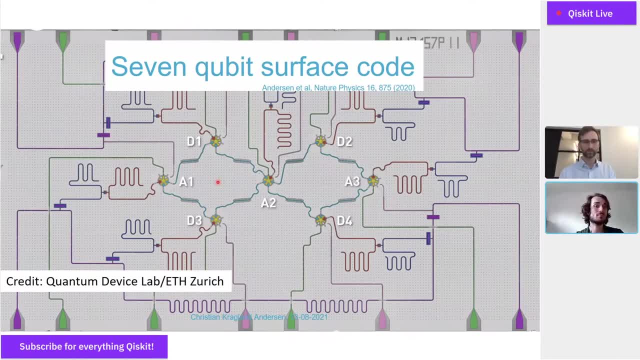 I think that this was not Say that, say the last part again. sorry That we did not do in this experiment. Got it, got it great. And question from deep from the audience: Can you talk, explain if possible, about quantum LDPC codes? 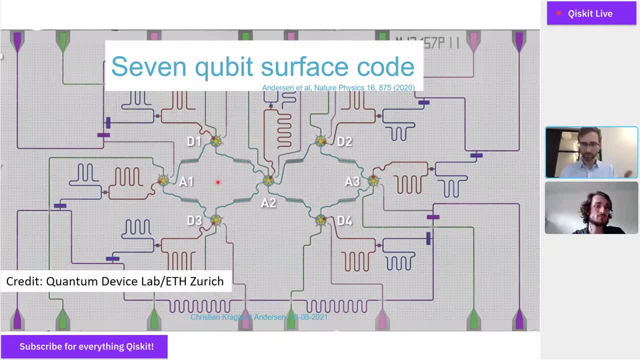 and its future in realization, slash how it performs, or you know, against the surface code. I guess it's a question about surface code versus other codes. Yes, So these quantum LDPC codes are very, very, I think, very interesting from a theoretical point of view. 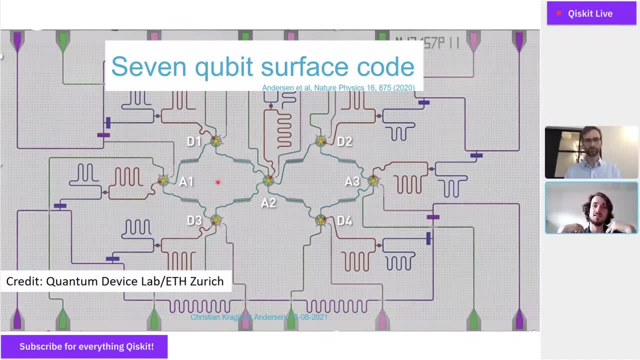 But I think what is really missing for me as an experimentalist, when I see these papers- and they have very nice thresholds when you look at them and they have nice results in terms of if you have many qubits, you can really compress the information much better. 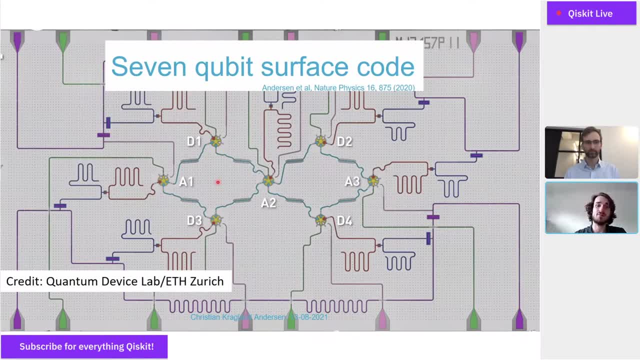 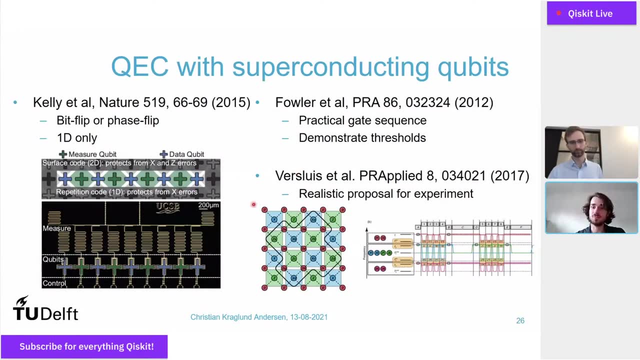 which is really nice, But what you really need if you want to make it a device, is a really concrete gate scheme. So you need to essentially look at a paper like this one. We can start with the one by, and then you would need to write a paper. 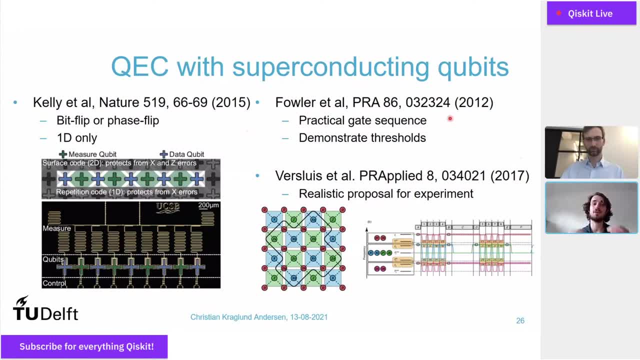 like this, but for the LDPC code You can really say that: okay, look, this is the concrete gate scheme that we need to run to demonstrate this threshold on a real device. I think this is still. I would be excited to see it. 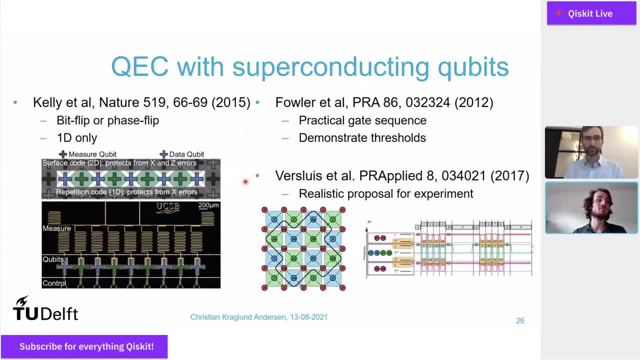 but from my point of view I have not seen it yet for these LDPC codes. Hmm, Wonderful And I know I guess it's very preliminary work, but could you comment on why you have little circles for the fluxonium on the ends? 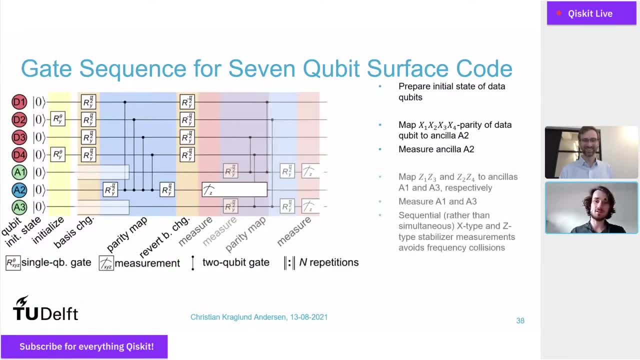 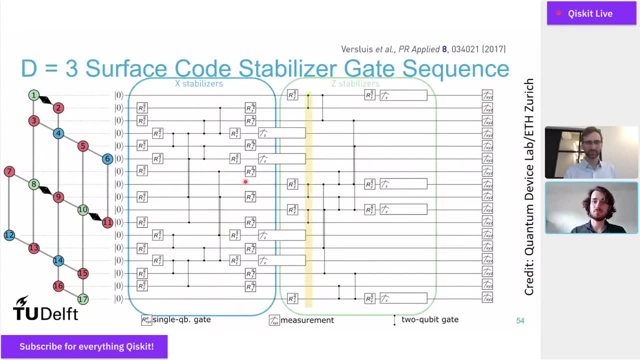 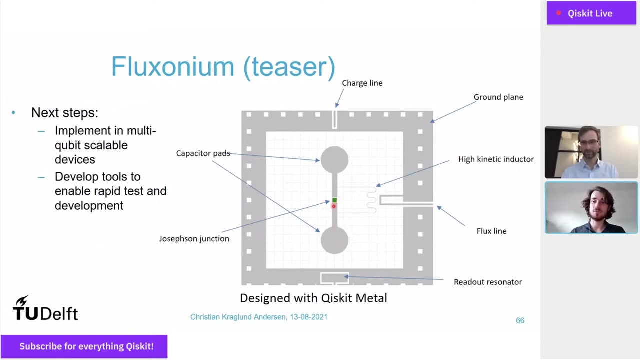 Yes. So what you need is: you want a finite capacitance. The circles are a good way of controlling that. So the idea would be that you want this sort of capacitance. You don't want it to be too close here because it wants to be far away. 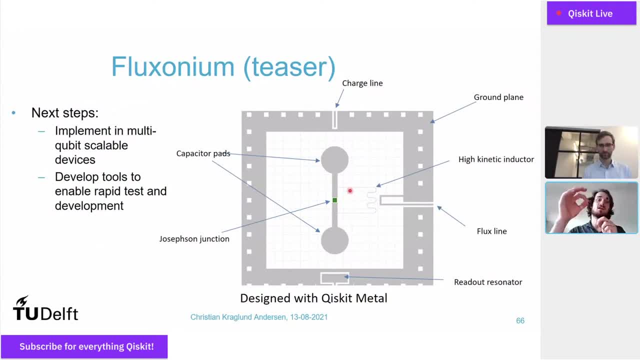 from the kinetic inductance to really have the capacitance sort of orthogonal to the inductance that you put. And then it needs to also have sort of a finite area such that you have strong enough coupling to the readout and to the charge line. 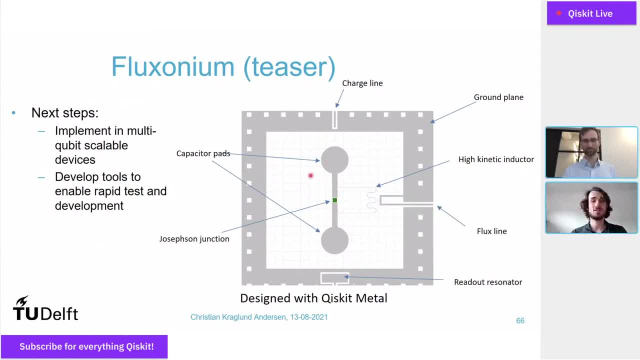 So you can put it sort of somewhat far away. Awesome, That's really nice. That's really nice. Excuse me, I'm just taking my breath back. you know, seeing this design with Qiskit now was really neat. Shout out to my master's student. 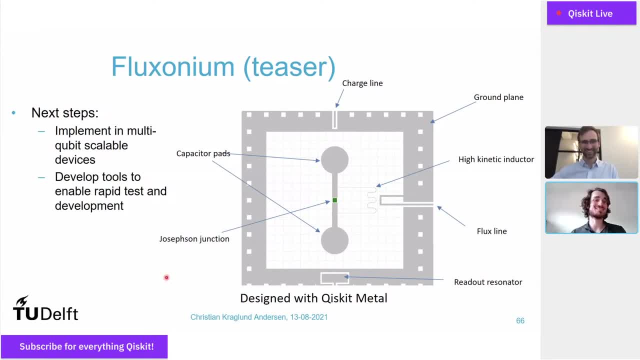 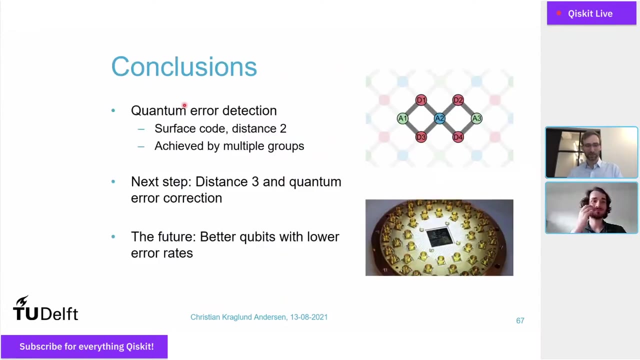 Rukhwal who managed to present this. Yeah, And we more than invite and welcome contributions. That's what makes open source thrive and work, And you guys should get a gold star and more for pushing the beta version. So, Christian, I think seeing